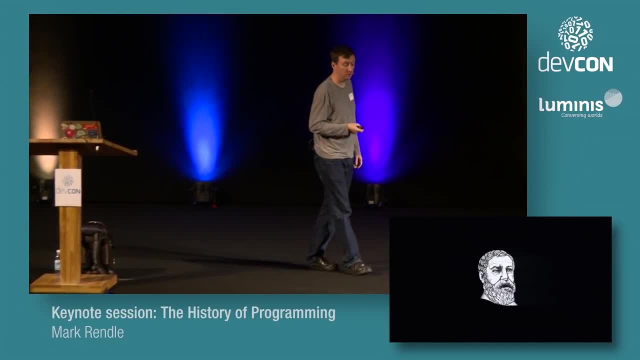 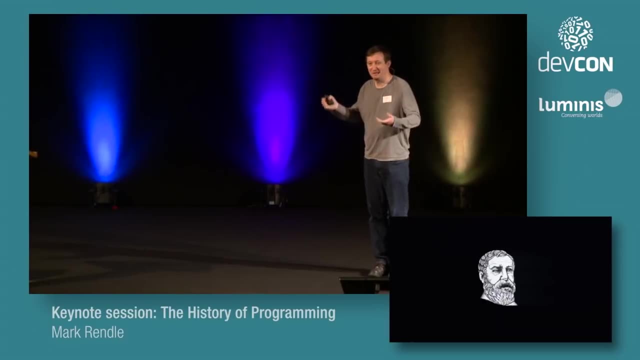 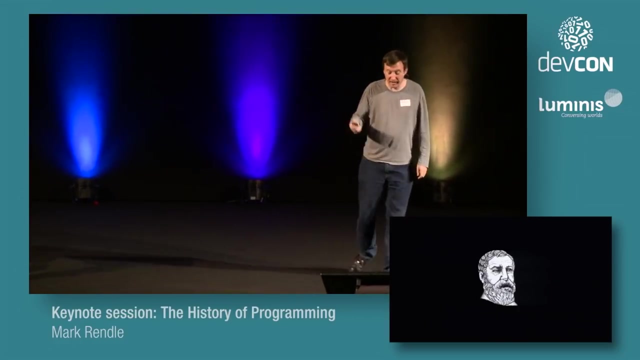 programmable thing that we know of. obviously there's that greek woman with the laptop as well, but has that been in your papers? over here there's like some greek relief thing and this woman is quite clearly got a laptop and it's got usb ports and everything. but yes, but no, and 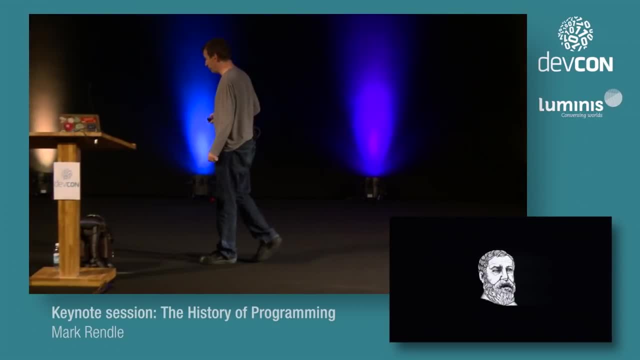 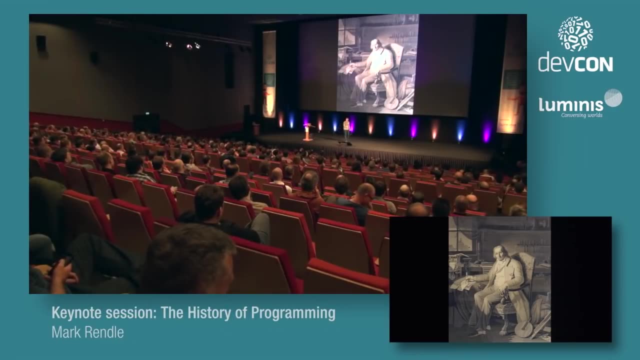 then there was very little progress in in the world of programming for the next 1800 years. and then this chap came along, and anyone know who this is. this is jacquard, jean-marie jacquard, and he created the jacquard loom. 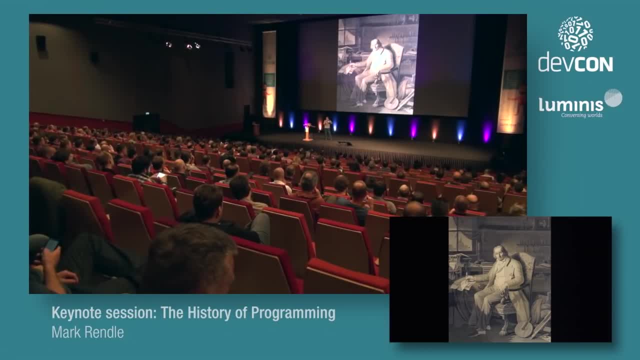 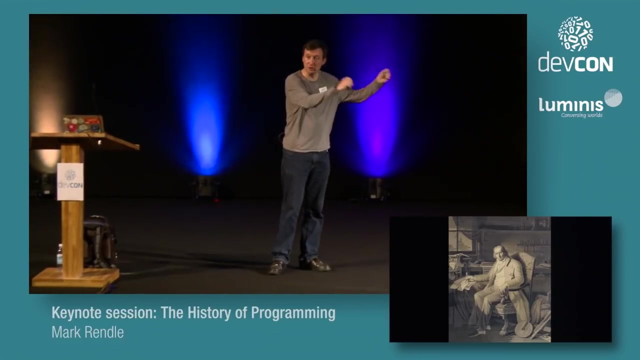 and the jacquard loom created patterns on rugs and carpets and things, but it used punch cards- actually the same kind of punch cards and the same principle as the punch cards that were used to to program computers. they were made of metal and you put them in the loom and it read the punch. 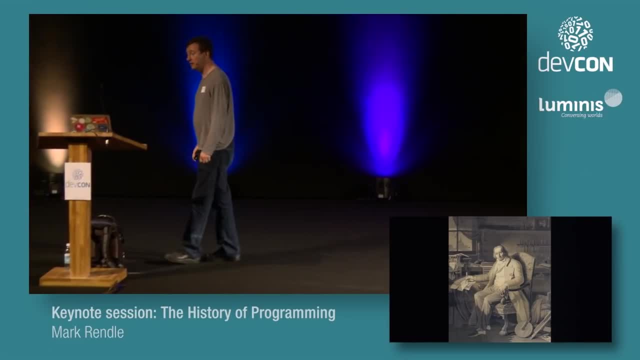 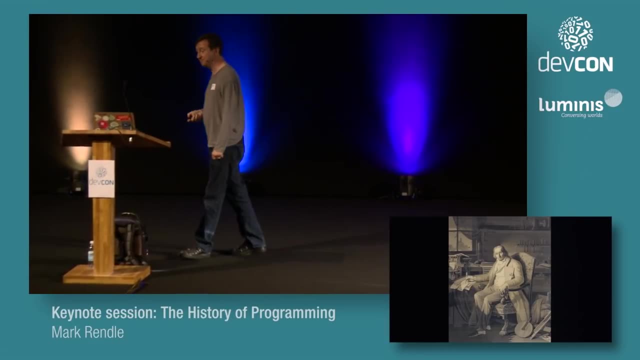 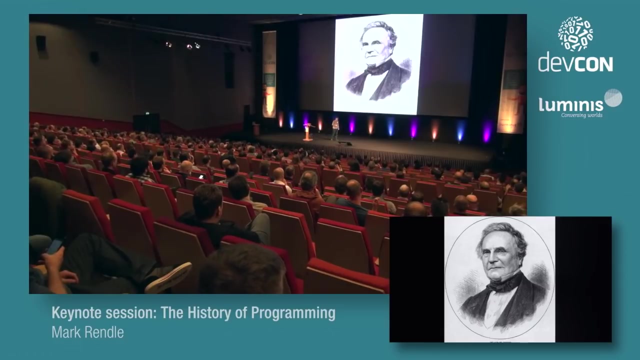 cards and then wove different patterns into the rug, and so that was kind of programming. people created the punch cards, they were sort of loom programmers. and then, uh, this chap came along, uh, towards the end of the 19th century, who's this babbage? that is charles babbage, and 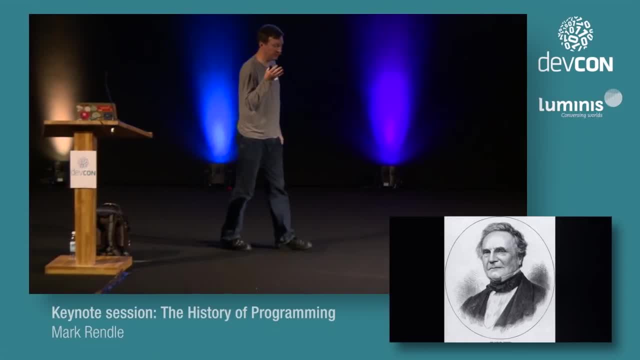 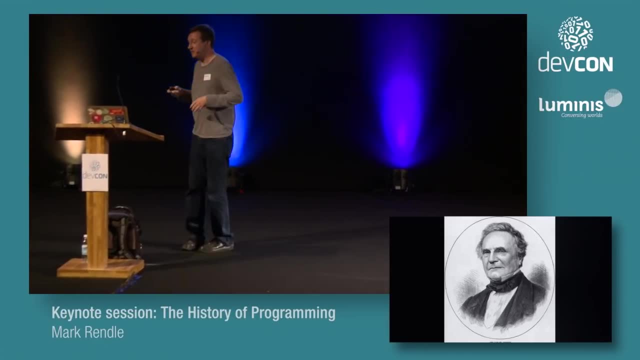 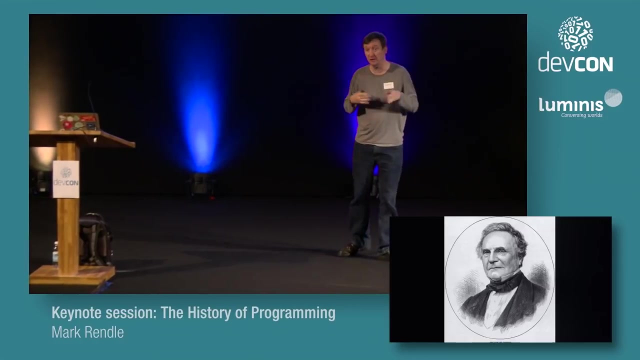 um, charles babbage uh, created this design. he had this, this dream, um, probably as a result of taking, but he had this dream of a, of a machine that could perform calculations, and, and he designed this machine and he called it the calculating engine. um, and, and he went to the uk parliament and said: 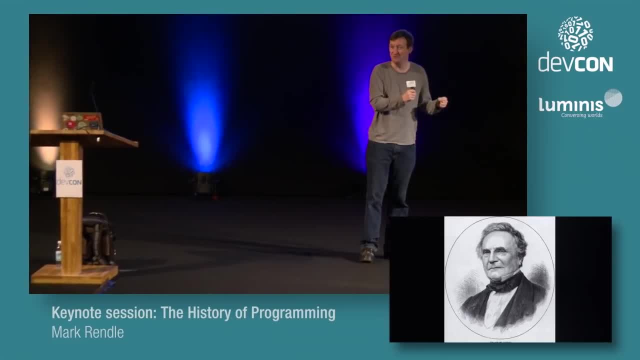 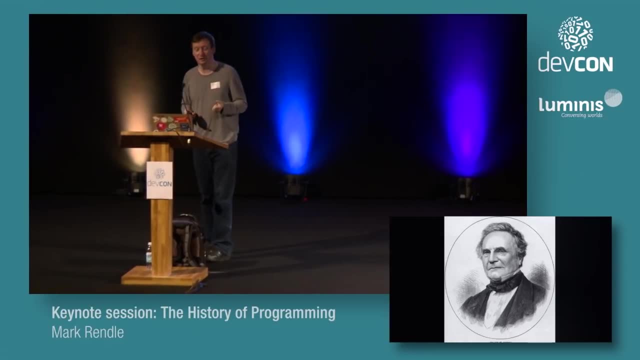 i need a million pounds, which in those days was a lot of money. i need a million pounds to build my calculating engine. and i love, i love charles babbage. um, he, he was ahead of his time in so many ways because he was a man of his word and he was a man of his word and he was a man of his word. 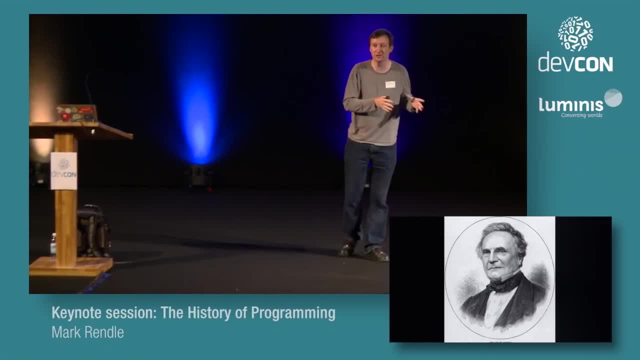 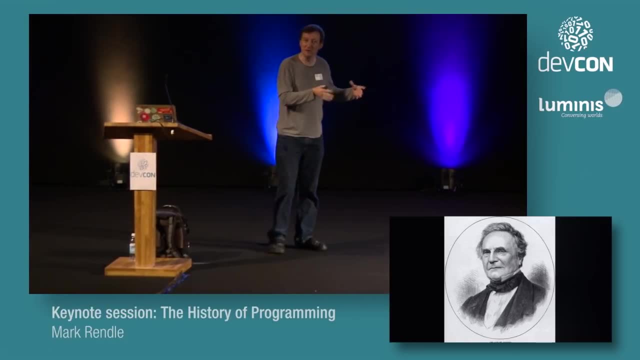 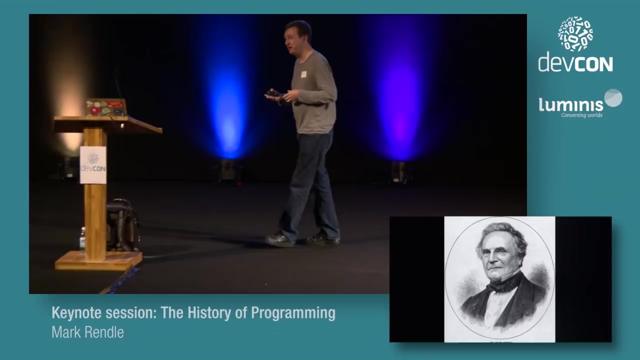 and he was the first person in the computer business to do something that i'm sure everyone will recognize as very familiar. parliament gave him the million pounds and he went off and he started building the calculating engine and he was about halfway through building it when he had 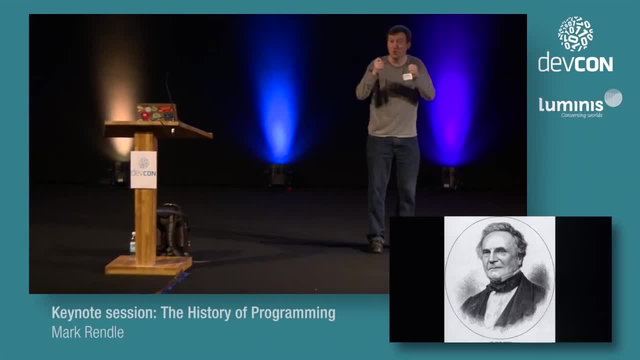 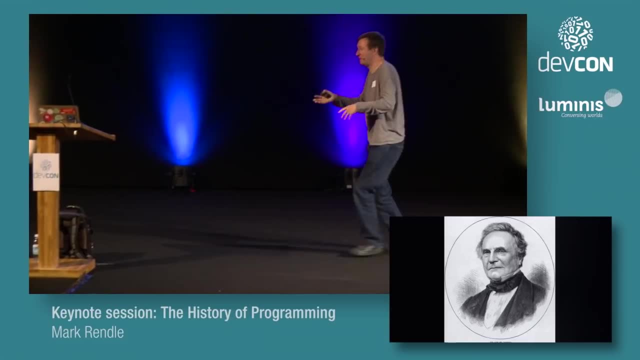 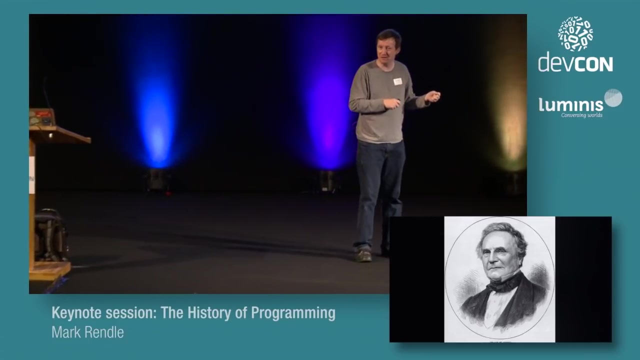 an idea for something better. and he said: oh no, oh, oh, that would be so much better. no, let's do that instead. and so, with the thing half built, he went back to parliament and said: i need two million pounds. give me two million pounds to build the analytical engine. and parliament said no finish. 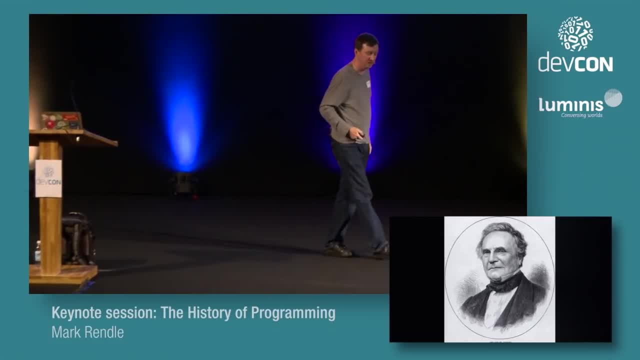 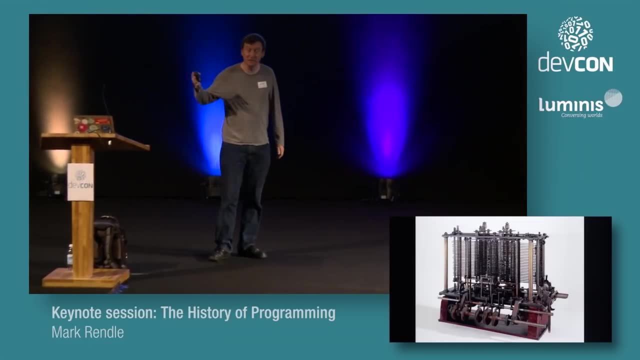 the thing that you said. no, i'm not doing that, i under the analytical engine. and so he never finished the calculating engine and they never gave him the money to build the analytical engine. if they had, this is what it would have looked like. this is a modern. uh, they built it at the 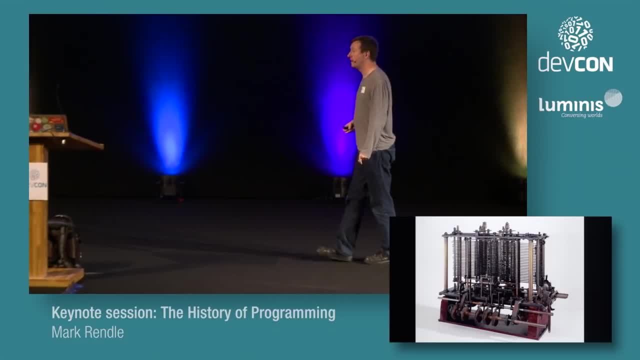 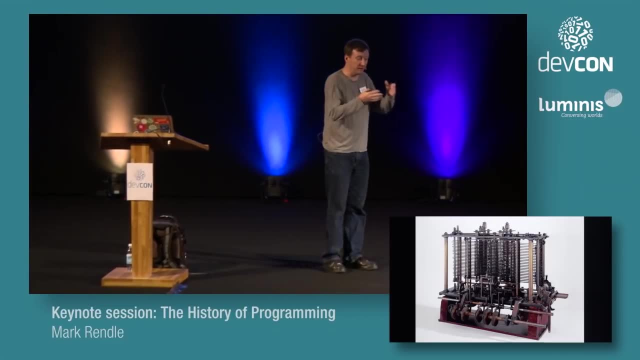 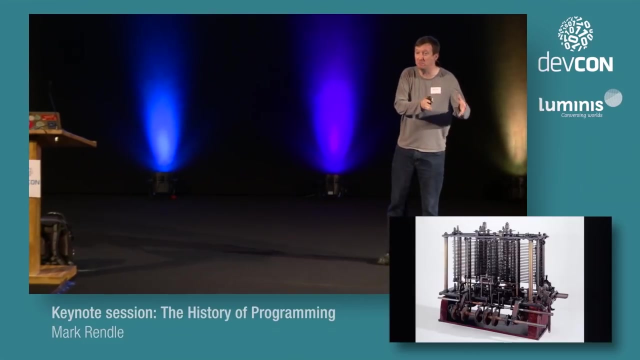 science museum in in london, and that's what it looked like, um, and that's what he designed, and it basically works. the thing that's really interesting, though, is that, obviously, the hardware never got built, and and it's questionable whether they had the tools that would have been necessary to build that. 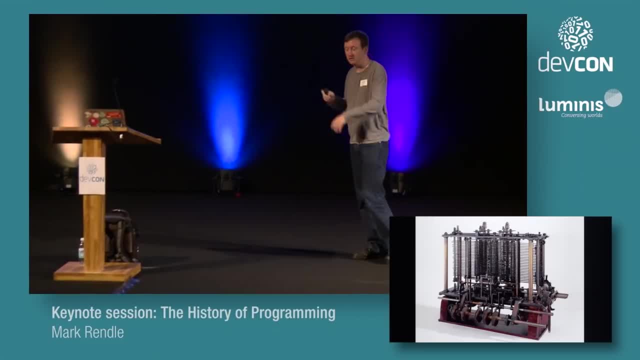 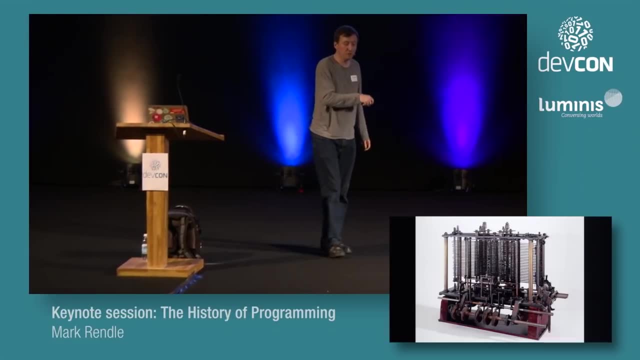 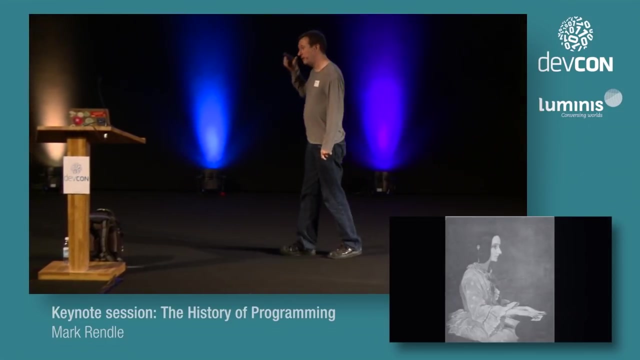 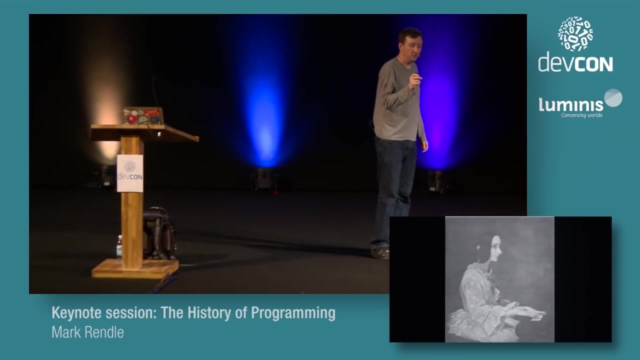 hardware, um, at the start of the end of the 19th century anyway. but the fact that it couldn't be built didn't mean you couldn't write software for it. and so somebody did write software for it, this woman, ada lovelace, the world's first computer programmer, and she was translating a book. so a chap wrote a book. 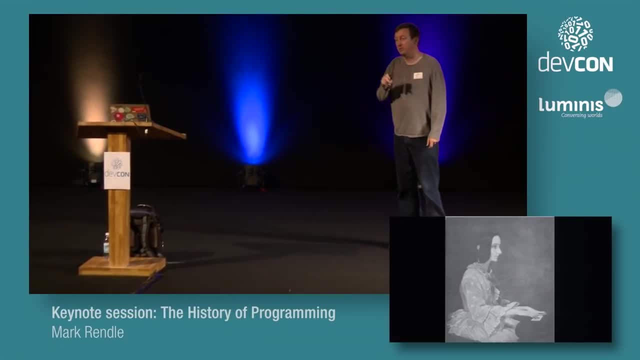 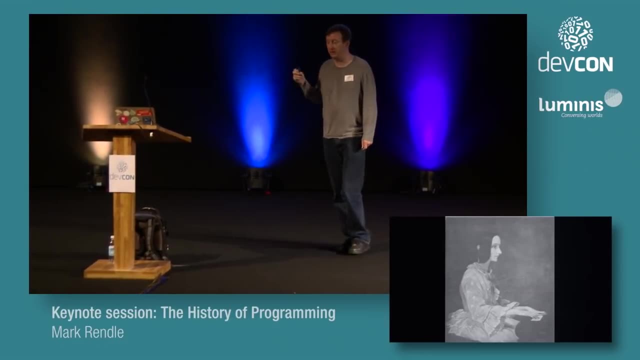 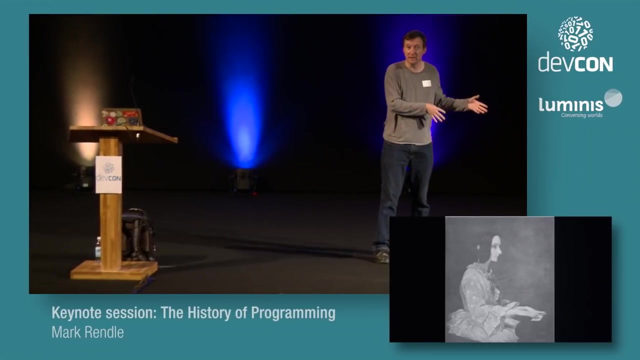 about the analytical engine, which didn't exist, uh, but the chap who wrote it was italian, and ada lovelace translated the book from italian into english, so you know quite good with languages, and as she was translating it, she learned all about how it worked, and so she worked out how. 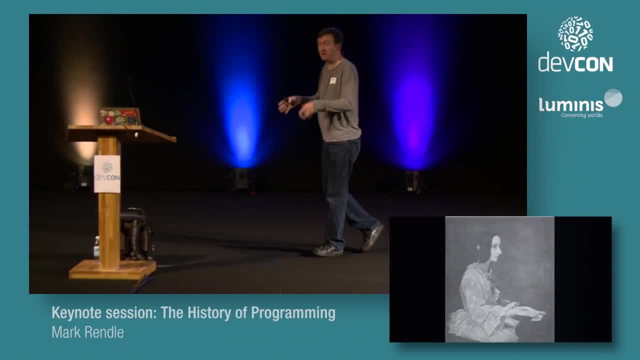 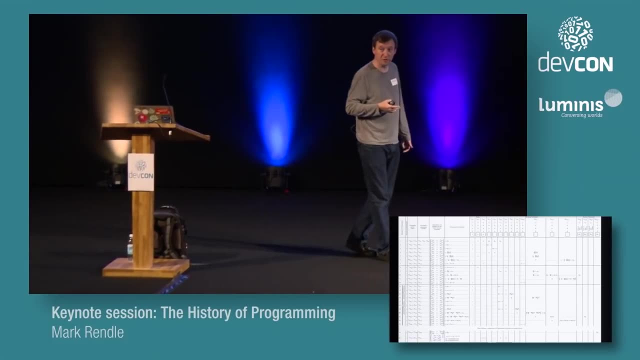 to program it. and she said: well then, this theoretical engine is going to be used to build the analytical engine and theoretically would be a program that would work. and this is her kind of sketching out of this computer program that would have run on the analytical engine. and when they built it they did. 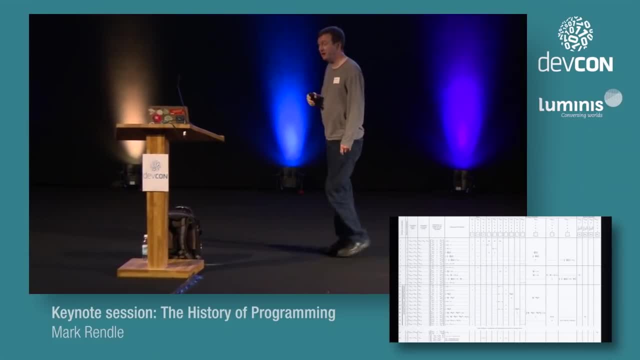 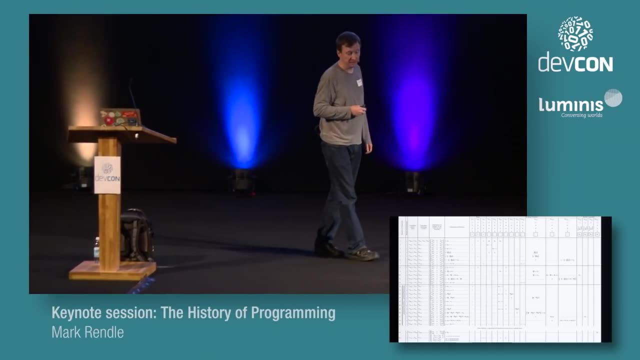 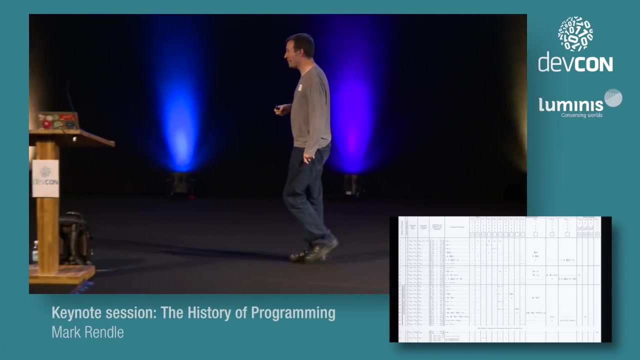 it and it did work, and it did what she thought it was going to do, which i just think is spectacular. also, she was the daughter of byron the laudanum addicted, syphilis infected poet. so, yes, not not great parents, not the best start in life. so that was babbage and that was all very exciting, and then really, 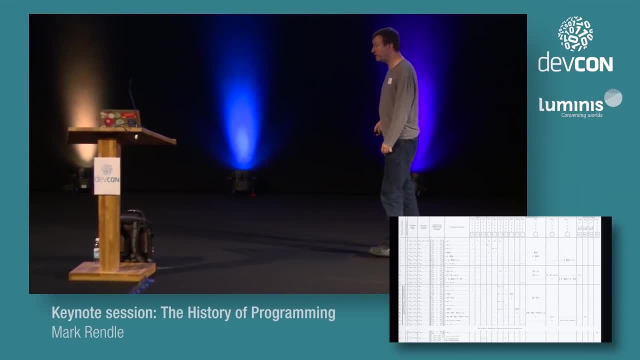 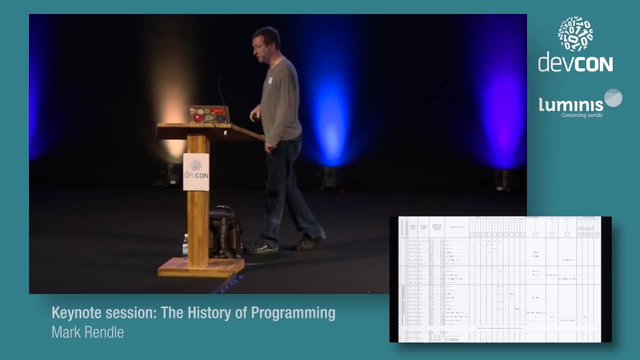 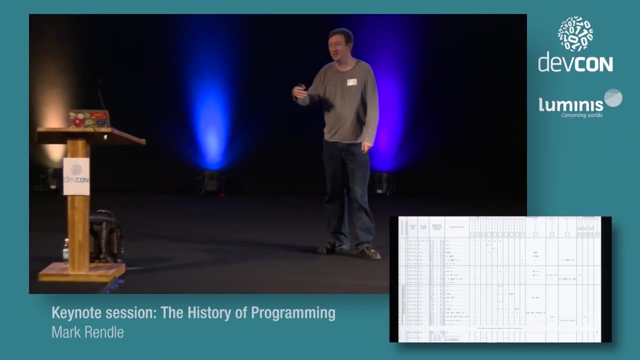 it kind of went quiet again, uh, until the middle of the 20th century. um, and there was, there was a bit of a, a scuffle, um, in the middle of the 20th century some people disagreed over a few things, um, and, and the germans obviously were using the enigma, uh, encrypting machines, and they thought: 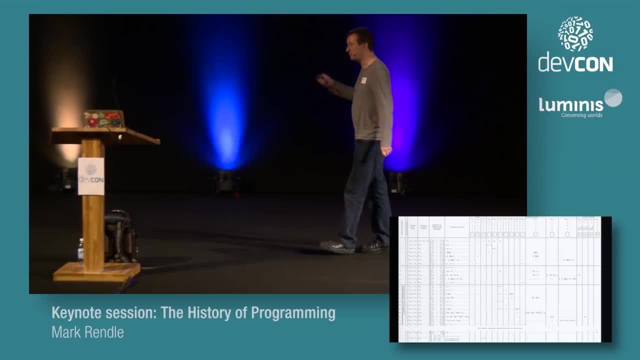 the code was unbreakable and the british people were trying to get the paper to do trickery all the time and but what they were doing was trying to get the paper to do trickery and they did it and British went. well, let's see about that, because we've got this chap: Alan Turing and Alan Turing. 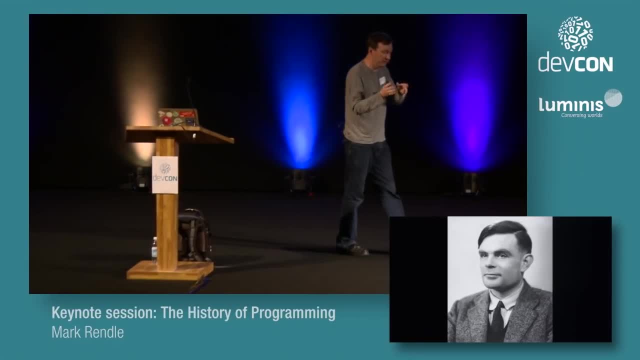 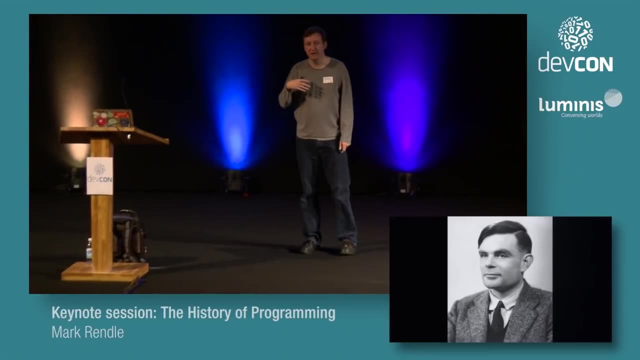 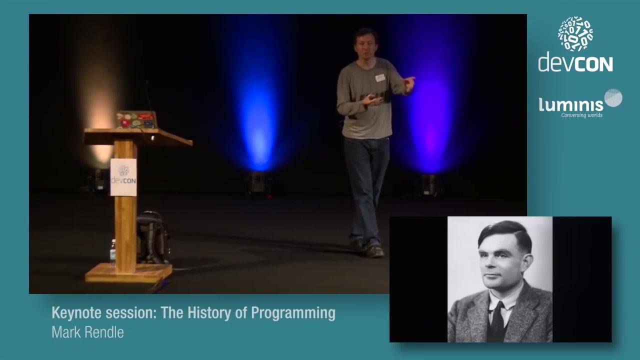 really, out of all the people I've mentioned so far, Alan Turing is the guy who is the the father of modern computing. he's the guy who came up with the idea of a universal state machine, a thing that could be programmed and change its own programming while it was running. and 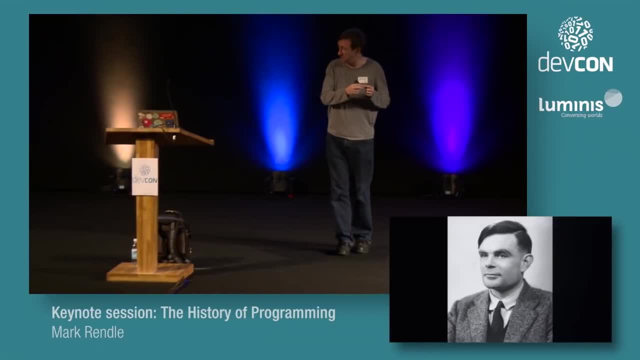 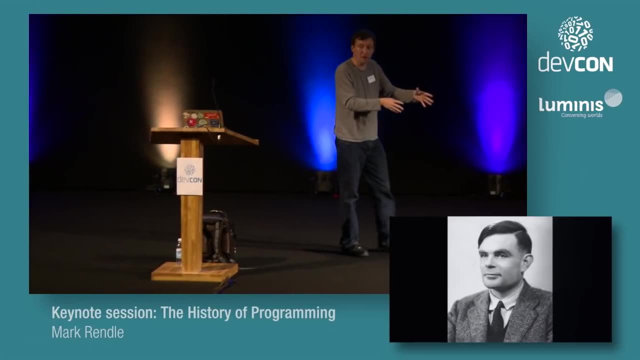 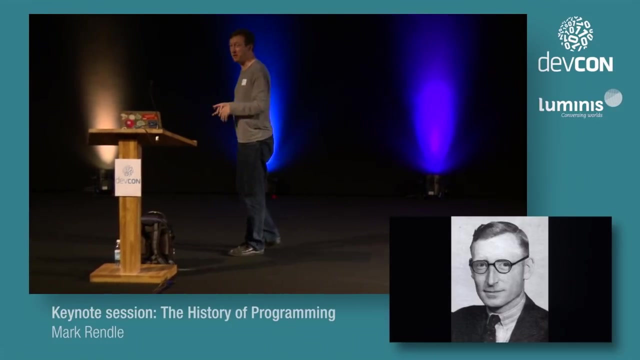 in his kind of thought experiment version of it. it was just an infinitely long bit of paper tape, but he built, well, he designed the first programmable computer. this chap built the first programmable computer and you don't see so much about this guy. this is Tommy Flowers. 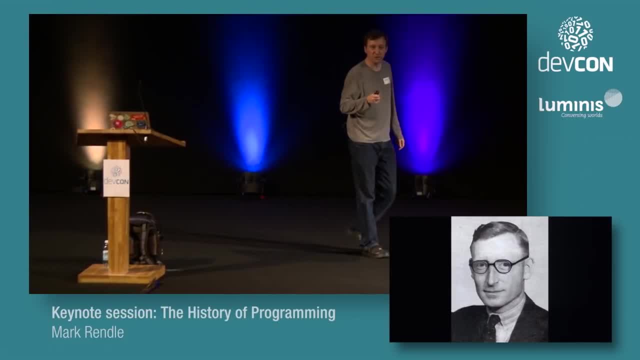 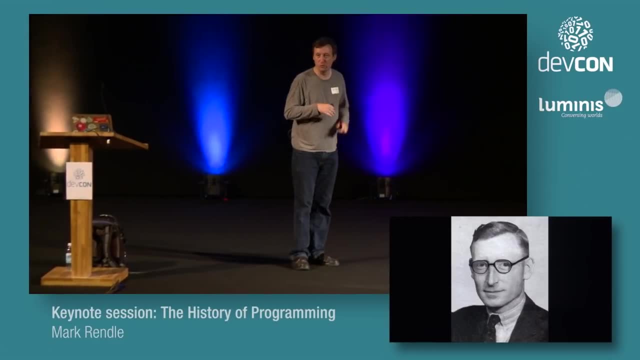 and he's one of my heroes because nobody knows about Tommy Flowers. Tommy Flowers worked for the post office in Britain and he worked with telegraph relays and telegraph relays- uh, basically, when you've got a telegraph, you've got a very long. 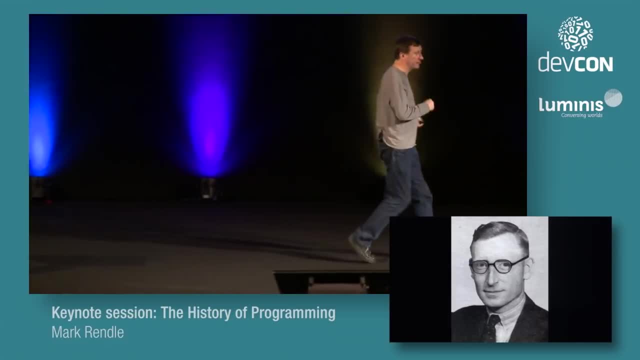 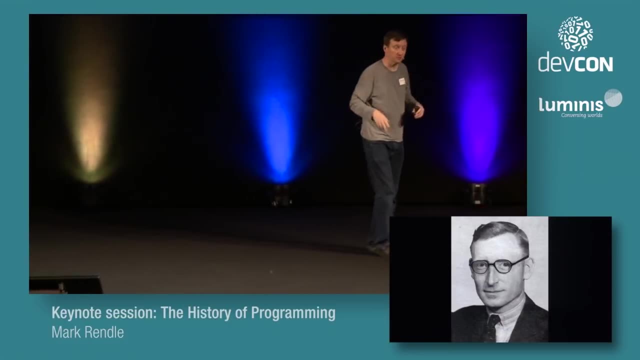 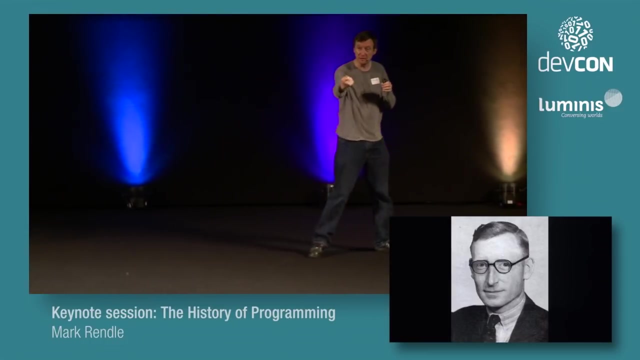 wire that goes from there and it goes all the way over to here, like this, and as it, as the electricity goes along, it kind of weakens. you run out of electricity after a certain while. so telegraph relay is a magnetic thing, and when the power gets to this end it closes the magnet which then forms. 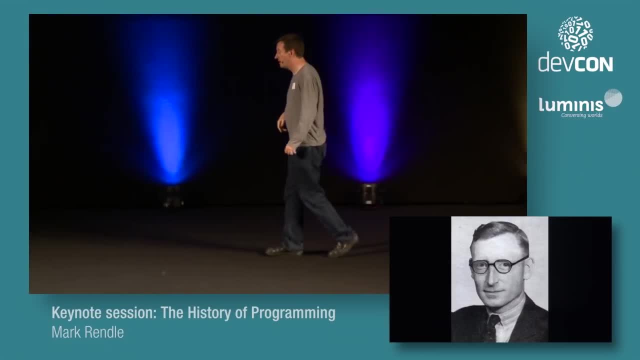 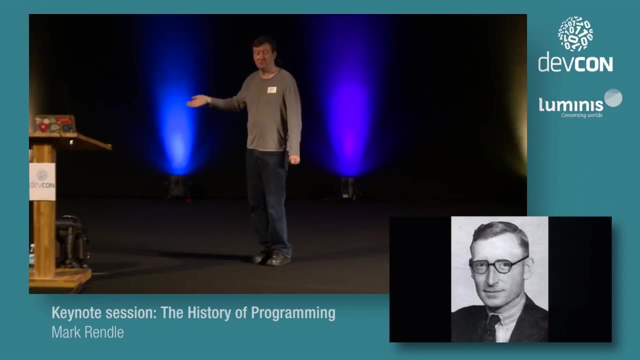 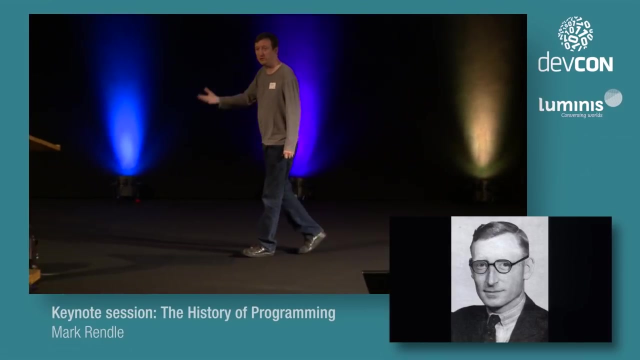 a new circuit so you get new electricity going down the wire like that um, and that means you put current through it and it goes on, and you take the current away and it goes off. so it's basically a transistor. and so tommy flowers built a programmable computer with and and not and, xor and all this sort. 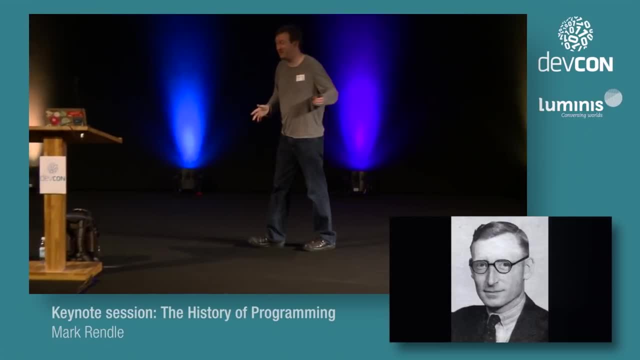 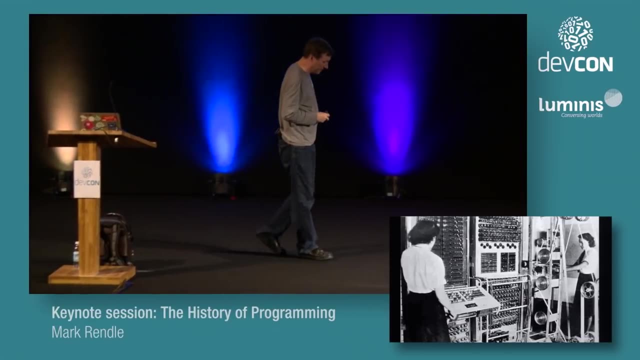 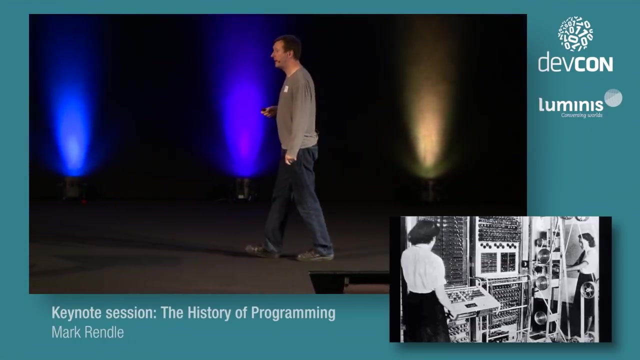 of stuff out of telegraph relays, which is just i, i find that spectacular. here's colossus. that's, that's what colossus looks like. um being operated, um being operated, um being operated and programmed, uh, by a couple of ladies there, um, and that was at bletchley park. and then when 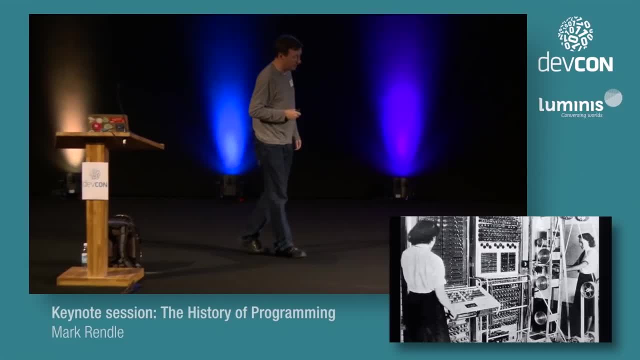 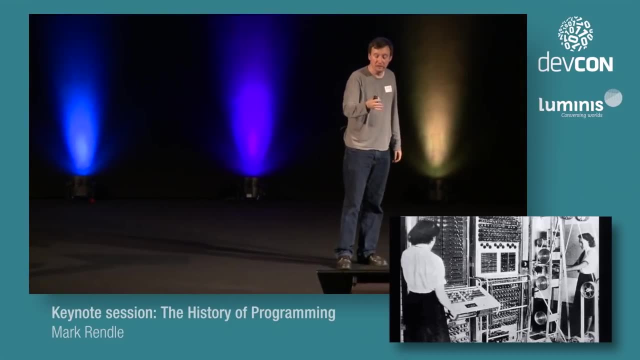 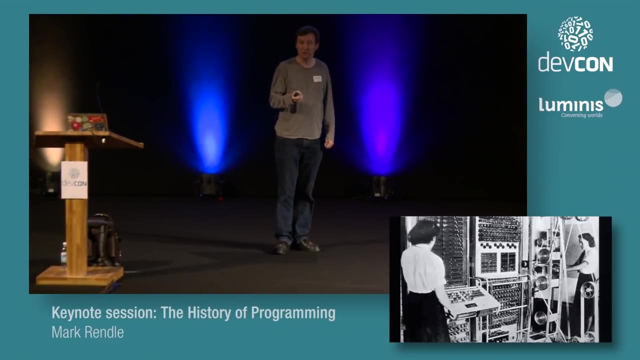 we won the first, the second world war, uh, and, and we, we beat the germans in no small part. uh, down to the, the work done by the people at bletchley park. the government said: we can't let anyone know that we know how to crack the enigma machine. um, because what we're going to do now is we're going to say: 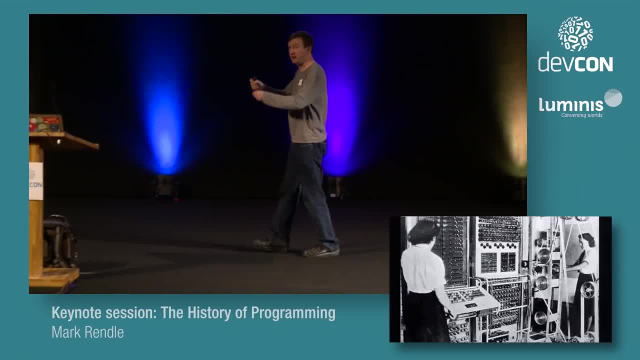 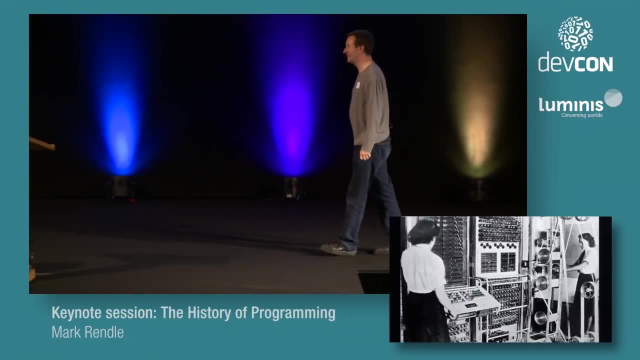 we've captured all these enigma machines from germany so we'll give them to all the different countries and you can use these for secure, secure communications and we'll know what you're talking about. yes, oh, it's. it's good that the british government these days is so much more enlightened. 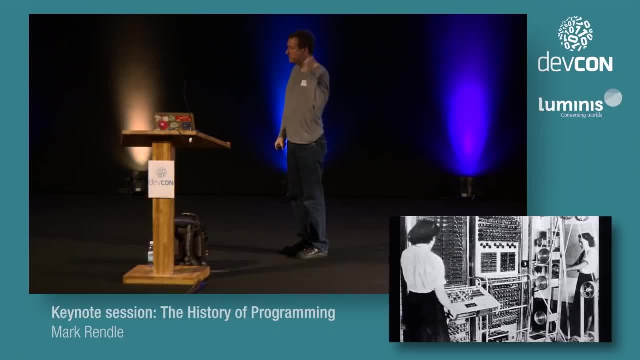 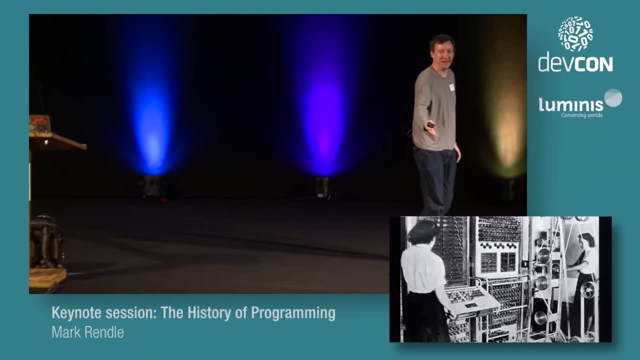 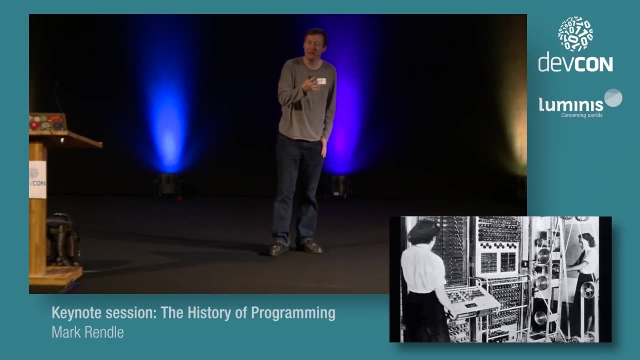 than that or not. so they smashed it, literally everything that was in there. they took sledgehammers to it and they smashed it up and none of the people who worked there literally on pain of death. they weren't allowed to talk about what they'd done. 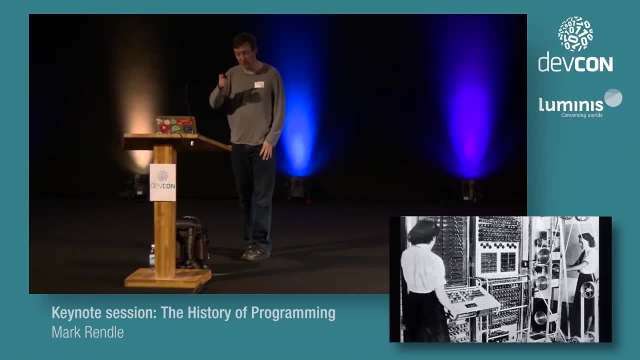 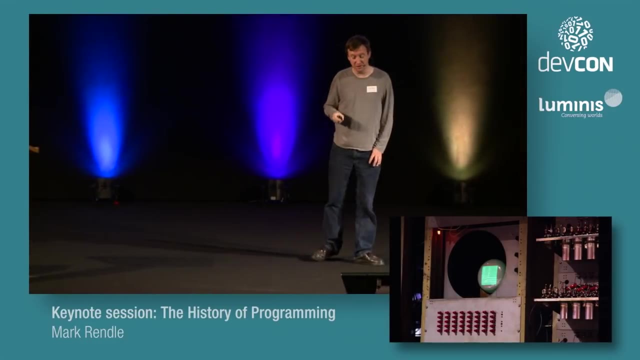 and it only came out 50 years later, after the official secrets act wore off and everyone went: wow, that was quite impressive. so nobody knew about colossus and so everyone thought that the first computer was this is. this is a little bit of the first computer, you. 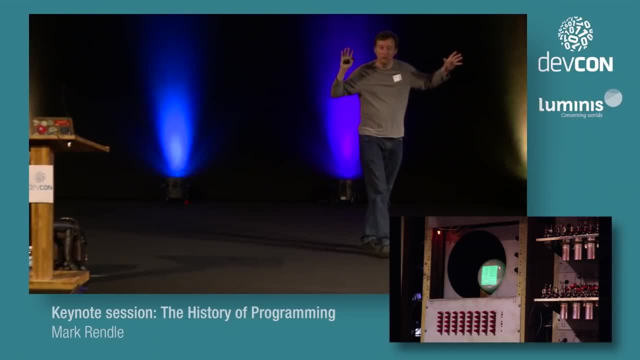 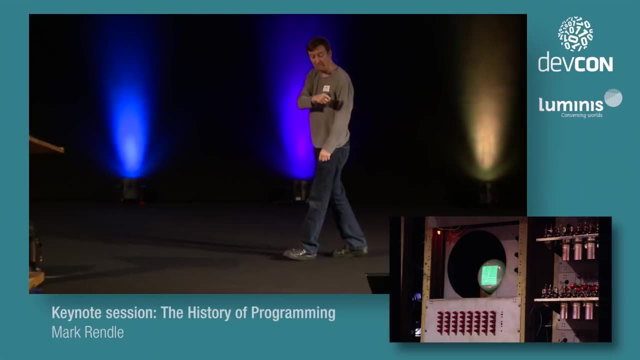 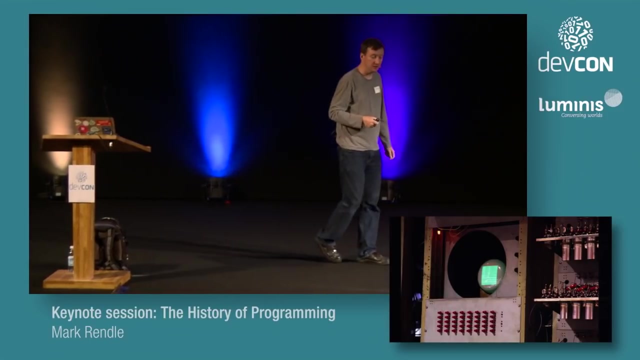 can imagine that the first computer was basically a room with a lot of of stuff inside it. uh, this is the- uh, the readout from the first computer. this is the manchester baby. um, it has a boring name as well, but everyone called it the baby, and this was built in manchester just after the- uh, the end of. 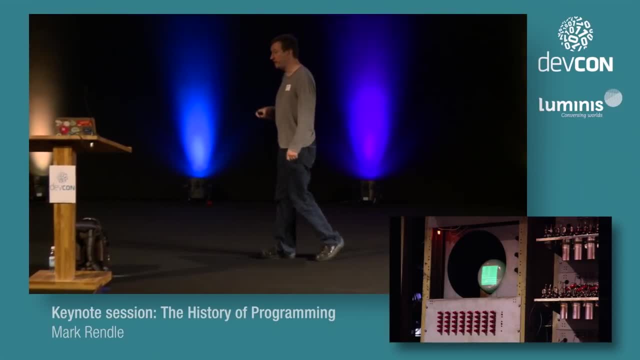 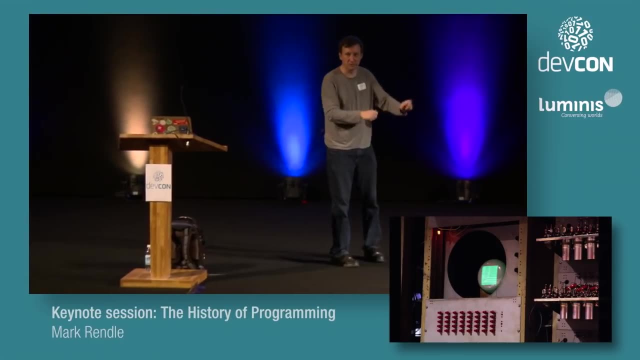 the second world war. meanwhile over in the states they were building eniac and all these sorts of things and the manchester baby, those switches and stuff and you'd like a range of the switches and then push a button and it would like light up some lights and everyone was very excited about that. 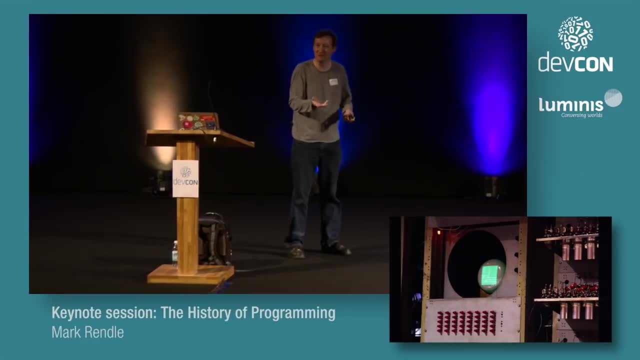 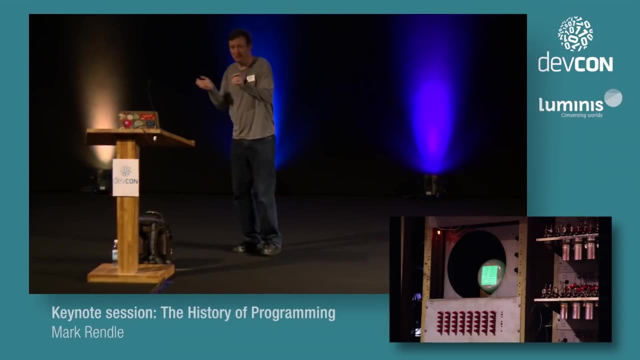 um, kind of like a raspberry pi. when you has anyone like got kids and and done something with a raspberry pi with their kids and you know one minute they're playing xbox one and throwing things around and stuff, and then you get them to kind of light up, every alternate led and they go. 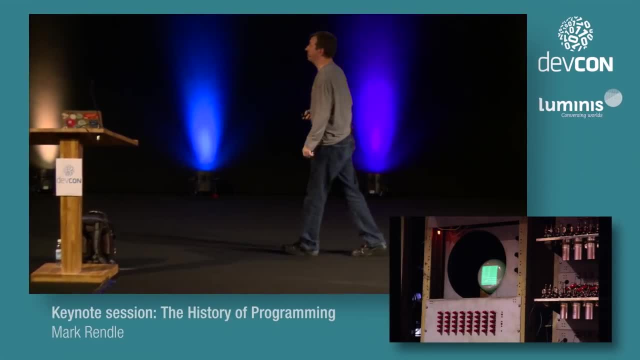 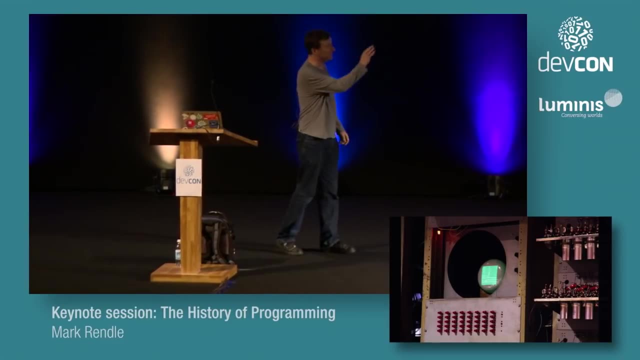 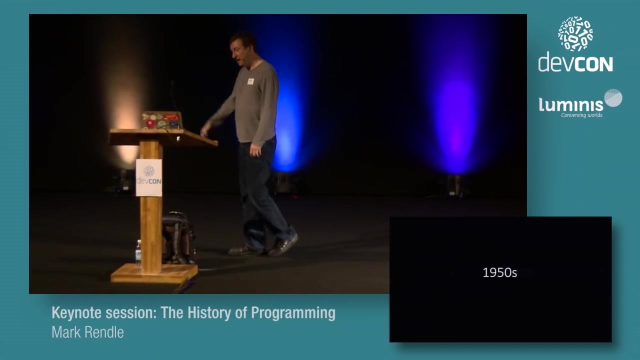 that's the best thing ever. can i go and play xbox again now? but yes, so. so by the end of the 1940s we'd kind of got these mechanical things and some of them could hold, had kind of limited memory and vacuum tubes and so forth, and then the 1950s is where programming really became. 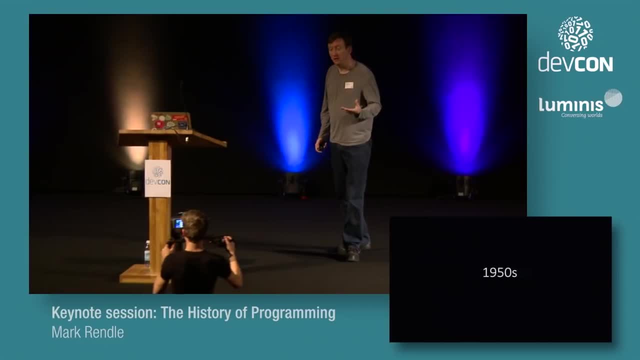 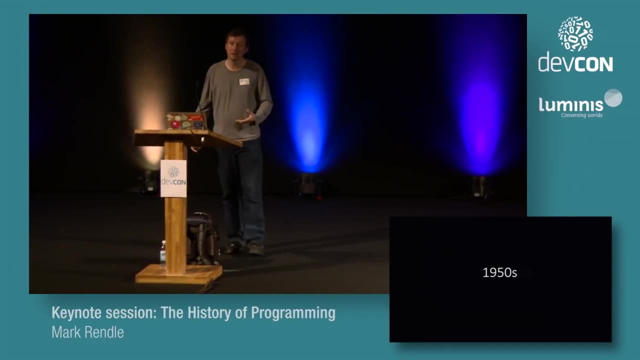 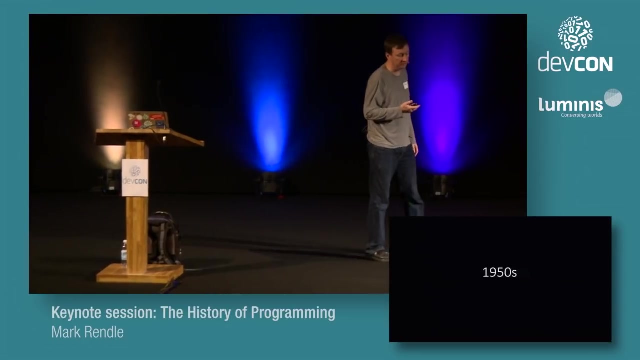 a thing and we started to get programming languages so we could express what we wanted the computer to do in terms that sort of made sense to us and also made sense to the computer. and the first programming language, uh, that really counts as a programming language and not just. 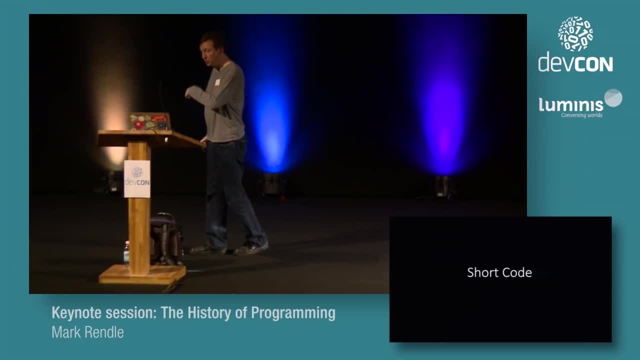 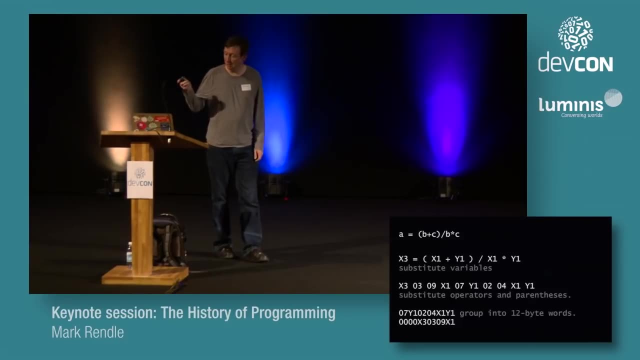 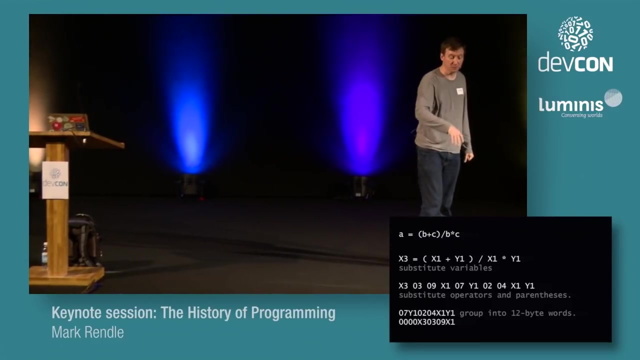 setting the various bytes was something called short code, which was created by somebody who was working at ibm and i've got a sample of some short code here and you can see. so the top bit there is short code. that's how you express it, and then what you do is you've got a set of predefined 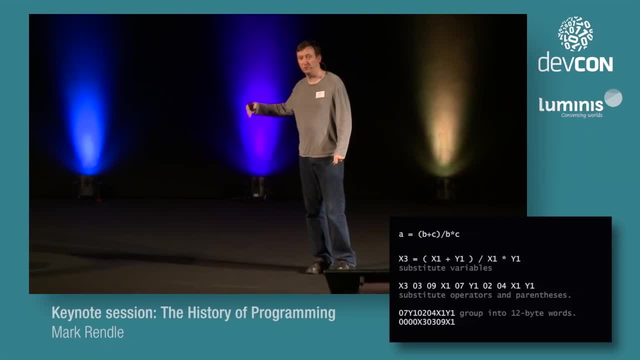 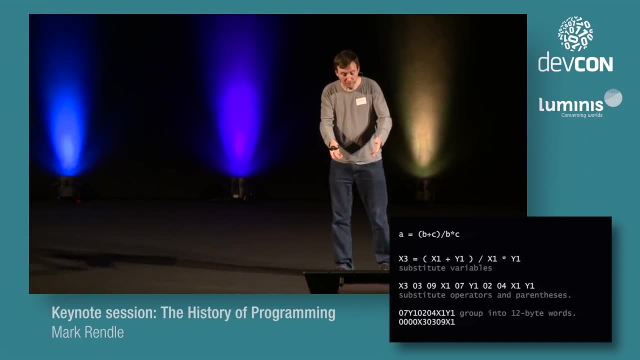 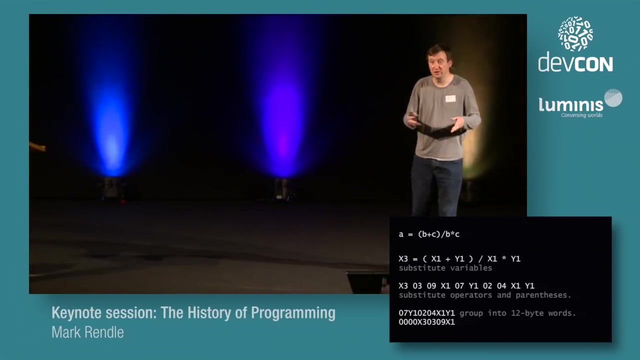 variables, which are all x1, x2, x3 and y1, y2, y3 and so forth, and so you replace the variables in your statement with the actual variables that the computer gives you, and then you replace the operators with the numbers that return to those operators, and then you group all of that into 12. 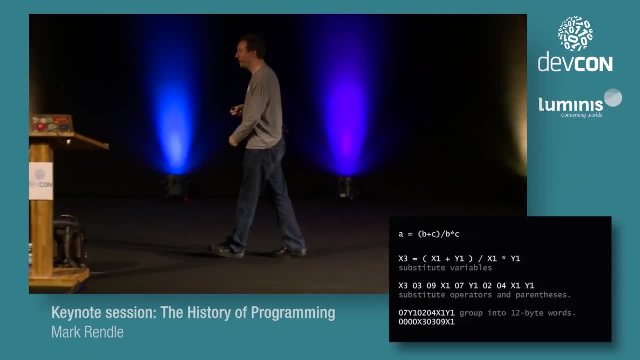 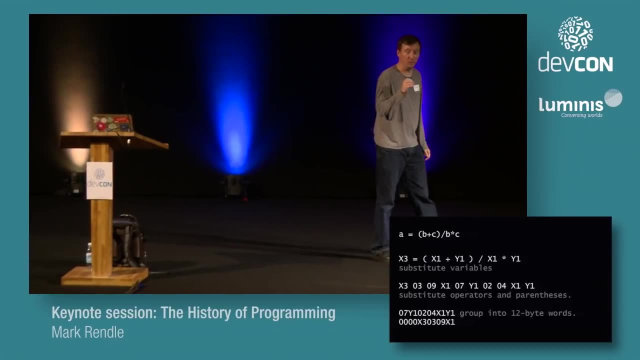 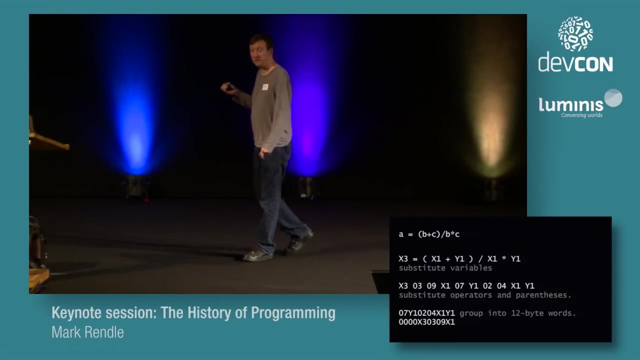 byte words and you've compiled your program. and in the 1950s, compiler was a job title and there were people that was. that was what you did. you were a compiler- and actually the vast majority of compilers in the 1950s- because women were better at that sort of they could do this more um accurately and more. 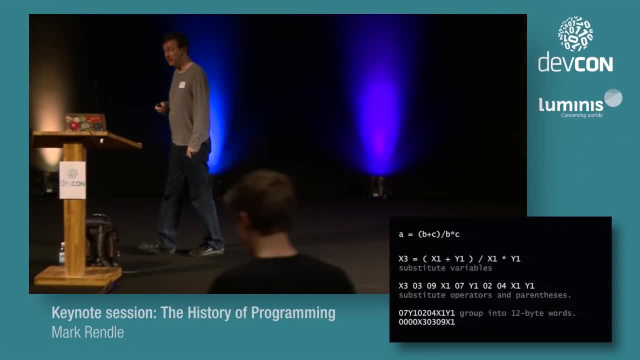 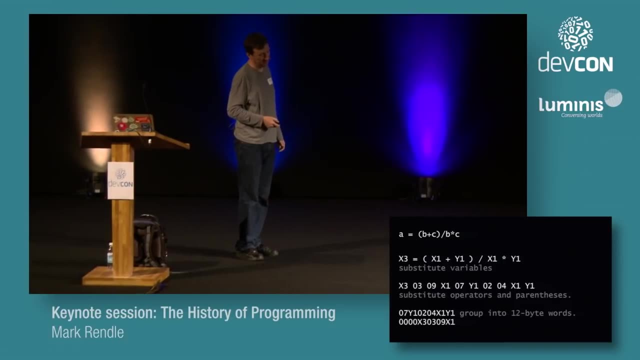 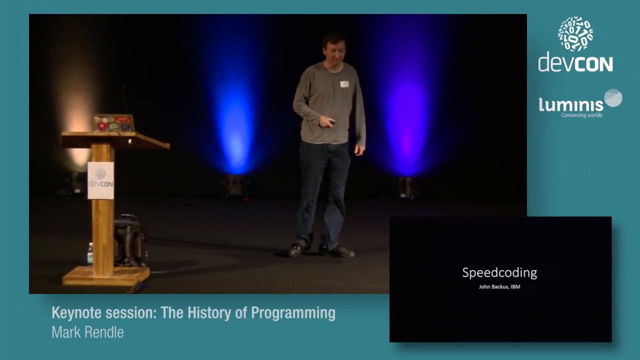 they made fewer mistakes than men go figure. so, yes, so that was. that was short code, not particularly short, uh, and not a particularly short process. and then, um, ibm said, well, that that's a bit faffy, let's, let's create something else. and they called it speed coding, which really that's very optimistic. 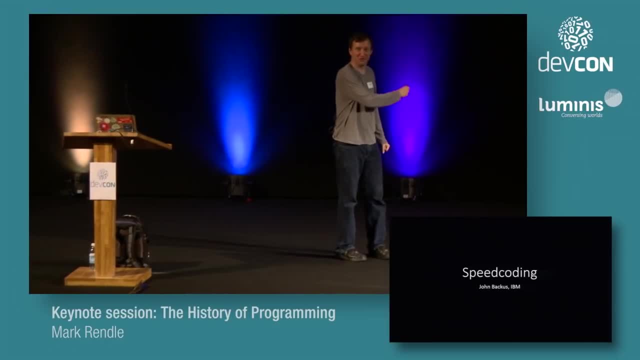 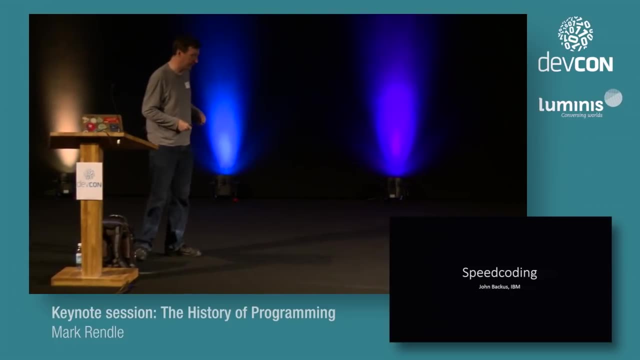 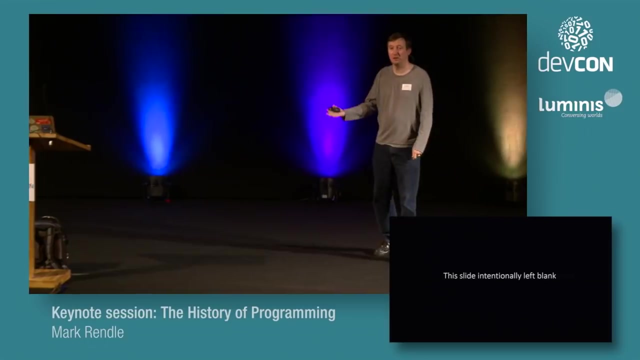 at the start of a revolution going: this is it. this is the fastest it's ever going to be. in 1952, uh, john backers, who was working at ibm, created speed coding- and that's an ibm joke anyone who's as old as me will remember. before the internet, everything used to be binders with. 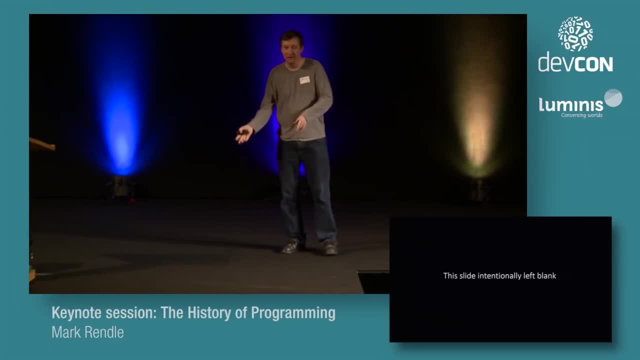 pages in them and pages and pages and pages. and ibm would have these enormous great binders full of pages and so on. it was like everybody could write in them and they knew what to write in them at the moment of their Nejera day, in of And iPm words you might not, But clinicensis wrote so many of those and the, notamment in 167 degrees of. 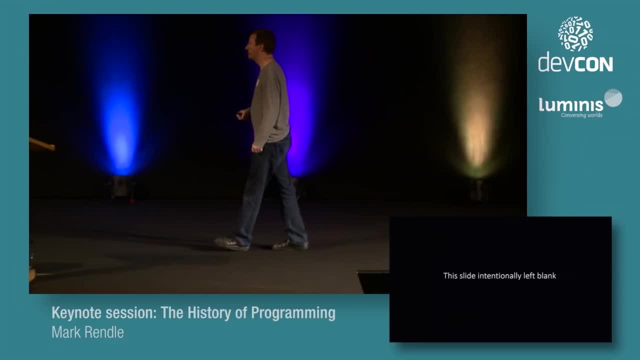 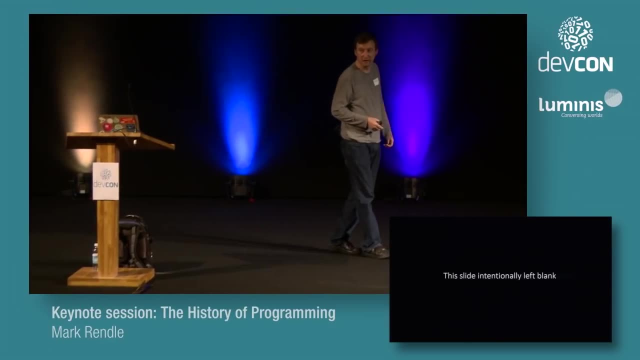 Several of them would say this page intentionally left blank, just so you knew it wasn't a printing error, and then another 10% of them would be blank, but without this page intentionally left blank where presumably some important information had once been. 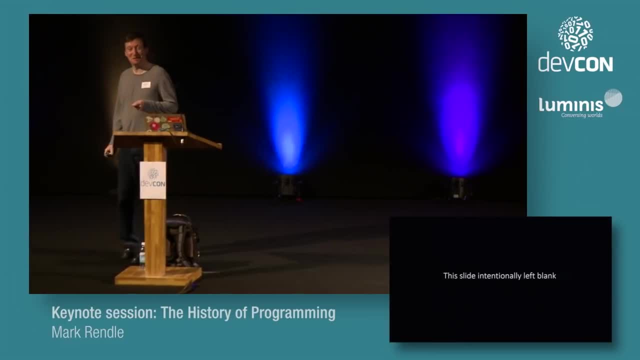 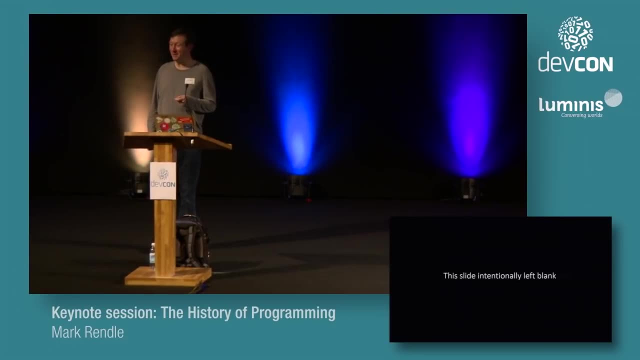 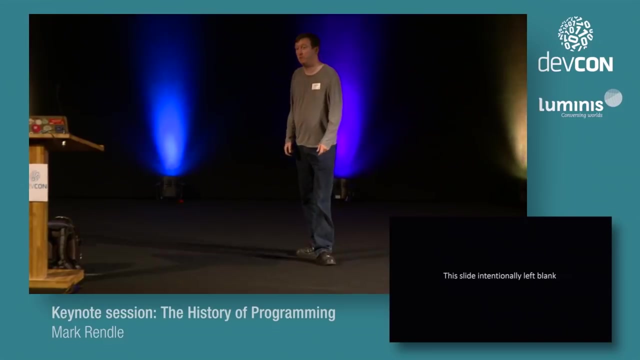 I don't like IBM, by the way. Does anyone here work for IBM? Hello, We're going to have fun, you and me. I couldn't find any samples of speed coding code, probably because nobody was ever able to write any. 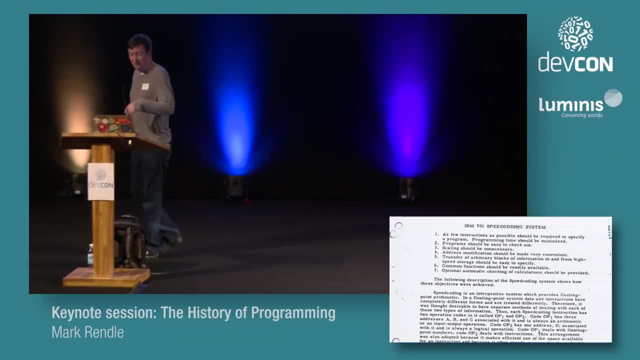 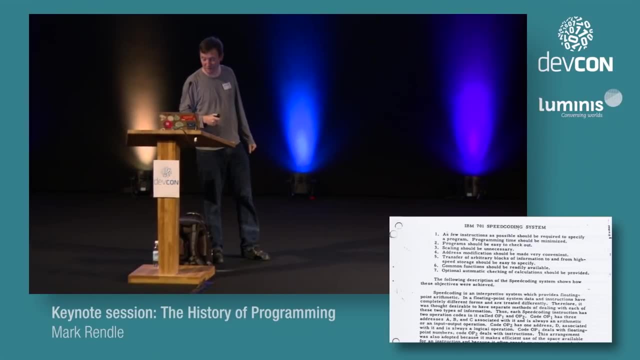 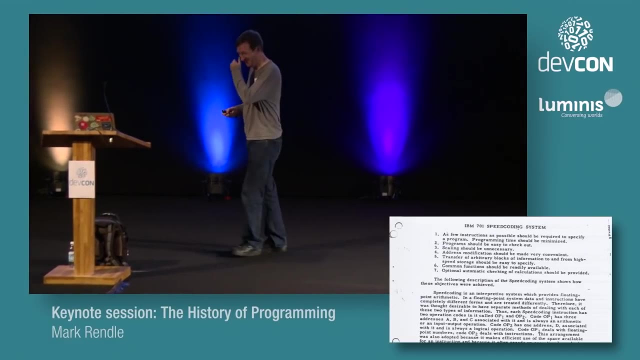 because half the pages were missing. This is something from the speed coding, IBM's 701 speed coding system. As few instructions as possible should be required to specify a program. That's not something you expect to hear from IBM, But yes, So I couldn't find any of that. 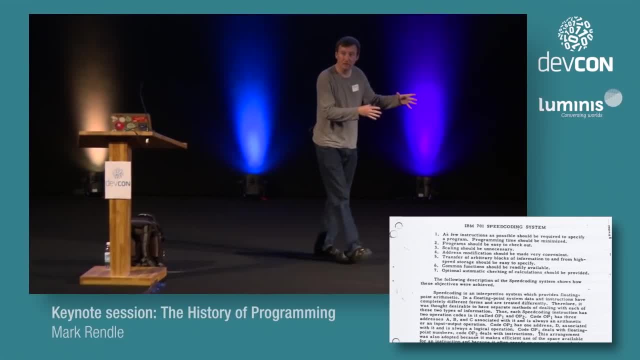 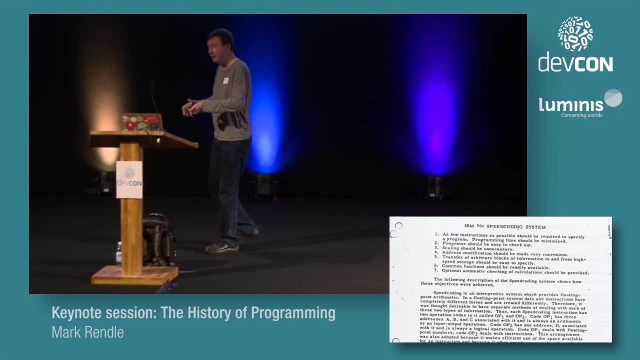 But so in the 19,, like I said, compiler was a job title and for speed coding as well. it was kind of like scribble it down as quickly as possible and give it to somebody who actually knows what she's doing. 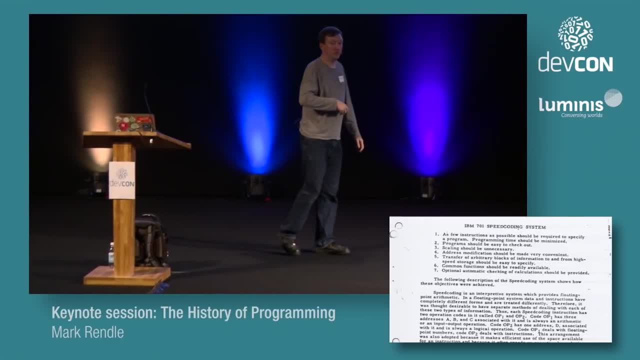 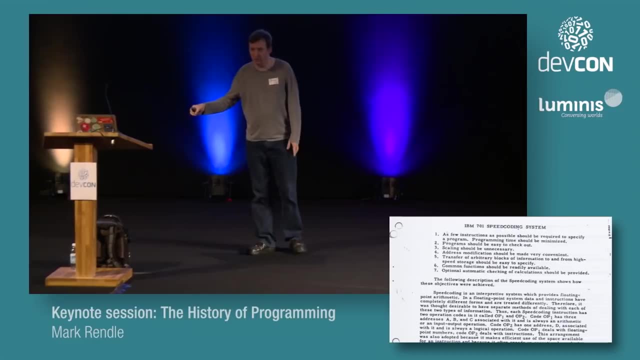 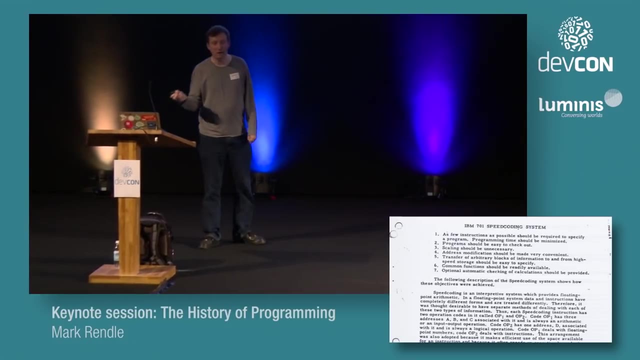 and she'll make the computer run that for you. But then someone went. it seems like this idea of taking symbols and translating them into other symbols. isn't that essentially what we've built the computers to do, And couldn't we therefore get a computer? 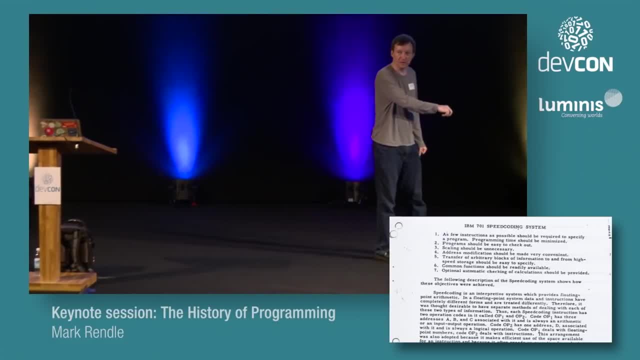 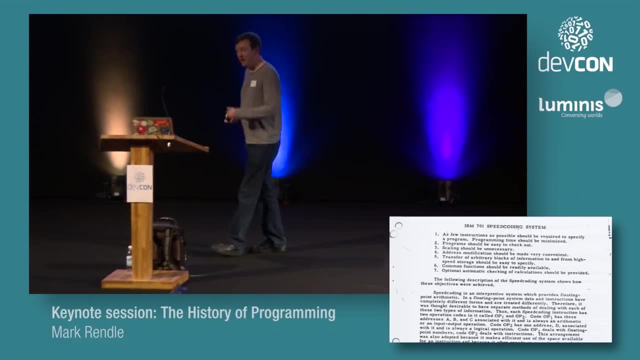 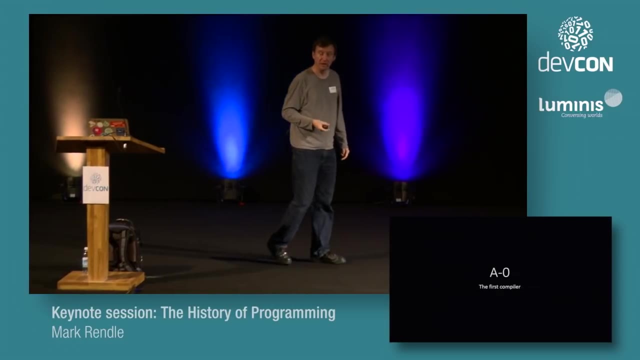 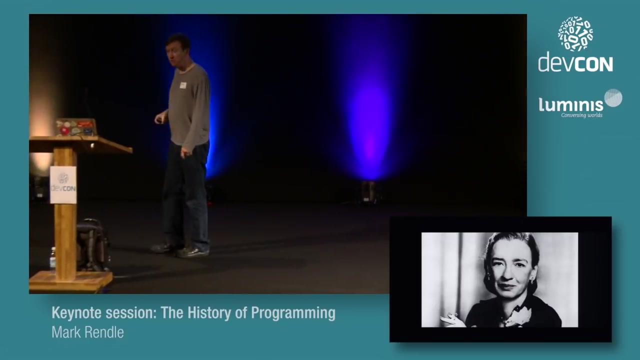 to automate this so that all these people can be unemployed, Thereby starting a trend that continues to this day. And so somebody did, and the first ever automated compiler was A0, which is a good name for the first of anything, And A0 was created by Grace Hopper. 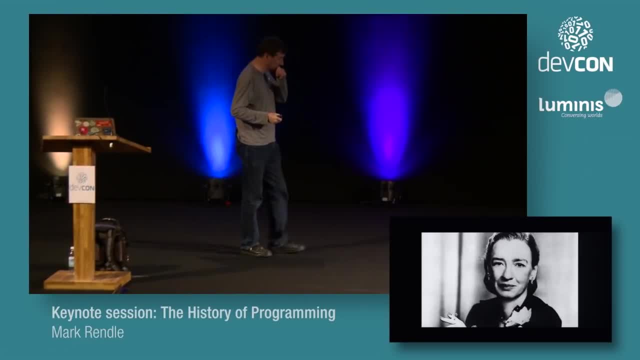 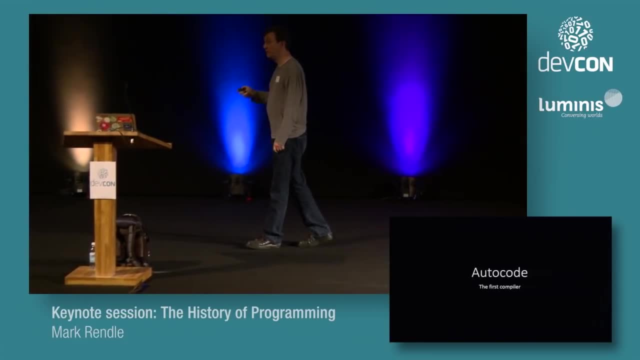 who was an officer in the US Navy and she created the first ever compiler. But the first ever compiler was called AutoCode and it was created by a man called Alec Glennie in Manchester, And A0 was created in the United States. 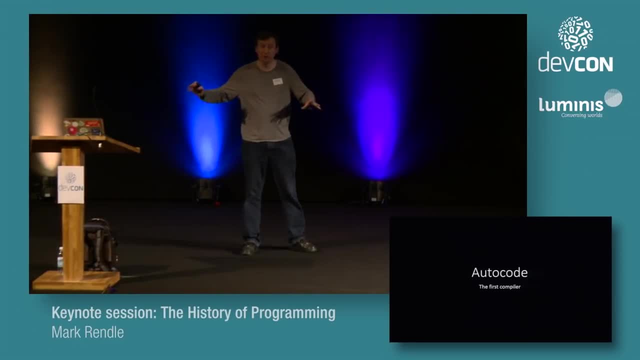 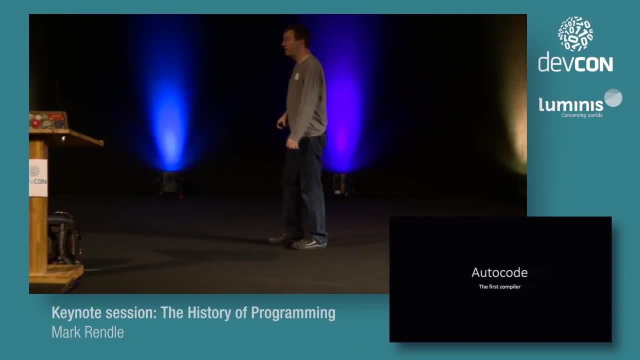 and AutoCode was created and they were both the first compiler. They were created at around the same time and there wasn't a lot of collaboration between the two sides, so they both said we're first Because of course they didn't have GitHub. 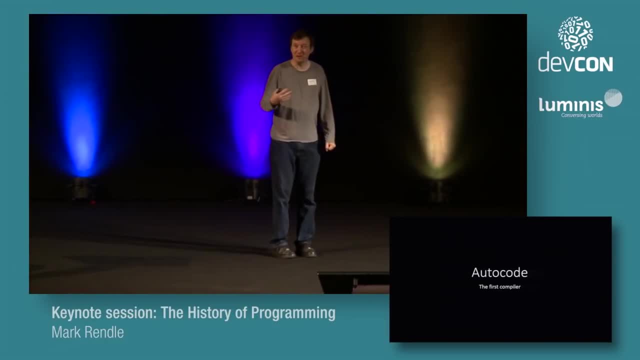 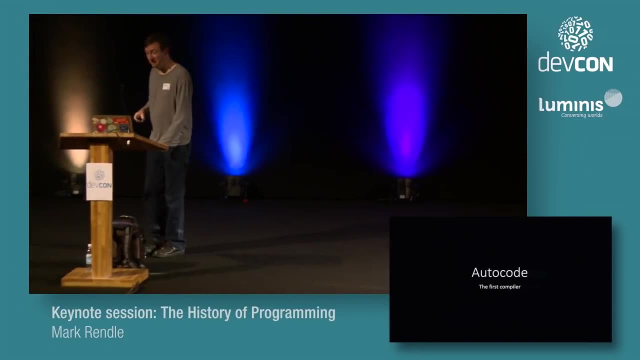 So you know, the duplication of effort, nobody went well. this is why we have open source, you see, because there was no concept of open source in the 1950s, because Bill Gates hadn't invented closed source yet. 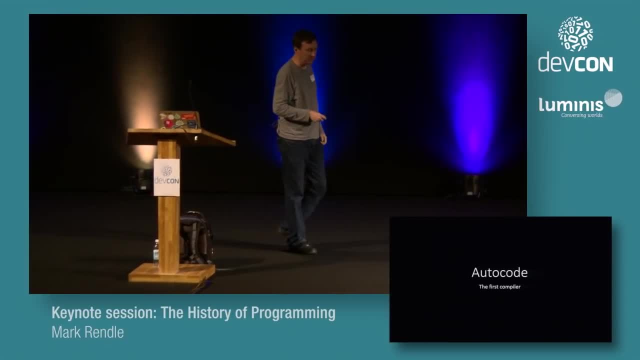 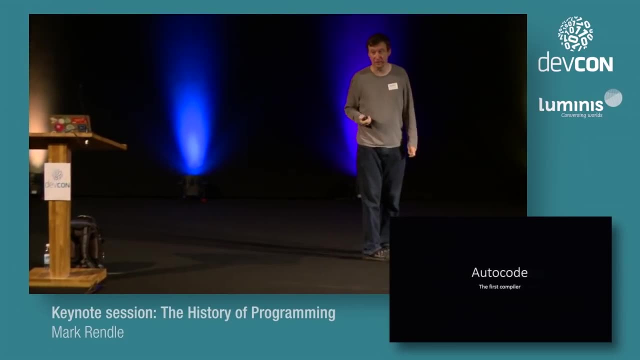 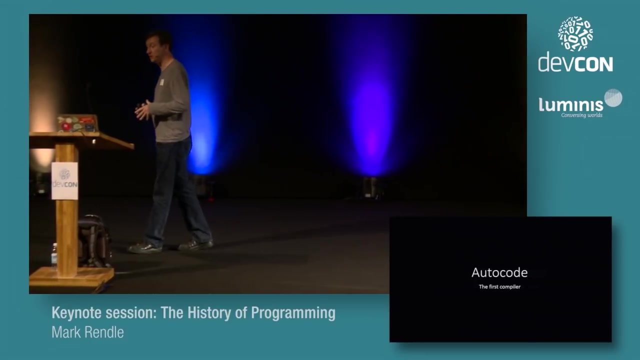 So, yeah, I couldn't find any examples of A0 or AutoCode either. The first language that I could find, that actually I could find examples of, is a language. it's the first real programming language that you would recognise today as a programming language. 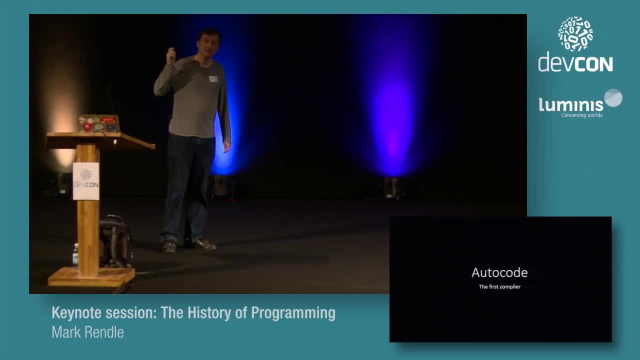 and it is still around today. Any guesses? Fortran. Fortran John Bacchus created Fortran John Bacchus. well, yes, he created Fortran for IBM, And this is Hello World. This is the first programming language in Fortran. 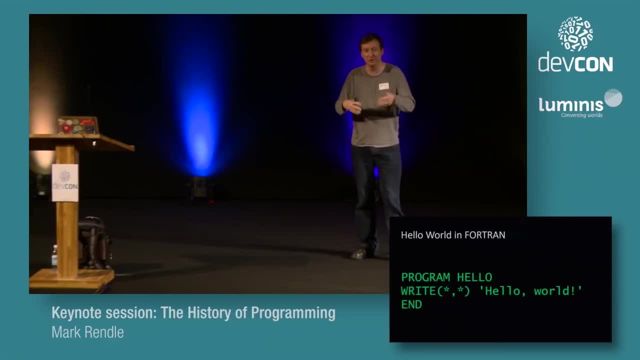 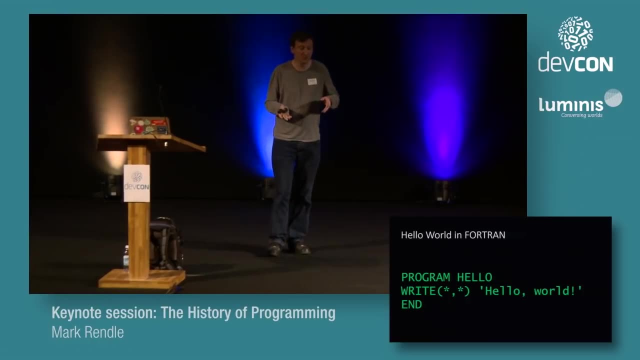 Except of course you couldn't just type this into a computer and have it come up on the screen, because they didn't have screens, And you couldn't even type it into it because they didn't have teletypes. So somehow this still had to be turned into something. 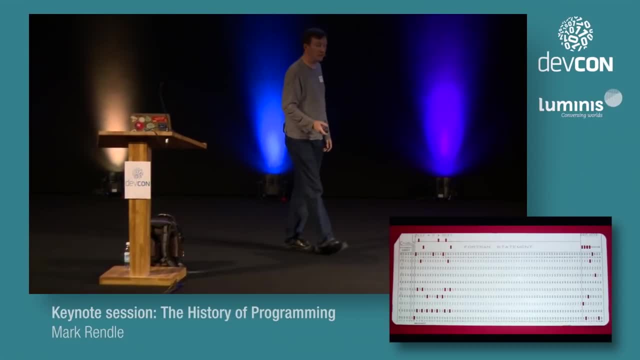 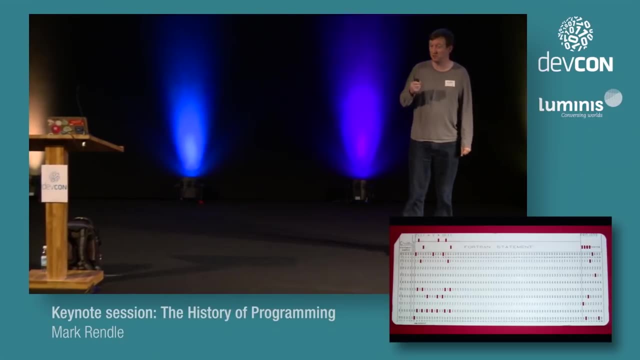 that the computer could understand, And so you would write your programming in Fortran, but then you would encode it on a punch card, just like the thing that they'd used to program the Jacquard loom to make pretty pictures in rugs. 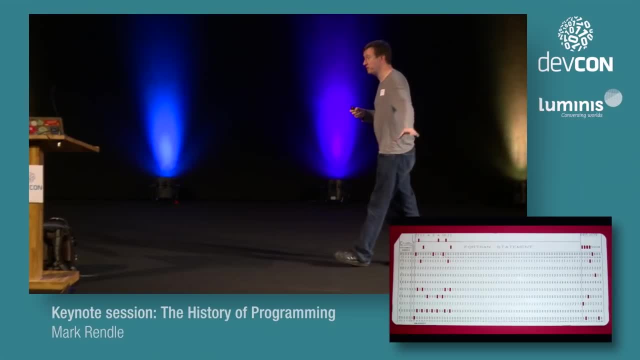 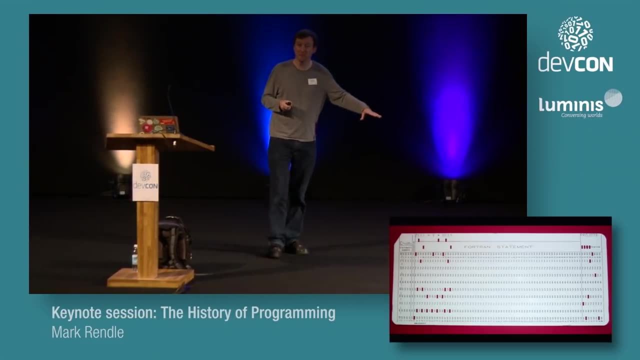 like you did previously, Except, of course, you couldn't do this because this was an IBM mainframe that you're talking to here and you weren't allowed to touch the IBM mainframe. There were people to do that for you. 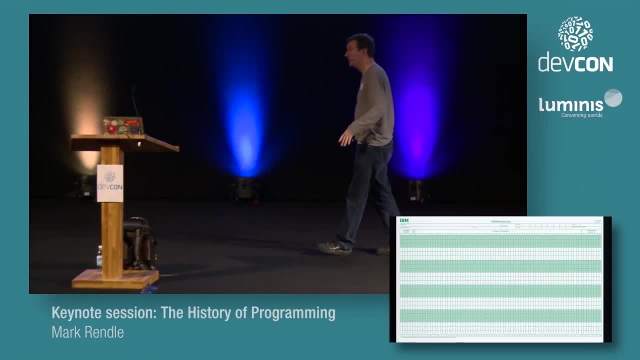 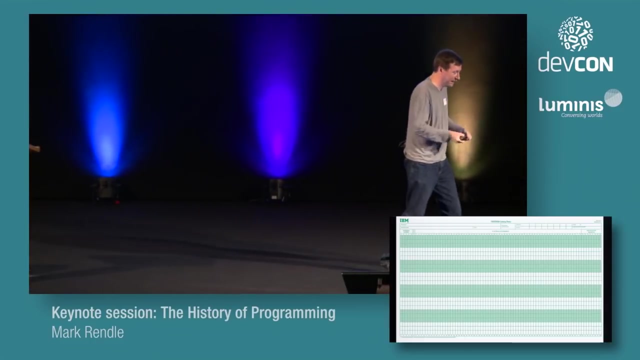 and people who would create the punch cards. So what you had to do was get one of these pieces of paper and write your Fortran program with a pencil on this piece of paper, and then put the pieces of paper together and hand them over to the high priest of the mainframe. 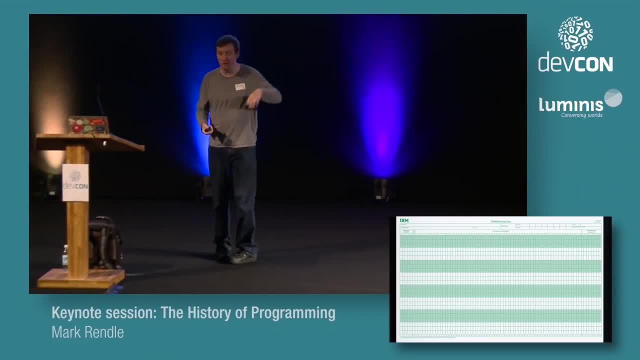 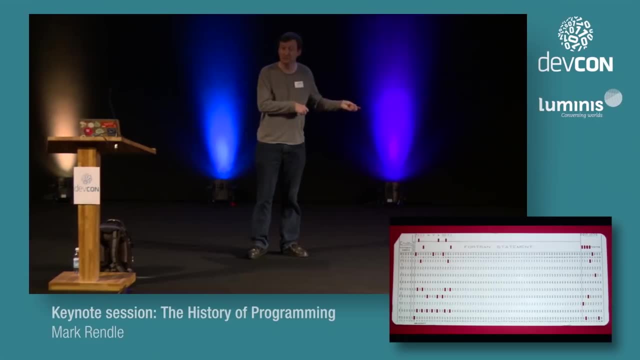 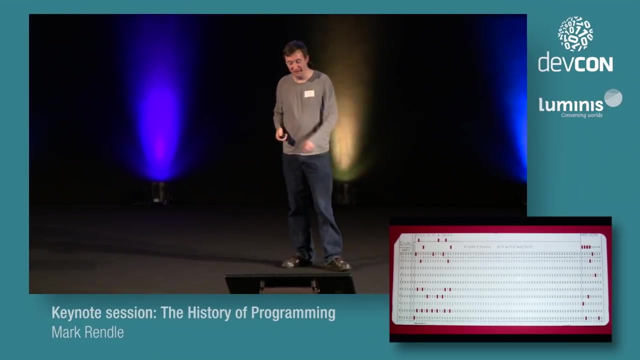 who worked for IBM And the high priest of the mainframe would go and create one of these punch cards and then feed them into the computer and then give you the errors that came out at the other end. And yes, and you know, these days we complain. 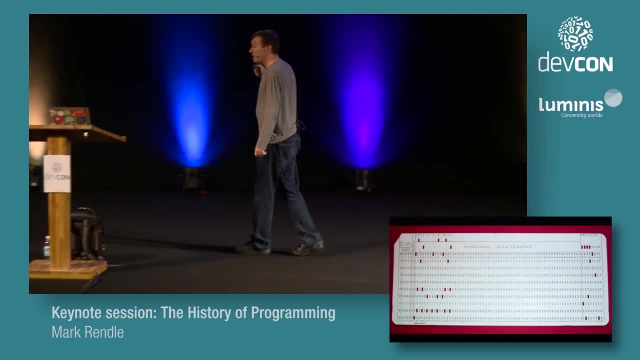 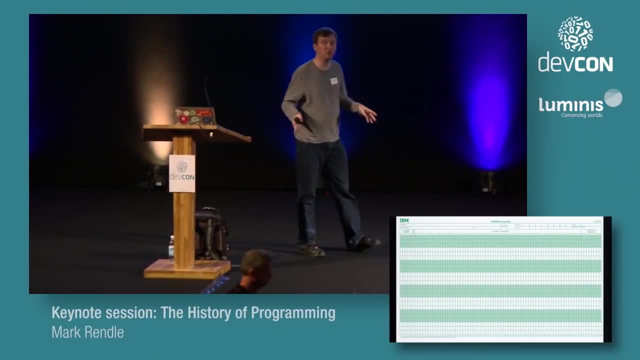 that C++ takes too long to compile. But yes, so, but yeah, Fortran First. this was in the 1950s. It was the end of the 1950s and it's still used today. 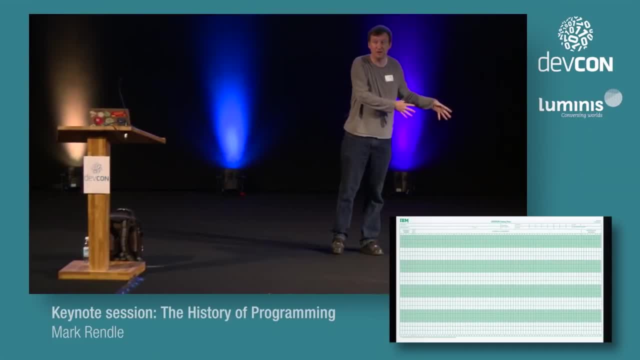 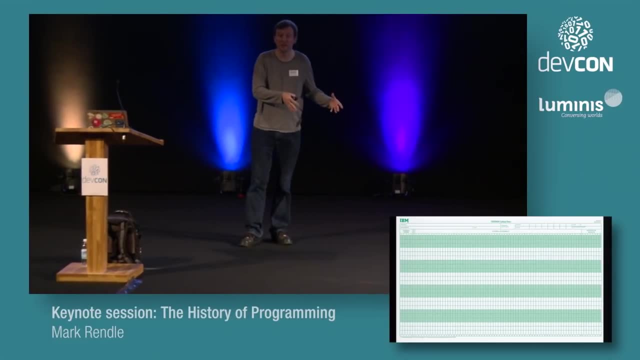 And one of the reasons it's still used today is because there are certain things it's really good at that. so far we haven't come up with any other languages that are that good at it, So like the SIMD instruction set. when the SIMD instruction set first popped up, 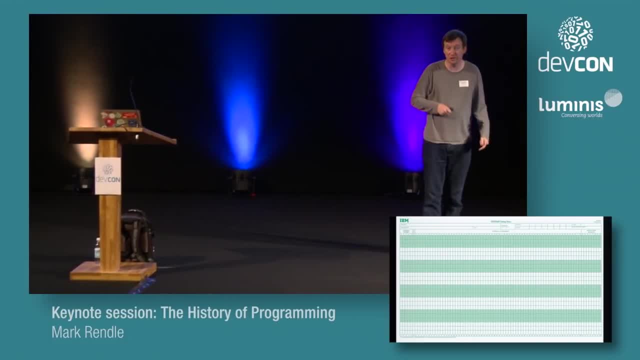 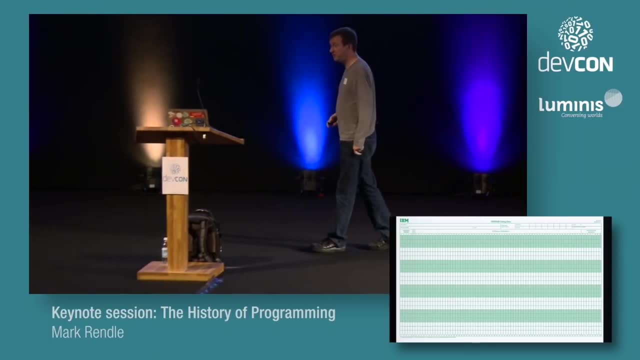 in the Intel processors. Fortran was the only thing that could actually talk to it, because Fortran was the only programming language that dealt in arrays as its kind of primitive type. But Fortran was also created by John Backus. John Backus, I didn't know this. 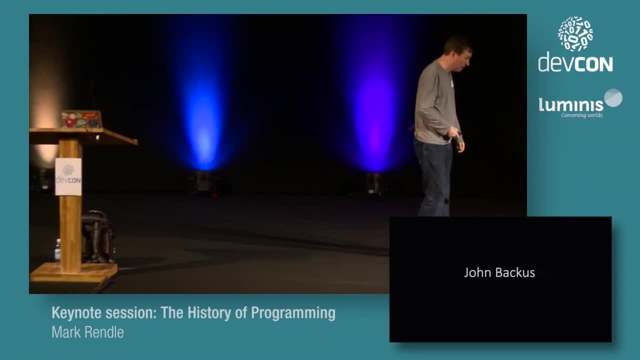 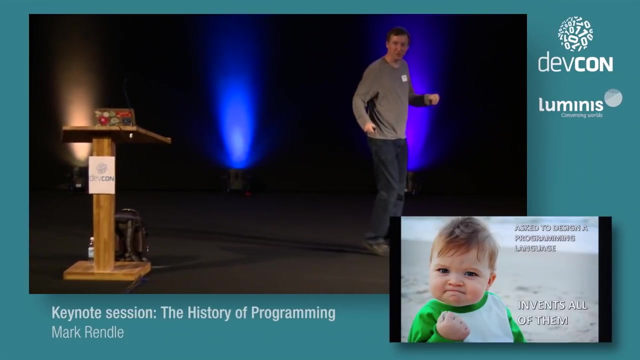 when I started researching for this talk, pretty much every programming language in the world, even the ones that are used today, are based somehow on a language that was created by John Backus. He was just, you know. they just went make a programming language. He went: here's 12. Take your pick, Because the next programming language that John Backus created was ALGOL And, as I'm sure you know, ALGOL became C and well, ALGOL became B. and then B became C, and then C became C++ and everything else, But ALGOL was the first C-like language. This is Hello World in ALGOL 58, which was the first version of ALGOL. ALGOL 58 didn't have IO. 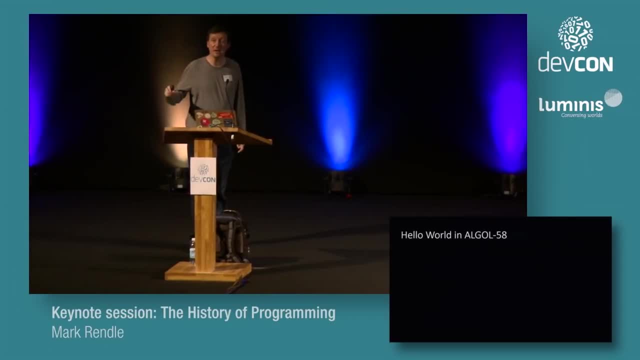 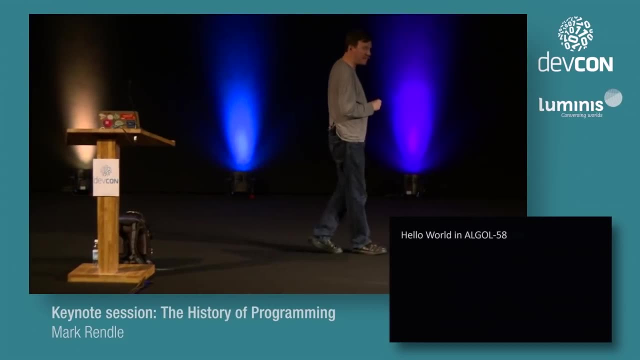 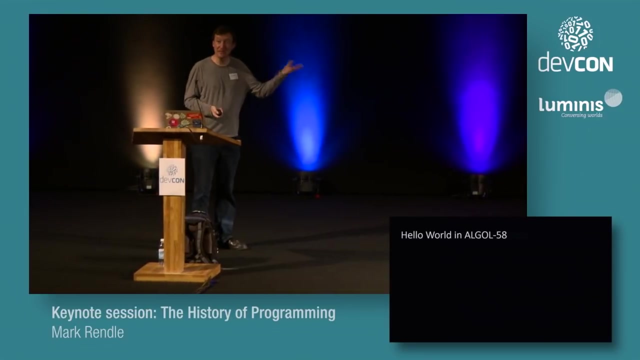 So there was no print, there was no read You literally you could not get in or out of an ALGOL program, Any Haskell programmers in the room. So, yes, ALGOL 60,. someone obviously took John Backus into a small room somewhere. 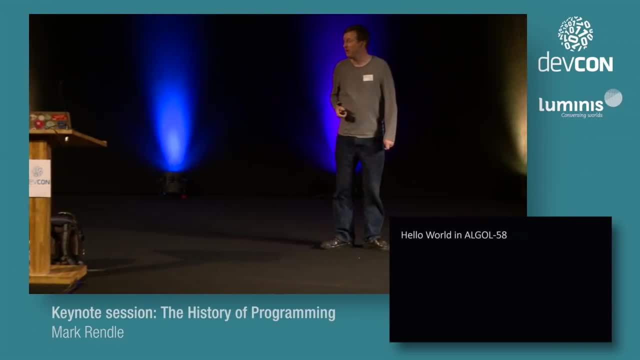 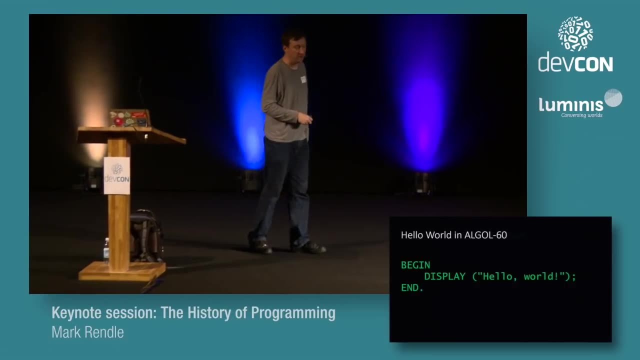 and had a meeting with him and went, John, little problem. So two years later ALGOL 60 came out. That's Hello World in ALGOL 60. And it's you know, this is starting to look really quite reasonable. 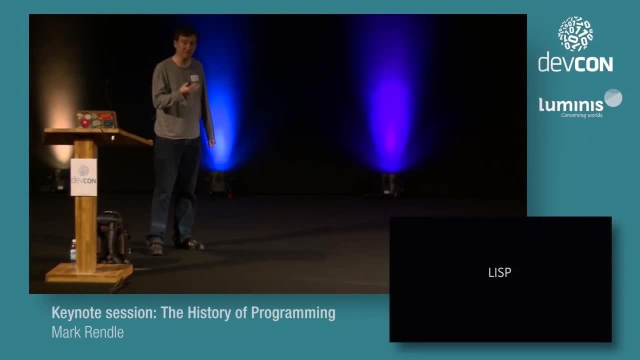 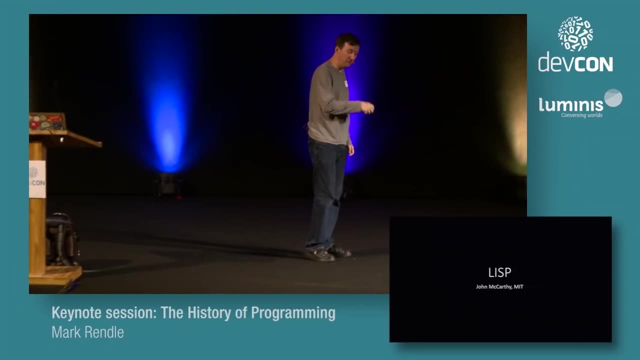 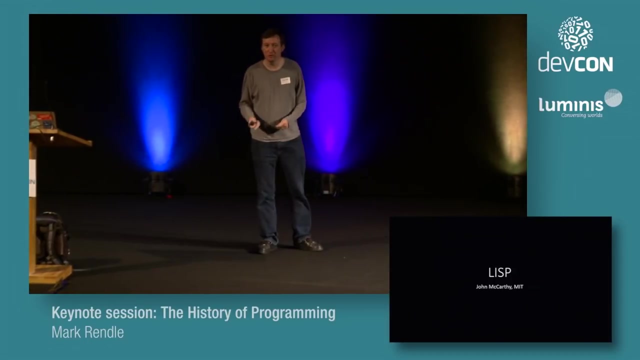 Also in the 1950s Lisp. Lisp was created at MIT by John McCarthy And the thing I find really fun about Lisp is these days you kind of go onto Hacker News or Reddit or whatever and there are people who do Lisp. 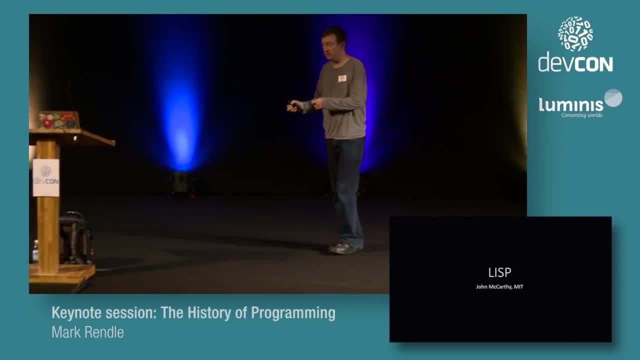 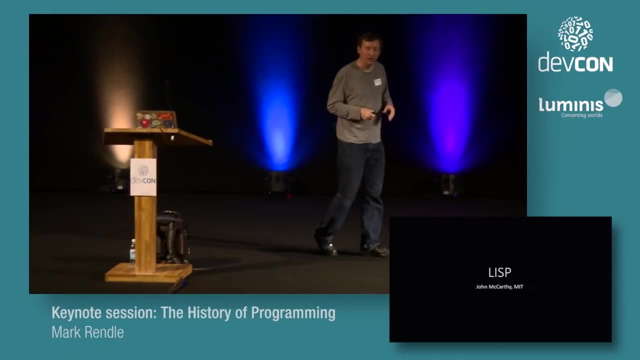 or who do Clojure and think it's Lisp, which it isn't for so many reasons, And they think they're really cool and hardcore and clever because they do Lisp. But at the time, in the 50s, Lisp was the programming language for the thickies. 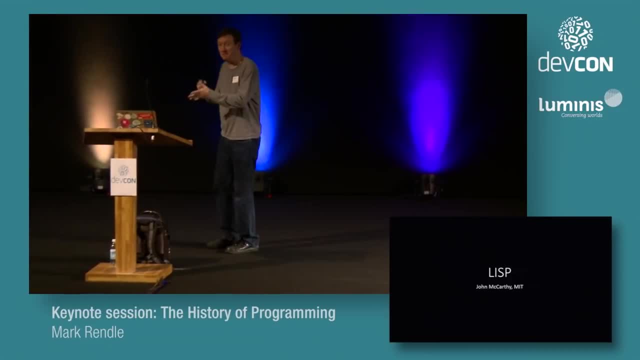 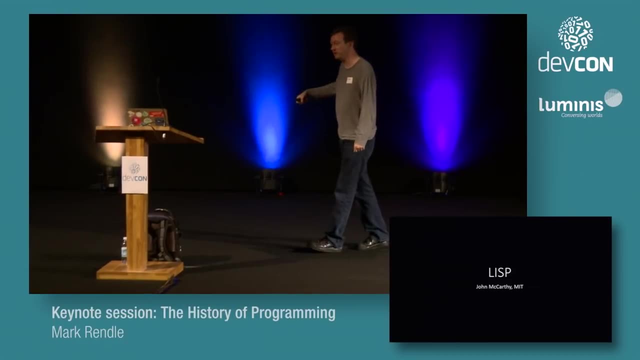 the stupid ones who couldn't actually understand assembly language. It's kind of like: oh no, your IQ is below 180, so you should probably just do Lisp and leave the hard work and the proper stuff up to us. So yes, 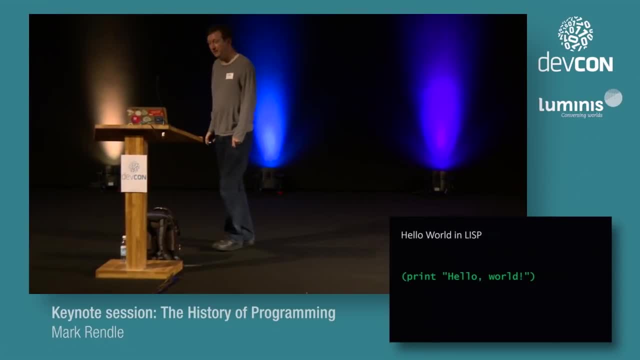 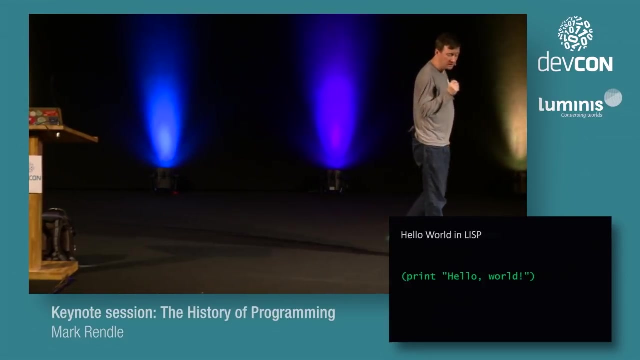 That's Hello World in Lisp. And then the last big advance in programming languages of the 1950s, Everybody's favourite programming language and unless I am the oldest person in this room- which is possible because I'm getting very old- 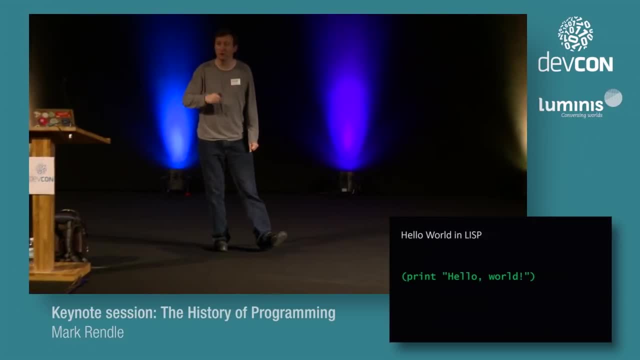 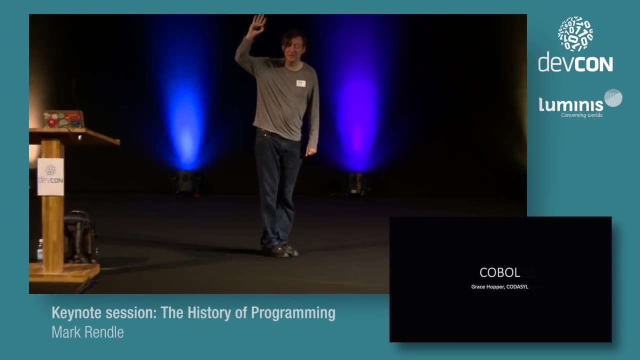 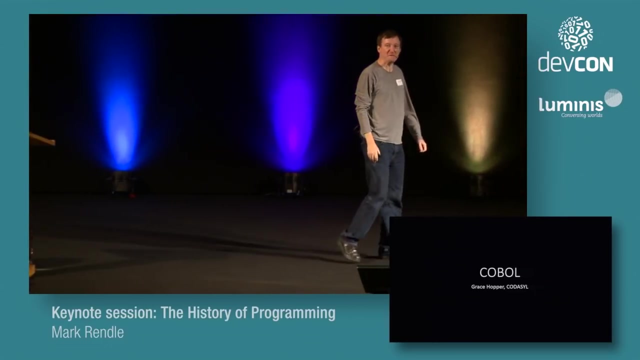 there will be people in this room who used to program in this programming language. Hands up, if you programmed in COBOL- Actually my first- There's two hands going up there. There's this guy going and I loved it Every fucking minute. Oh, those were the days. But yes, my first job was actually taking COBOL code and rewriting it in C to make it faster, allegedly, But COBOL was created by Grace Hopper was on the committee- but COBOL as those who have programmed in it. 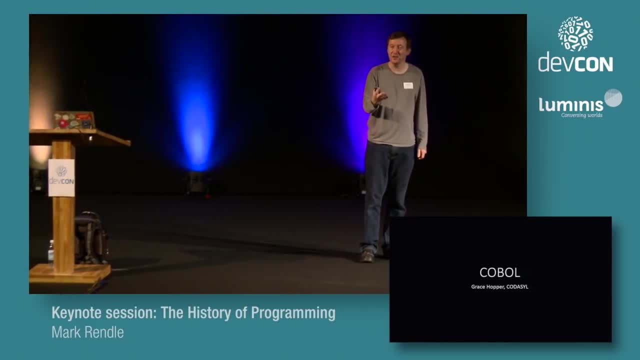 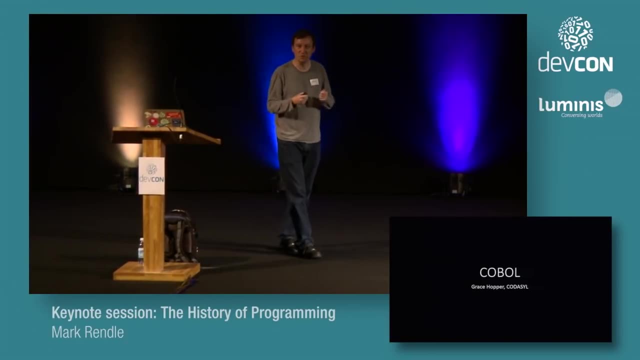 will be able to tell you was a programming language designed by God. It was a committee And it really really shows They. just The problem with committees is they don't know when to stop. So here's Hello World in COBOL. 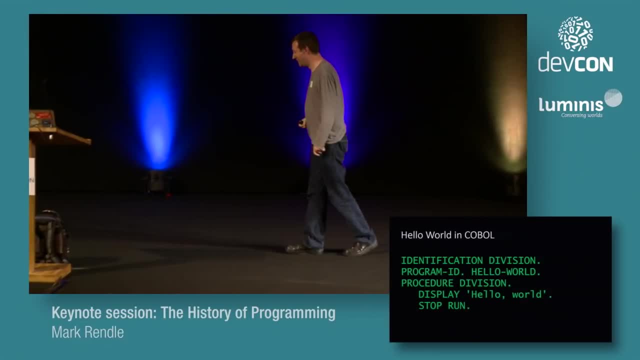 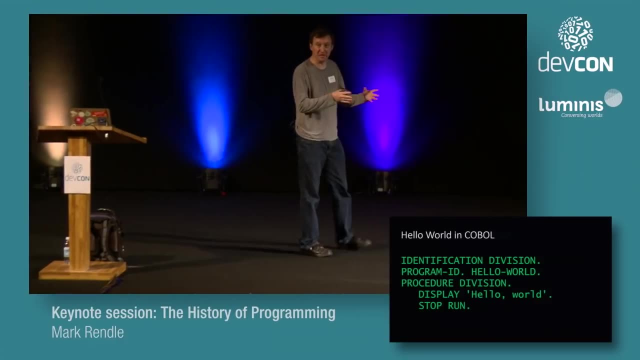 Of course, Hello, IBM, IBM. well, they couldn't just use normal COBOL and IBM. Remember speed coding, the minimum number of instructions. That was like a 1950s IBM target, a goal for their programming language. 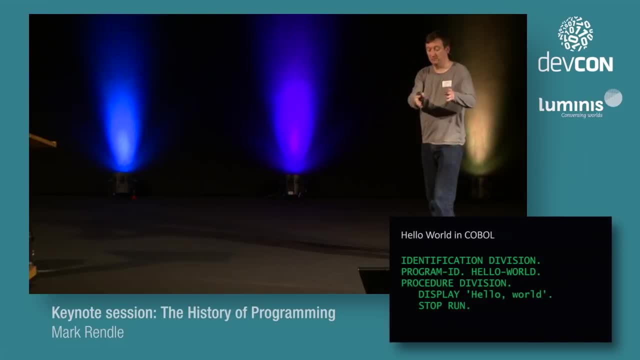 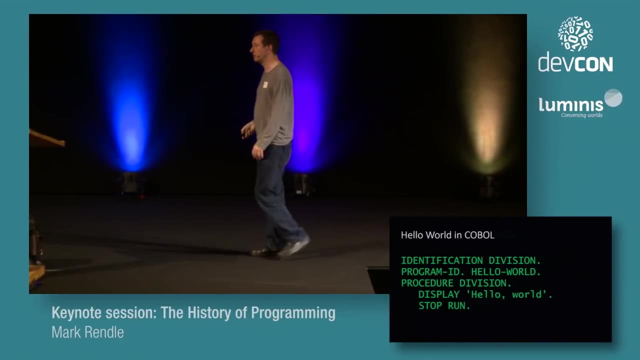 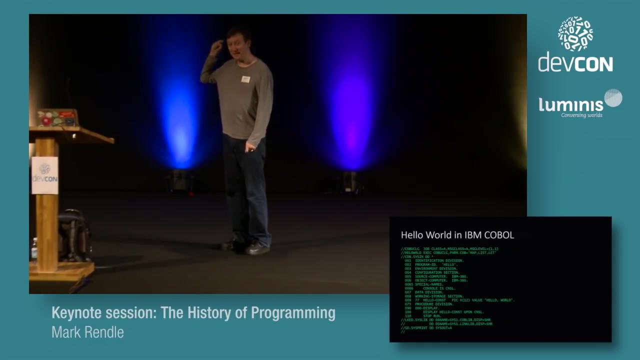 Apparently, for IBM COBOL, as defined by Codasil, was not explicit enough about the intentions of the programmer and it needed more detail. So here is Hello World in IBM COBOL. I am not lying. That's the minimum necessary. 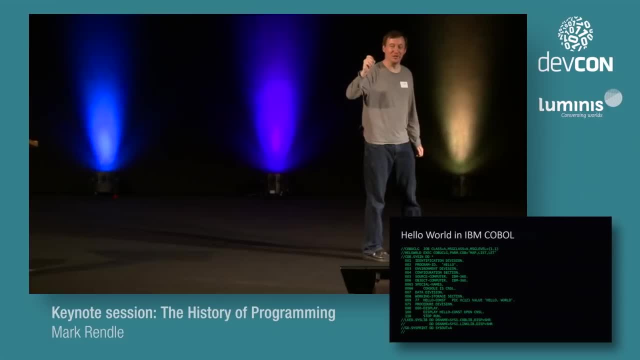 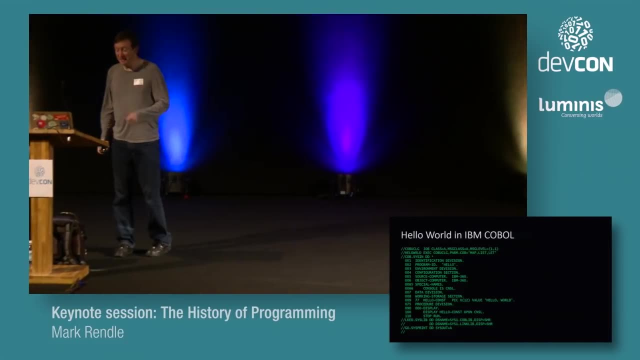 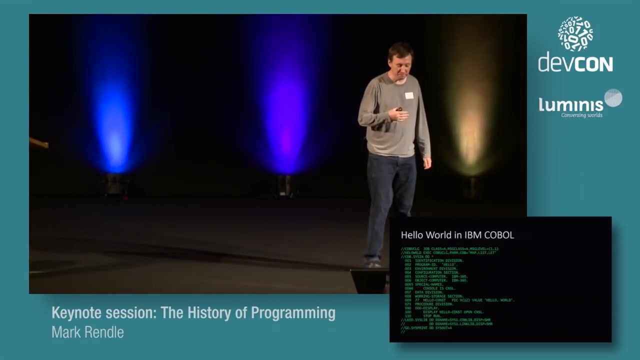 to get Hello World on the screen in the first-ever IBM COBOL. Can you say boilerplate? Yeah, So that was the 1950s. IBM rounded out the 1950s in spectacular style with essentially this thing that was just going to punish programmers. 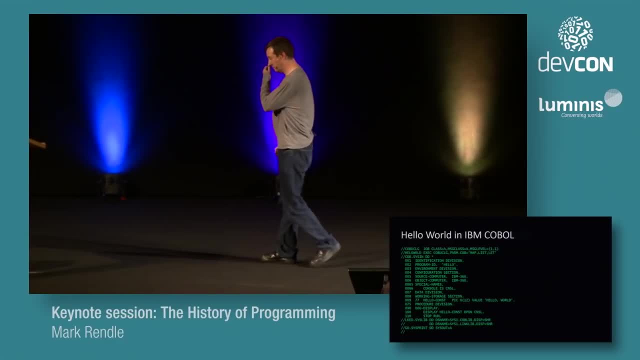 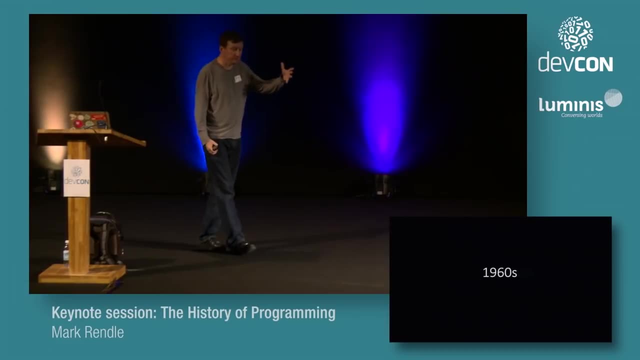 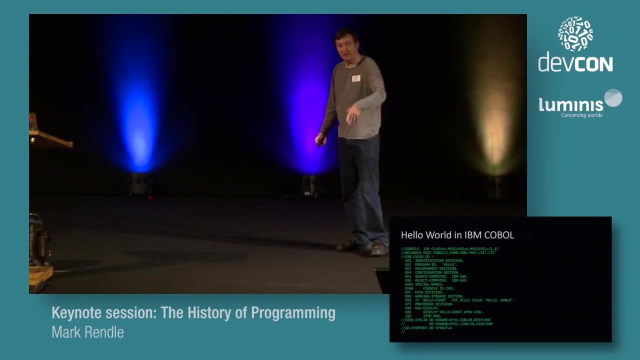 for the next 20 years, But then the 60s started and the 1960s brought a really useful advance. All of these languages that we're talking about here- Lisp and COBOL, and all this sort of stuff. we were still kind of writing the code. 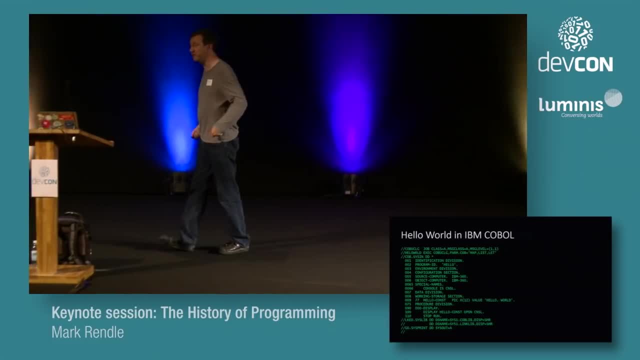 with a pencil and encoding it onto punch cards and feeding it into machines. And then in the 1960s someone went: I've got a really good idea. You know all those teletype machines we've been using just to send messages. 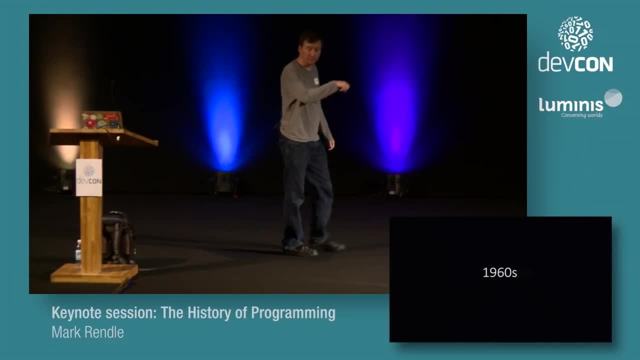 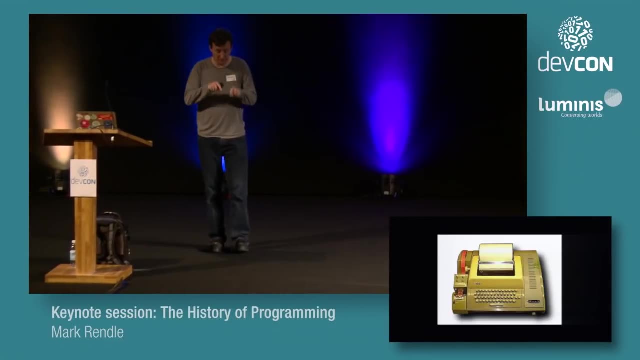 backwards and forwards between news agencies and governments and things. We could get those to talk to the computers, surely? And so people started actually being able to type letters directly into a machine and then hit enter and it would send that line of letters to the computer. 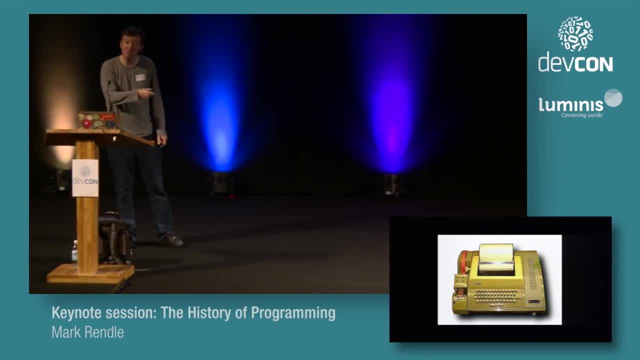 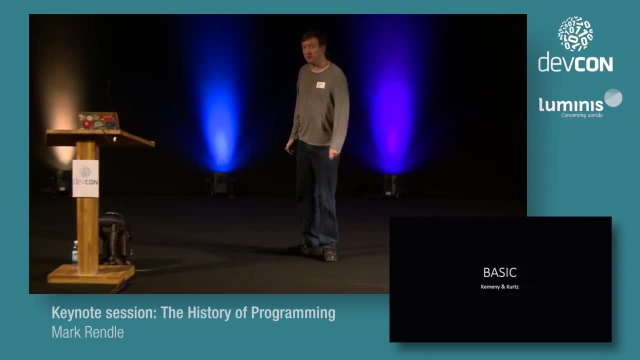 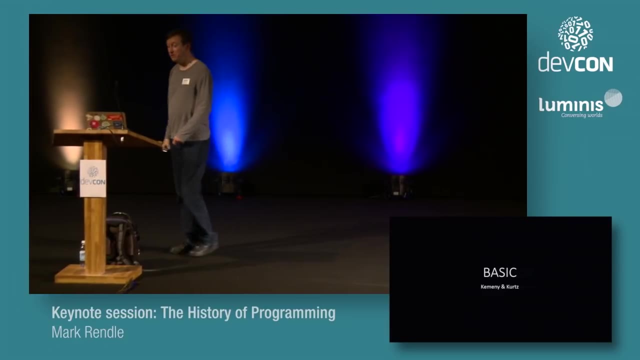 And that meant that you could start creating some simpler programming languages, more accessible programming languages, And so promptly, Kemeny and Kurtz created BASIC, Whose first programming language was BASIC. Yes, I'm not going to knock BASIC, BASIC, you know, it's brilliant. 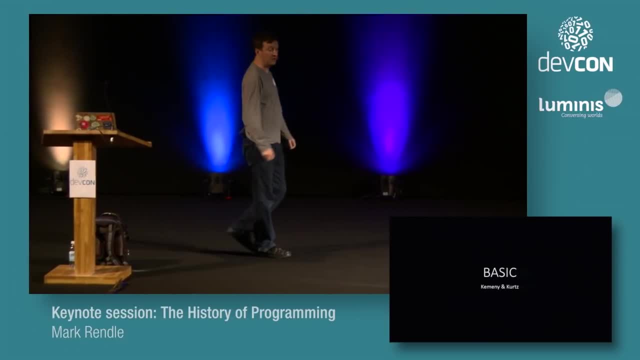 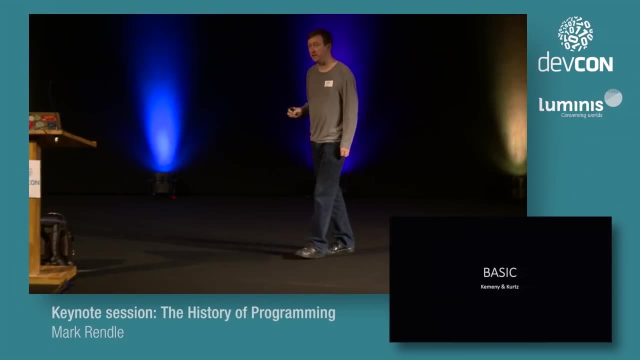 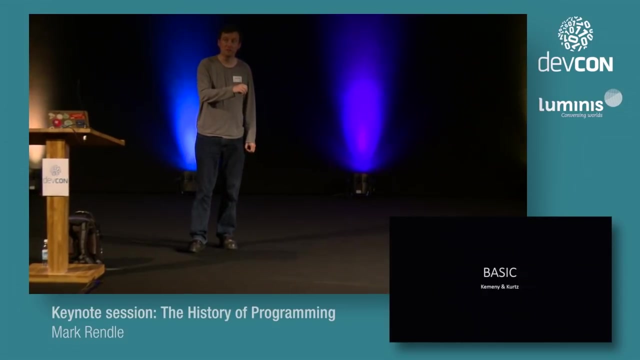 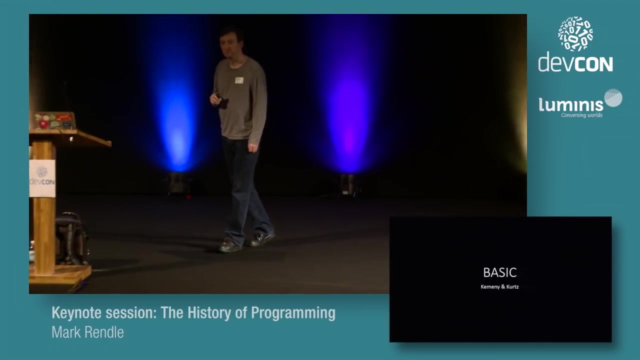 Beginners. all-purpose symbolic instruction code. The only thing that I will point out is that the B in BASIC stands for beginners And the B in VB stands for BASIC, And so the B in VB stands for beginners. Yeah, C sharp. 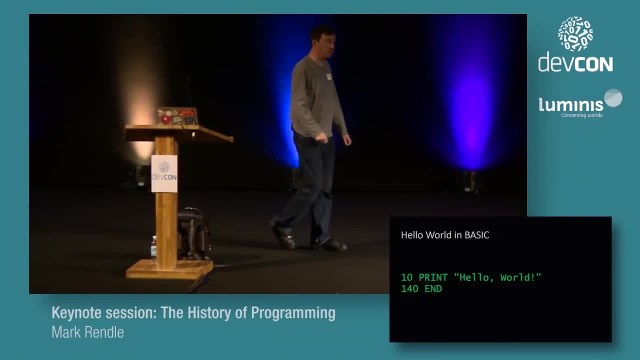 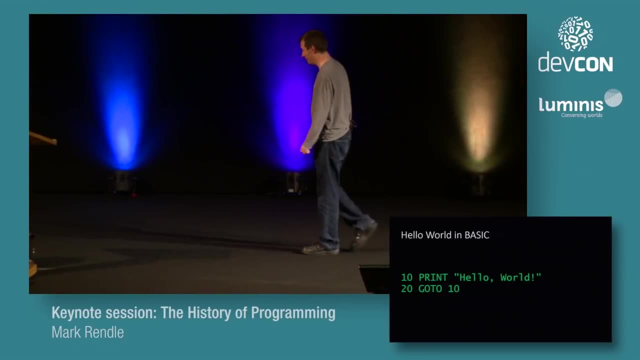 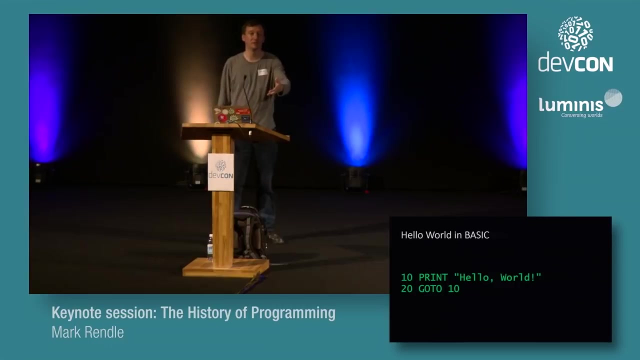 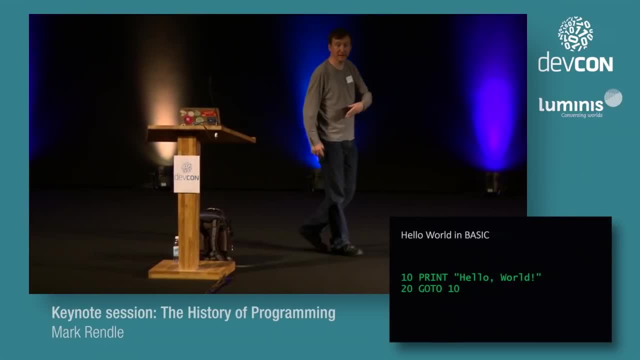 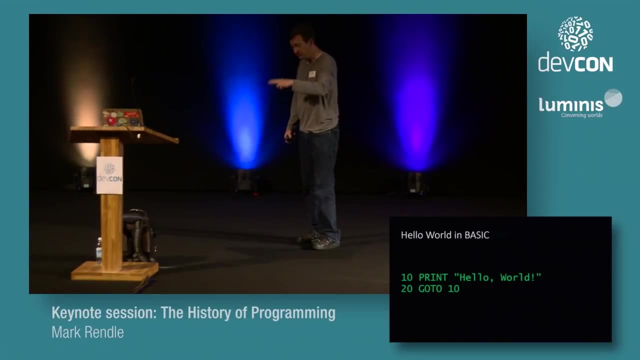 for teaching programming And it had GoTo. It also had GoSub And I remember kind of going what the hell is GoSub for? And it was. you know you go to this line number and then do some stuff and then return to the line number. 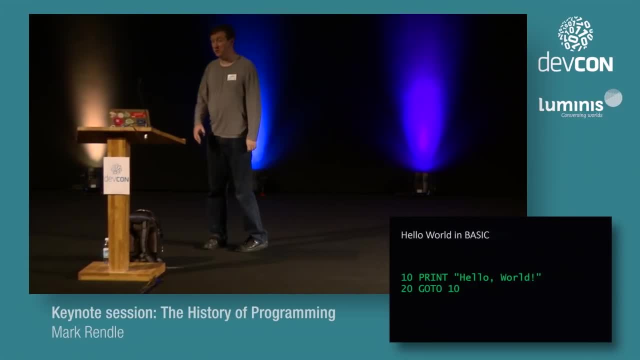 after the one that you went to this one for, And it was slightly confusing. Makes much more sense when you express it as functions. But yeah, a generation of developers learned to program, starting with BASIC. However, not everyone thought that the way to teach programming. 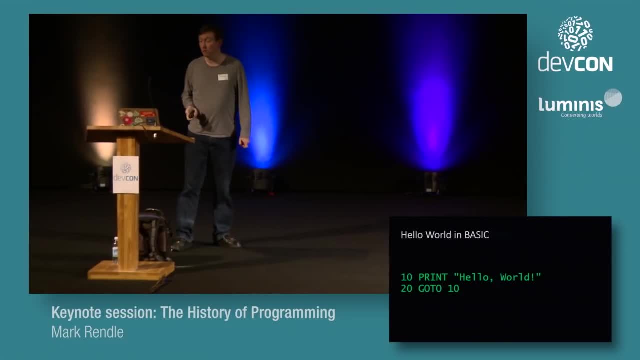 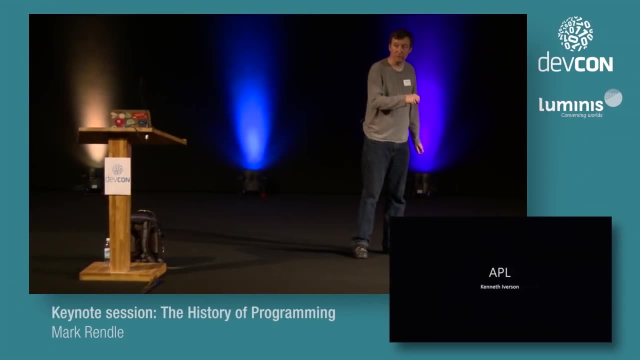 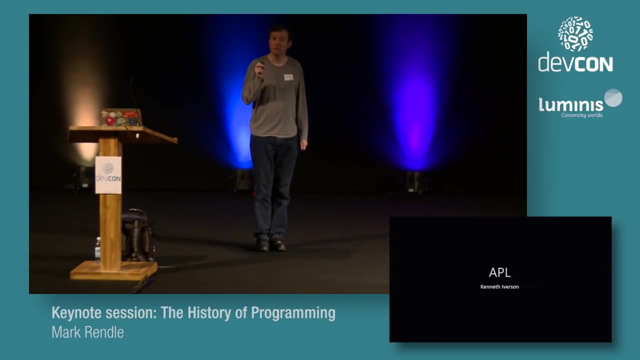 was to make it nice and simple with big, friendly keywords, And so Kenneth Iverson created APL to teach programming in his programming course at Stanford, I think, And APL stands for a programming language, Because basically, by the time he came to naming it, 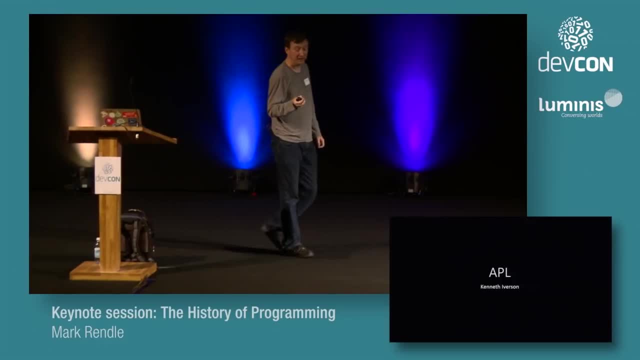 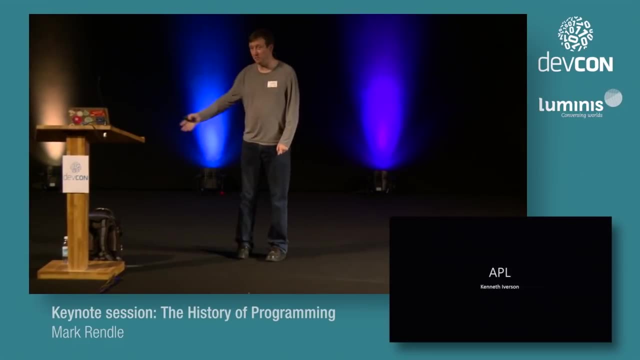 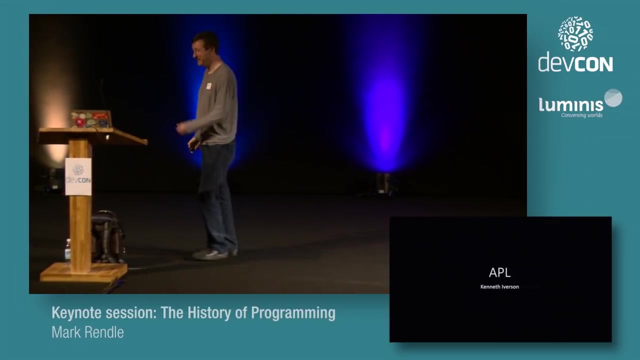 Kenneth Iverson had used up all his creativity. Kenneth, hey, these are your children. Yes, this is A-boy and A-girl. What are their names? A-boy, This is Hello World in APL. Anything that you just put in quotes. 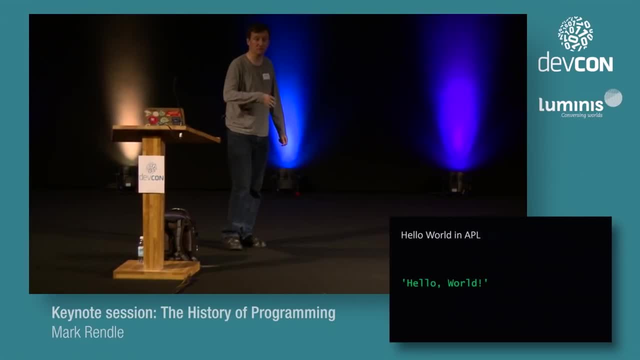 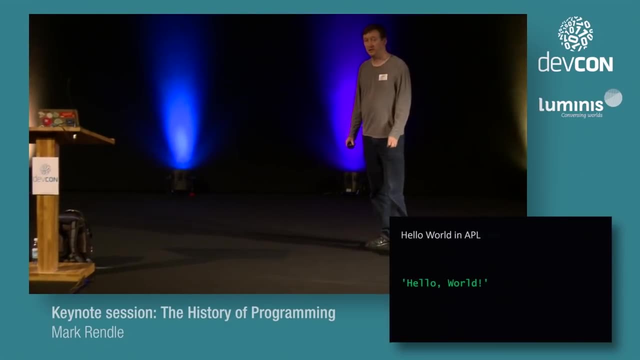 you probably want me to write that out, don't you? Yeah, I'll just write that standard out, That's not a problem. You might look at that and think APL is quite clearly a very succinct and intelligible and sensible programming language. 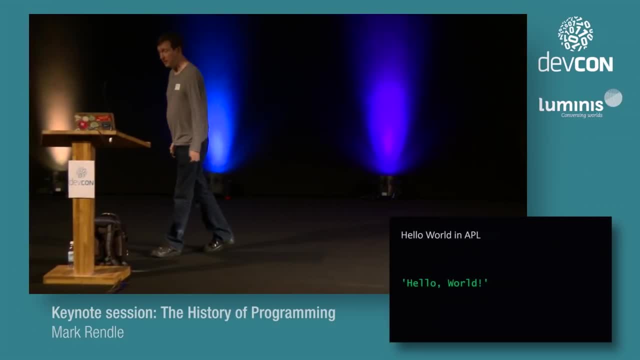 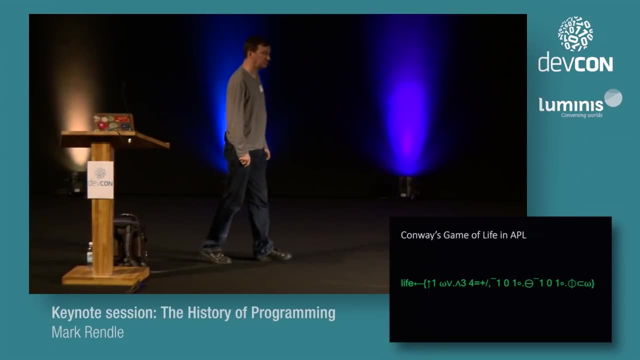 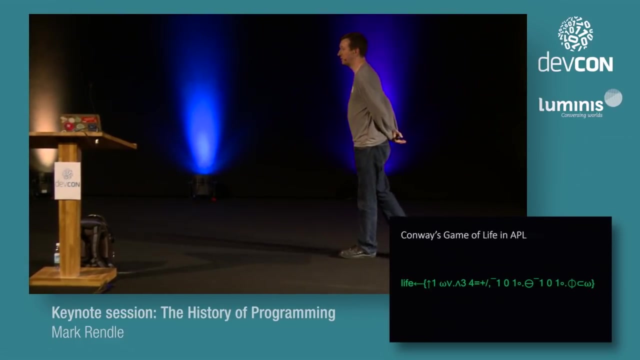 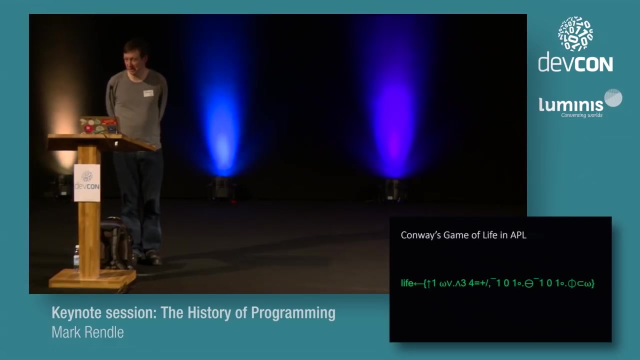 And if that's true, you've never actually seen any real APL code. Here is Conway's game of life in APL. Now you may notice a couple of unusual things about APL. Not all of those characters are on your keyboard. 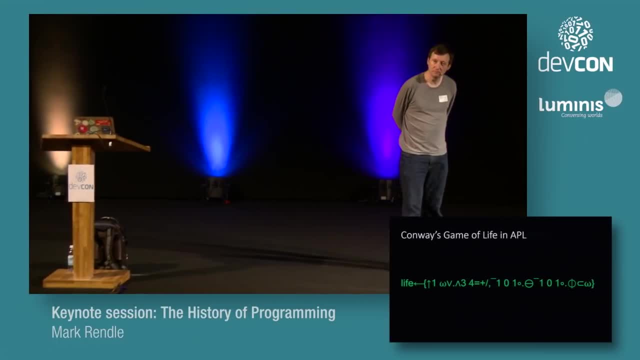 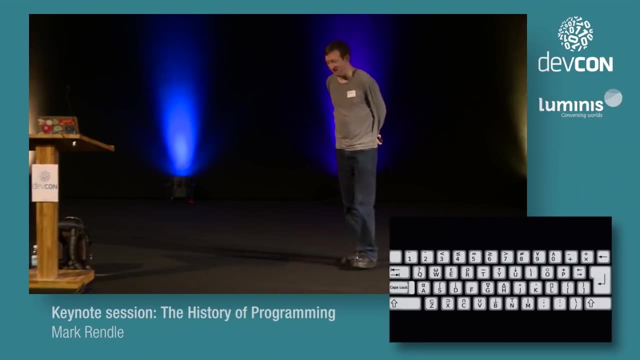 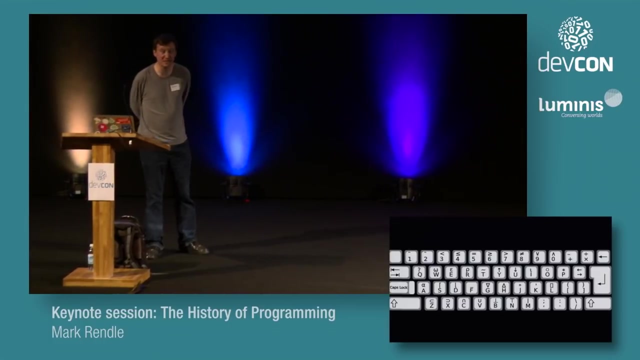 This did not deter Kenneth Iverson. He just made a keyboard that did have those characters on it. I swear to God, this is true. This is an APL keyboard If you wanted to write APL. there are people today still doing APL. 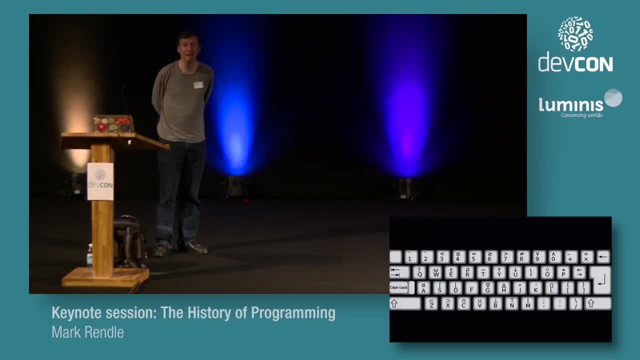 Anyone in the room do APL for a living, Even a little bit? Are there people who do APL in your business? If you go into the financial sector, where you've got these people who are trying to kind of trade shares in tenths of a nanosecond? 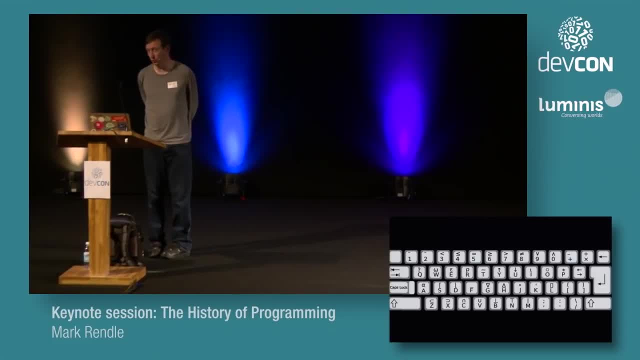 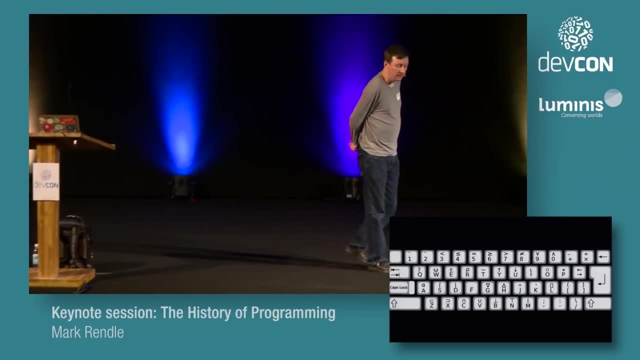 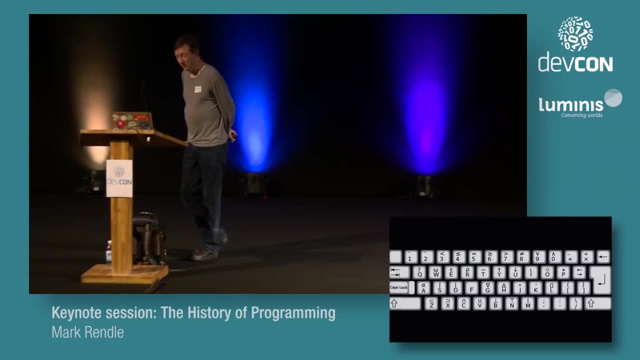 to try and scrape off the .0001 of a cent. they use programming languages like Fortran and APL And yeah, it's very, very powerful, But yeah, but it's also just weird. I kind of like it. 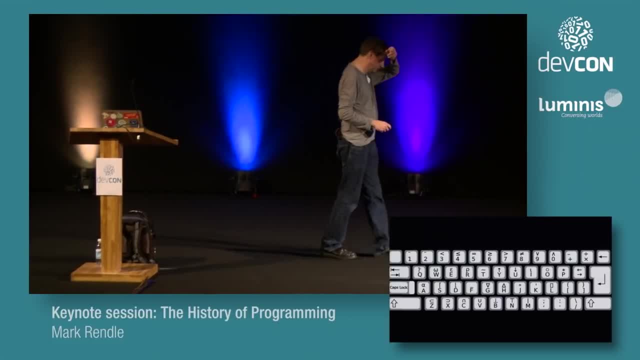 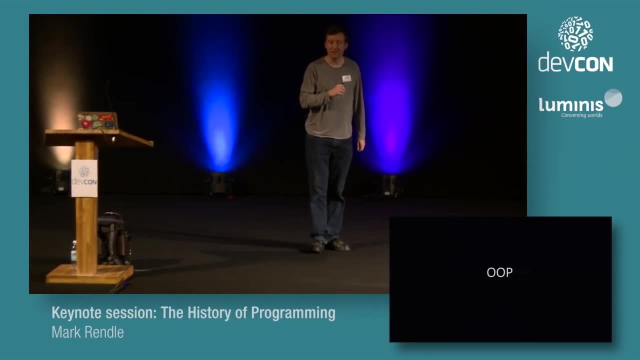 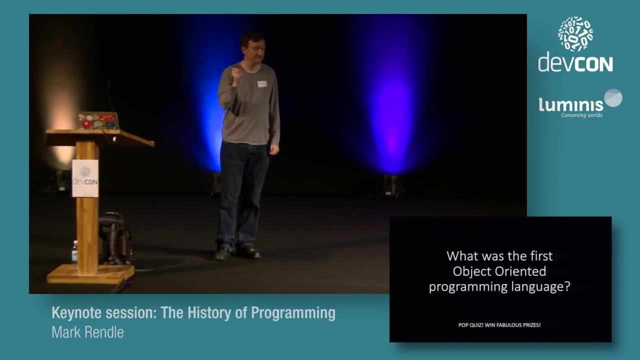 So, yes, okay. Also in the 1960s, on a slightly more sensible note than Kenneth Iverson and his APL, object-oriented programming was invented. So pop quiz, What was the first object-oriented programming language? See everyone, ooh. 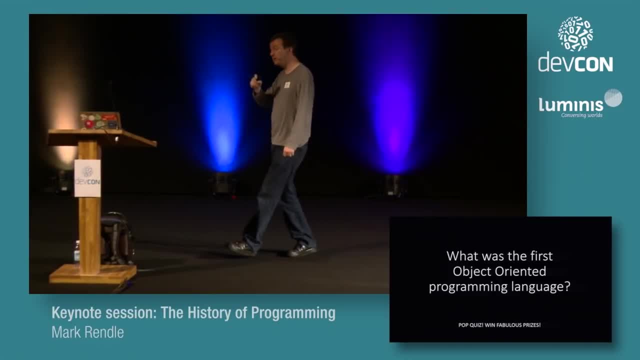 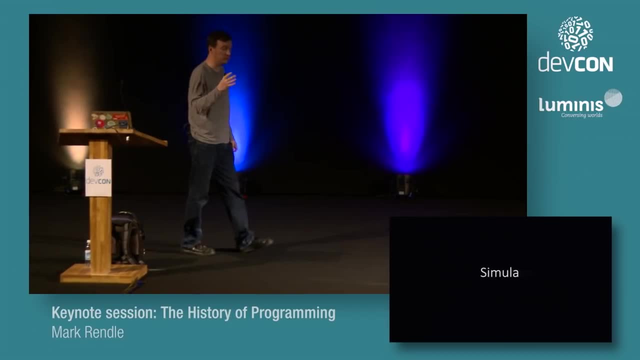 Simula. yes, Not Smalltalk. Foolish people who said Smalltalk, It was Simula. See, Simula was the first object-oriented programming language and it came out in the late 67.. I really should put notes on my slides. 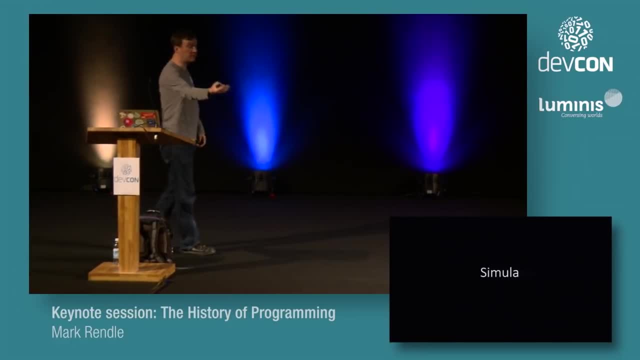 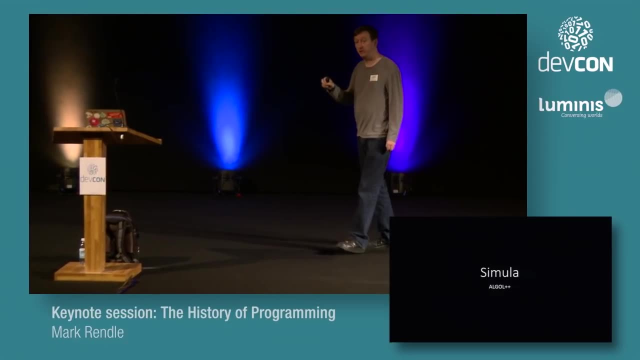 so I can look cleverer than this. But yes, Simula was the first object-oriented programming language. Simula would have been called ALGOL++ if ALGOL had had the plus-plus operator. But it didn't, And so 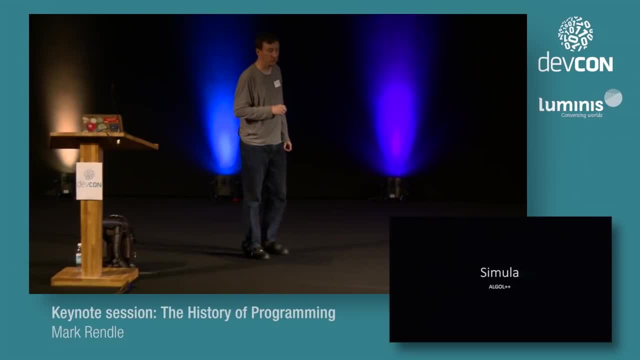 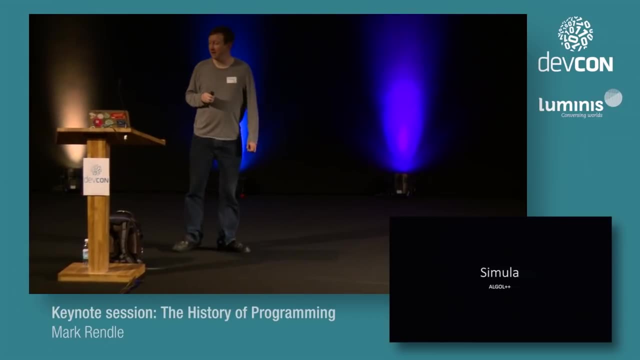 that would not have been a good joke in the way that C++ was such a good joke If they'd called it ALGOL++. people would just have gone what? But yes, here's hello world in Simula And typically of object-oriented programming. 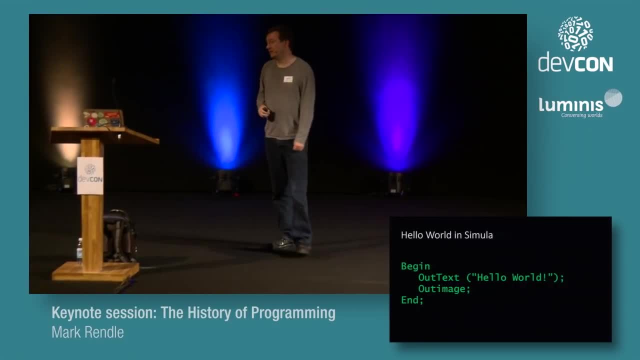 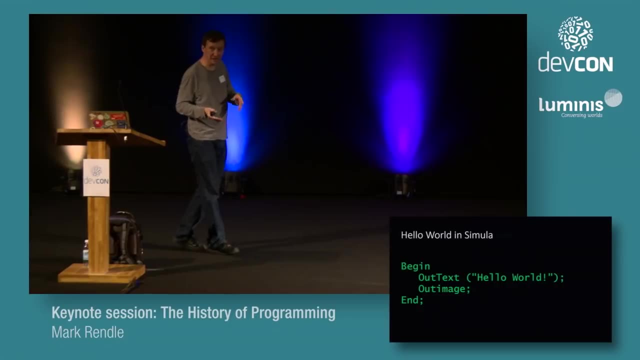 all it's done is made it longer and more complicated. So yes, So Simula was being used in kind of proper programming and APL was being used in kind of proper programming, and BASIC was being used by people who could afford keyboards. 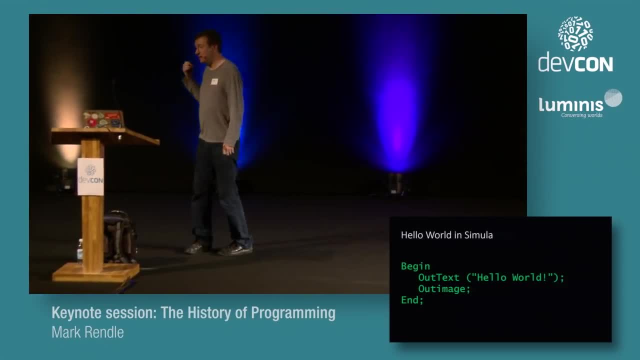 and BASIC was being used to teach stuff, But BASIC was still quite complicated. You could do lots of things with BASIC and people wanted a simpler programming language because by the end of the 60s quite a lot of students were tired. let's say 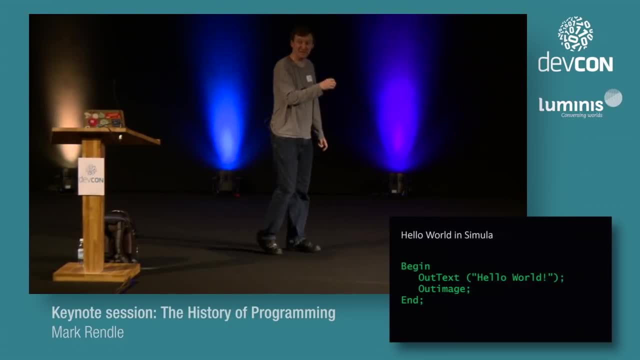 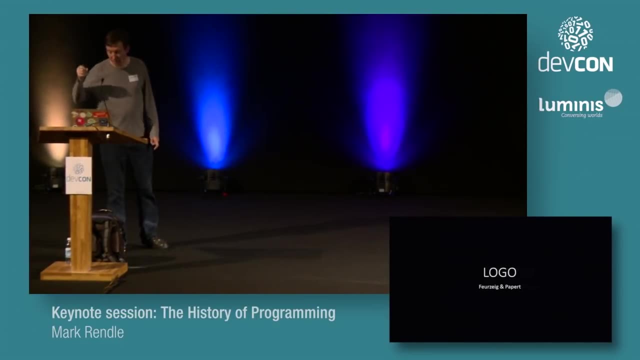 not really with it all the time, And so people thought we need to make a simpler programming language for the modern university student, And so Furzeig and Papert created Logo. I did some Logo at school. If you do Logo now, it's a bit boring. 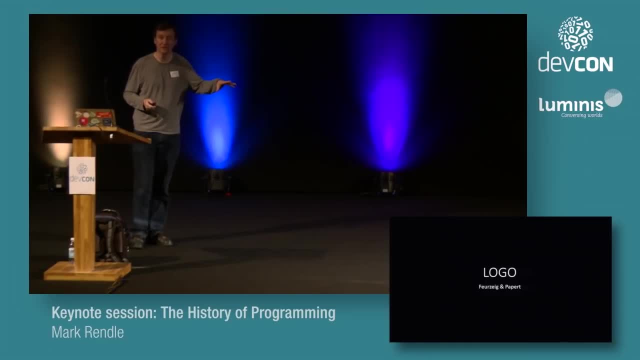 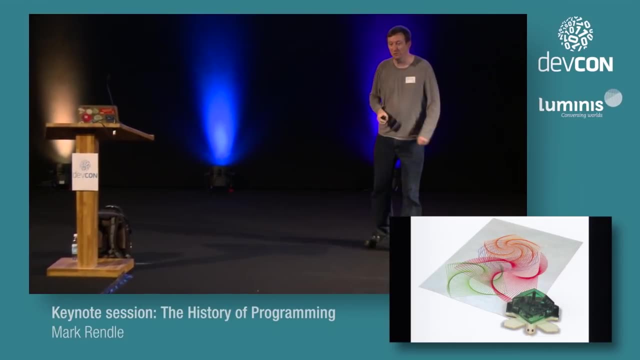 because they tend not to have the actual output device that you're supposed to have for Logo, which was this: That's a Logo turtle, and you would write the instructions in Logo and then set it going, and the turtle would just crawl around on a piece of paper. 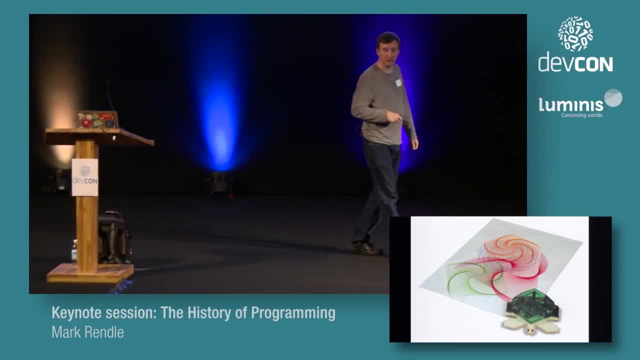 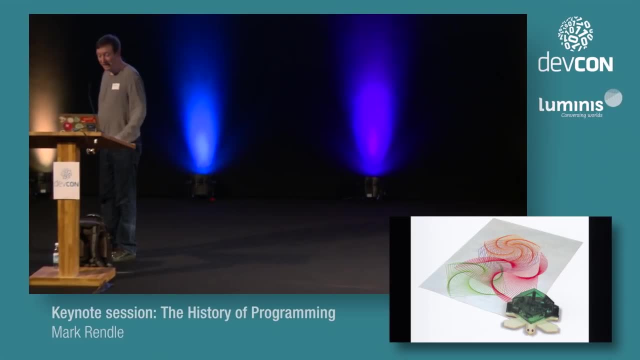 and your teacher would say: right, and when you come back tomorrow you can see the results of your thing And you're going. yes, it's just like IBM, But yes, I think it's telling that this programming language, with this particular set of features, 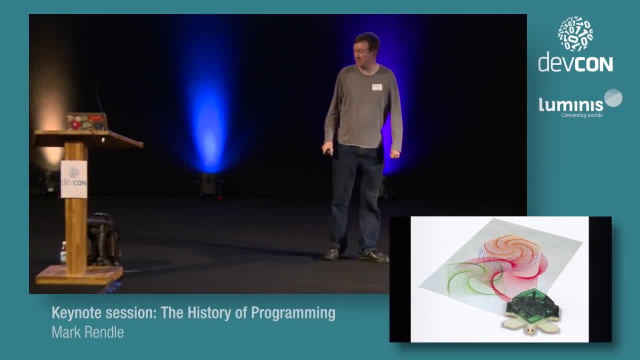 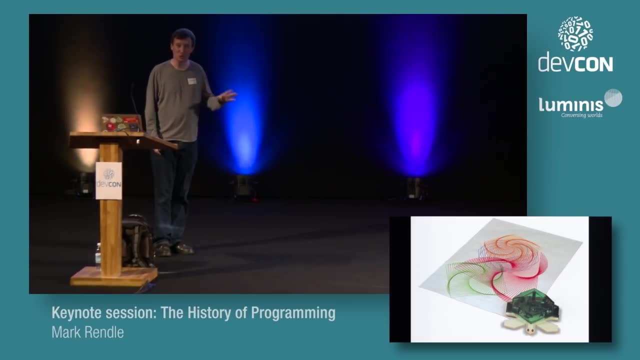 was created in American universities at the end of the 1960s And then the 1970s started and, quite frankly, it's all just been downhill The 1970s. so we got teletypes at the start of the 1960s. 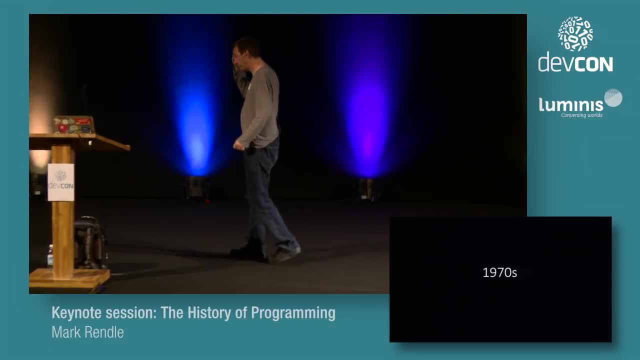 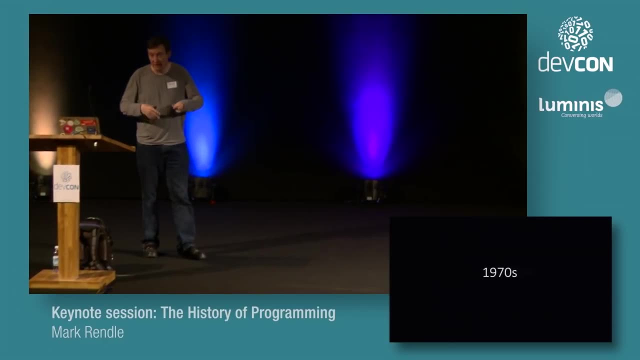 and those made our lives an awful lot easier. But it was still this thing: You'd type it in and it would go onto the paper and then you'd press Enter and it would send that to the machine, And then, after a while, 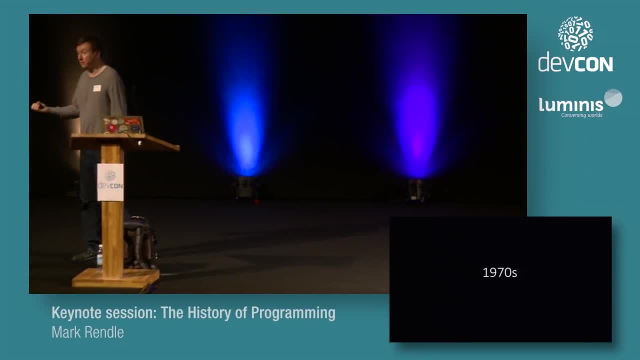 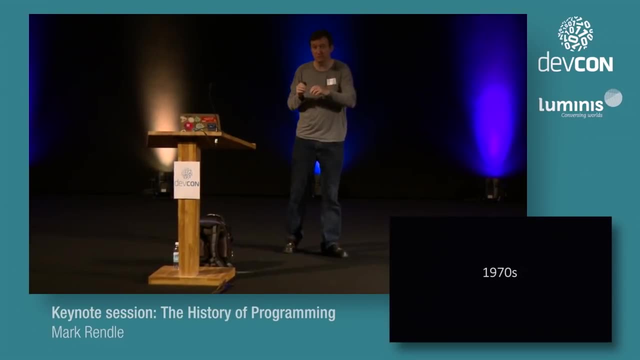 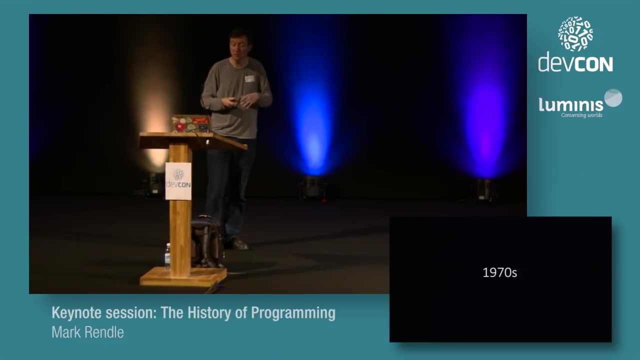 the thing would print out some more lines like this. And then someone else worked out that with the same set of electronics and stuff- that was the signals that were going backwards and forwards- you could actually replace the paper with just a cathode ray tube. 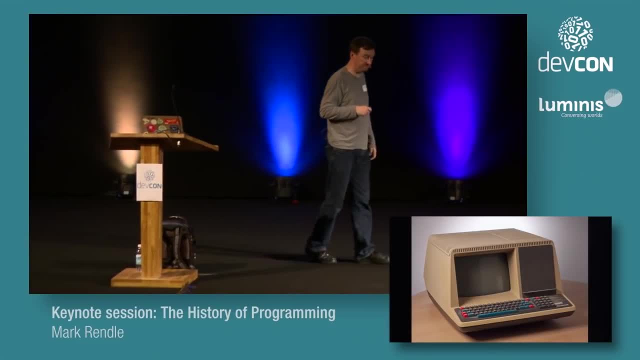 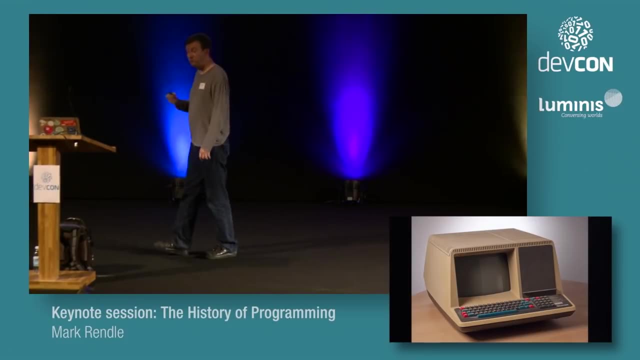 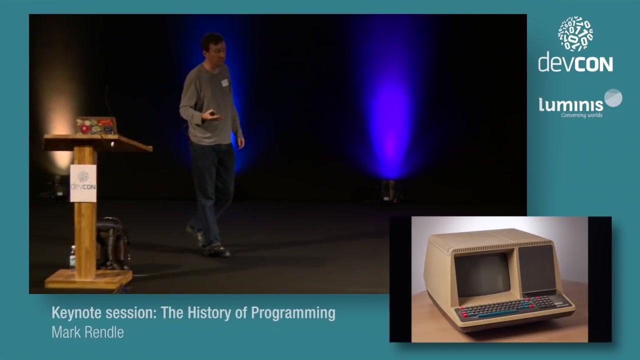 and they created the visual terminal, And so now, finally, we had a screen that you could type into, which was great. The brilliant thing, though, about the teletype terminals and the systems they were used with at the time was, you would think this would now mean. 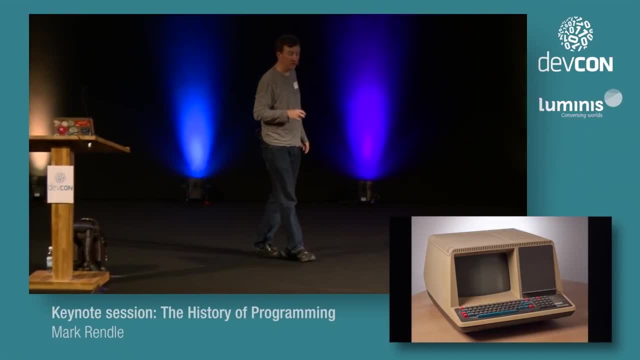 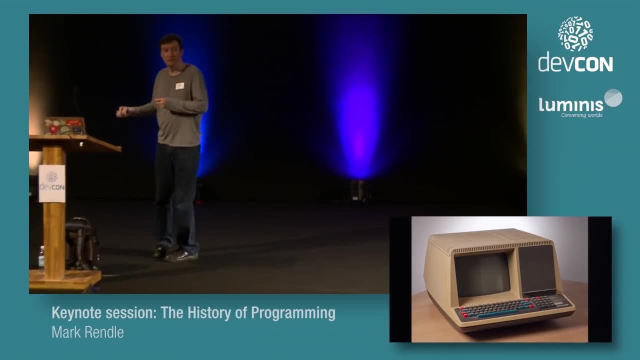 that you could kind of launch your editor and jump around the code and do all this sort of stuff. but all they were was a CRT pretending to be a piece of paper, And so you still had this thing where you were typing a line at a time. 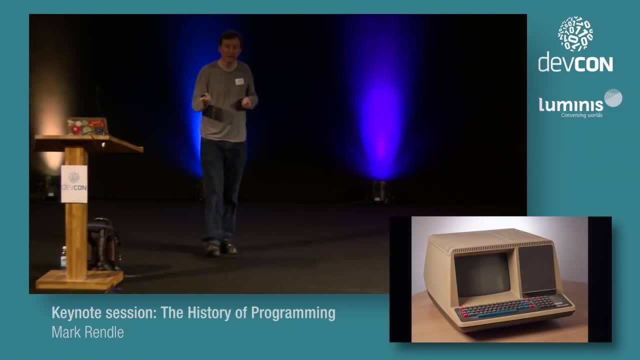 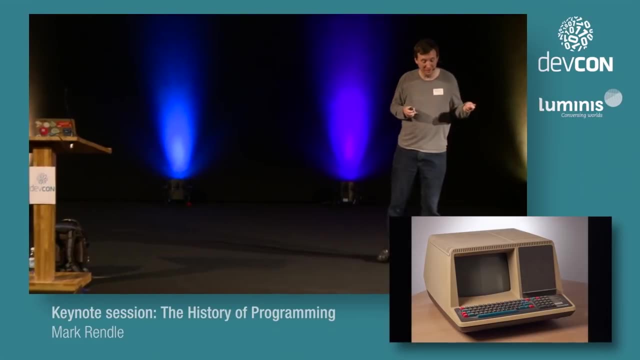 and sending that to the computer and getting a line back. Has anyone used Edlin? Yeah, yeah, From the people who created Microsoft Word in the end. But, yes, Edlin, In Edlin you say: show me line 20,. 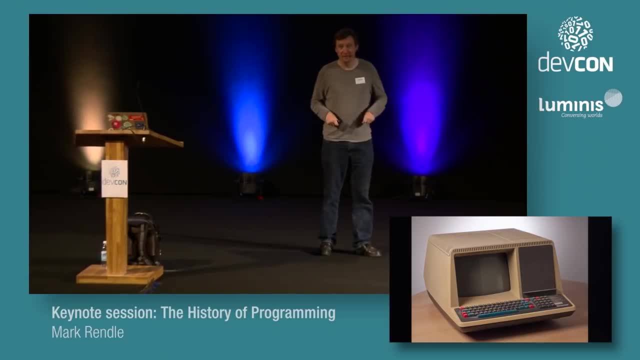 and it shows you line 20.. And then you go: I'm going to change line 20.. Now send line 20.. I've sent line 20.. Now show me line 21.. We used to write code like that. It was brilliant. 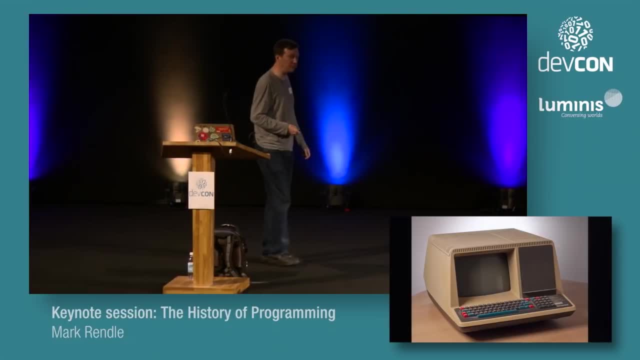 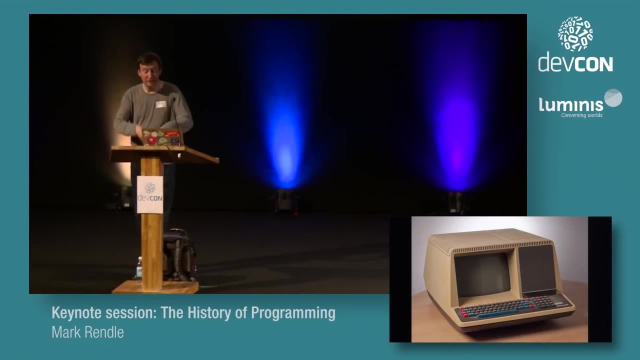 It wasn't. It was awful, But for the people here under the age of whatever I am, you don't know you're born. So yes, But this made it slightly easier to write your basic code, And actually basic was very well suited to this. 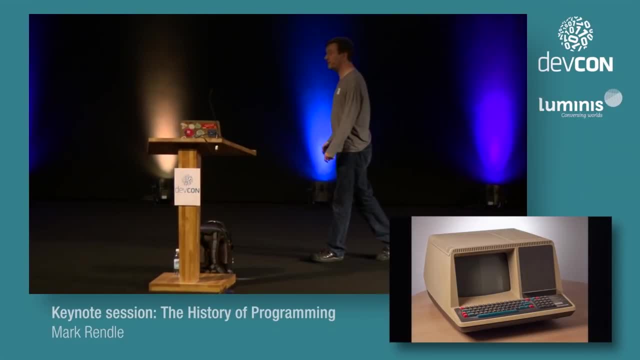 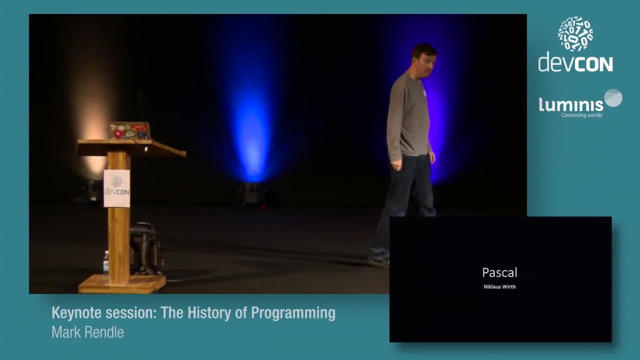 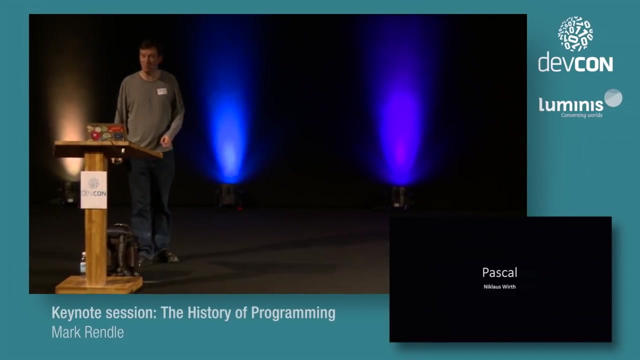 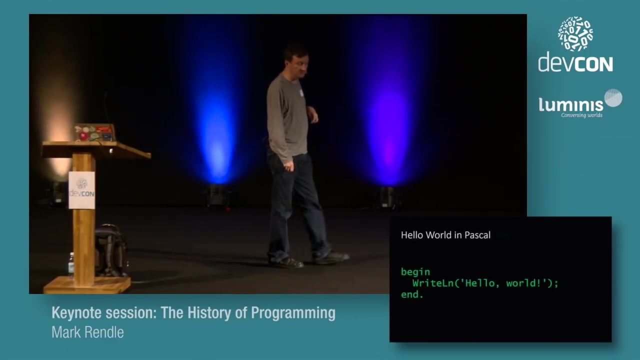 because it had line numbers, And so we started to get more people interested in programming and more programming courses at university. And we got another training language, Pascal, by Niklaus Werdt, And Pascal was really just somewhere between our goal and basic. And here's hello world in Pascal. 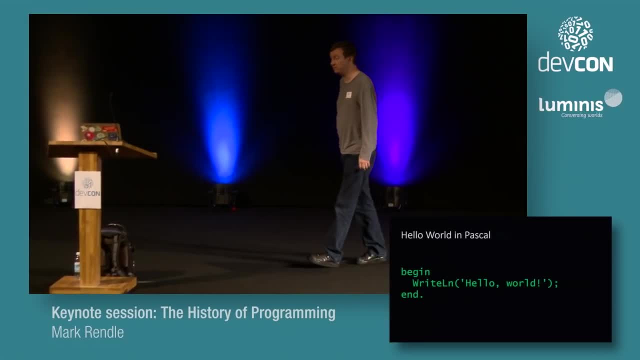 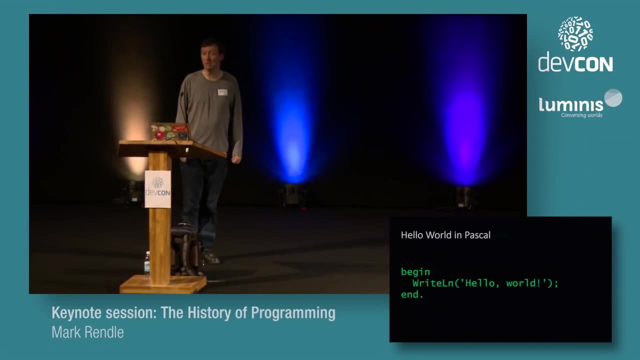 And yeah, there's nothing wrong with Pascal. It's led to some brilliant things And I'm not going to say anything mean about it. No, I am. It's shit. It's an awful language And just begin and end and full stops and semicolons. 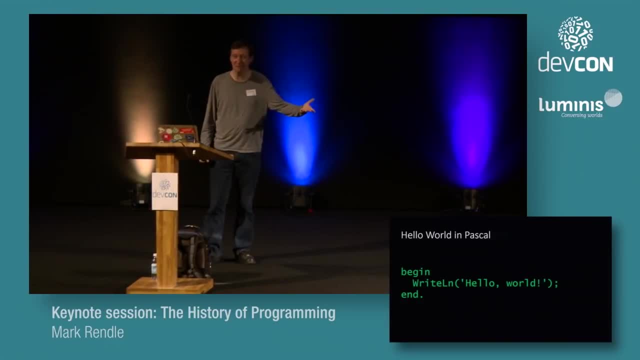 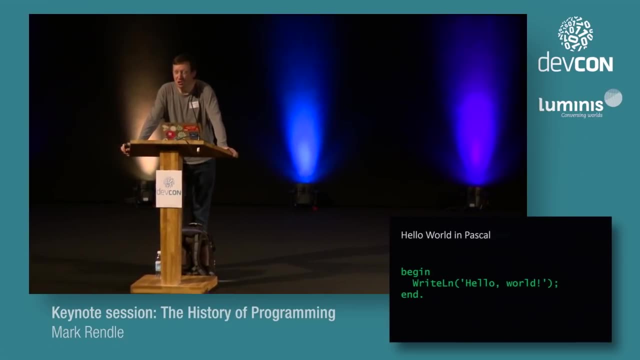 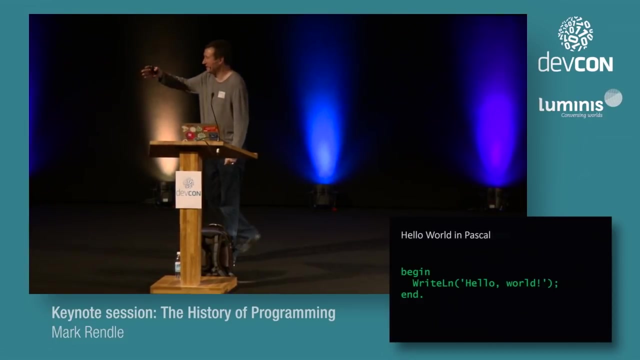 It's kind of everything that's good about C and everything that's bad about basic all crammed together into one godawful abomination of a language. I hated Pascal so much. I was at one college doing Pascal and my friends were at another college doing C. 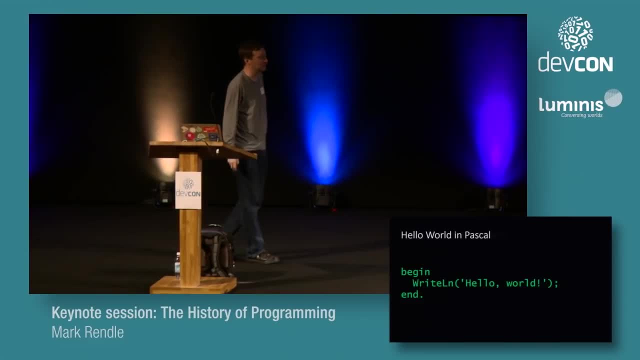 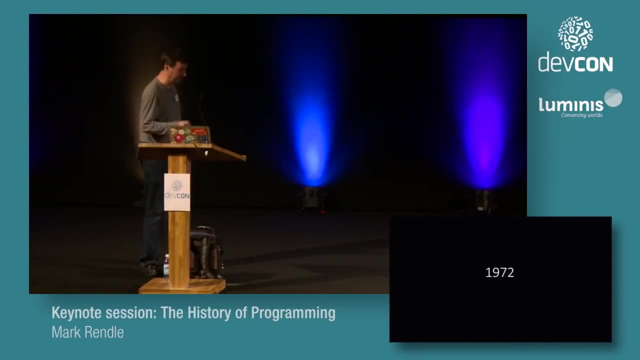 And I knew that C was actually what you needed to learn, And so I was kind of doing my homework. Not bitter I am, I'm so bitter Anyway, 1972. Smalltalk. there you go. You were six years early. 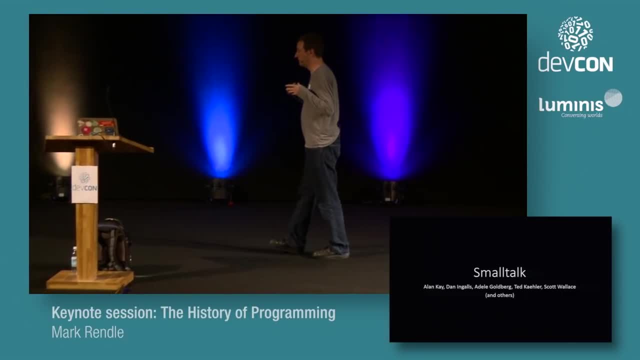 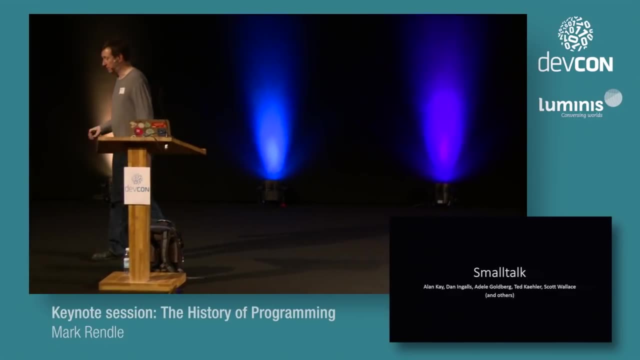 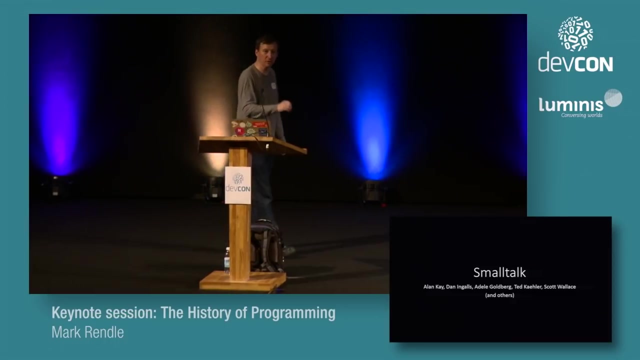 Smalltalk was created in 1972. And Smalltalk was the first kind of widely used and properly thought through object-oriented programming language. Except that what Smalltalk really was was a message-oriented programming language. The whole point of Smalltalk is that you created objects. 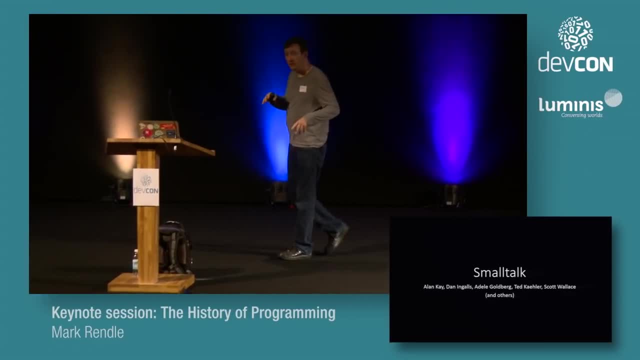 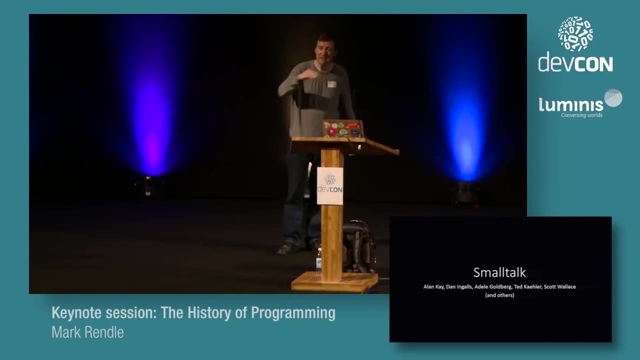 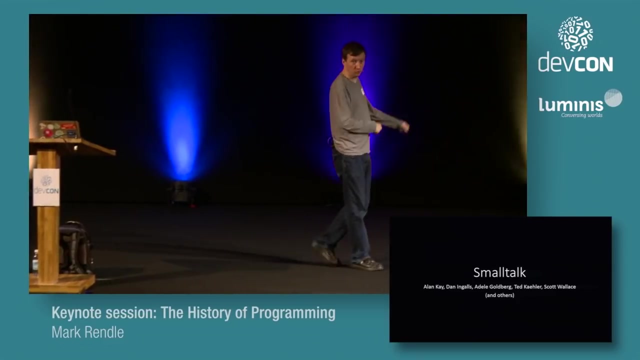 and then these objects communicated with each other using messages, And that was the key takeaway of object-oriented programming. And Smalltalk was messages between discrete components with no shared state. Unfortunately, what the world took away from Smalltalk was so animal is the base class. 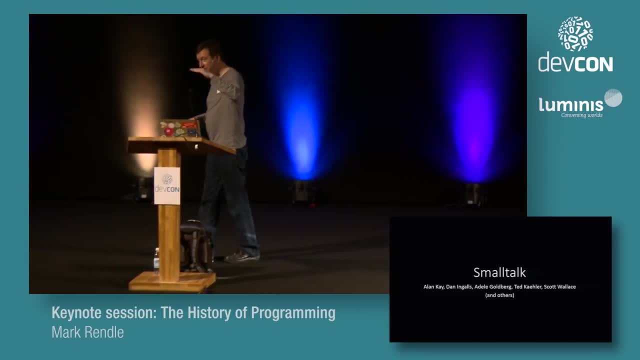 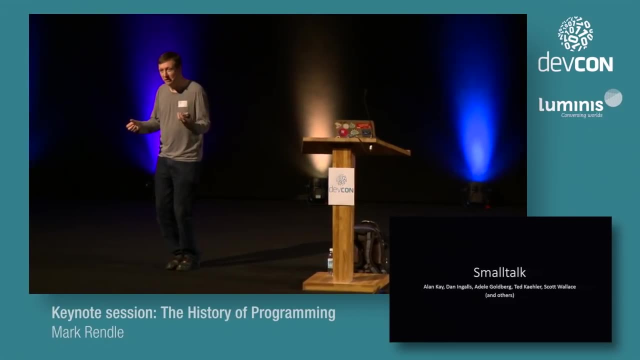 and then giraffe is a subclass of animal. Alan Kay just sits there at night by a dying fire with a bottle of brandy in one hand And a gun in the other, just going. if I just called it message-oriented programming, where would we be? 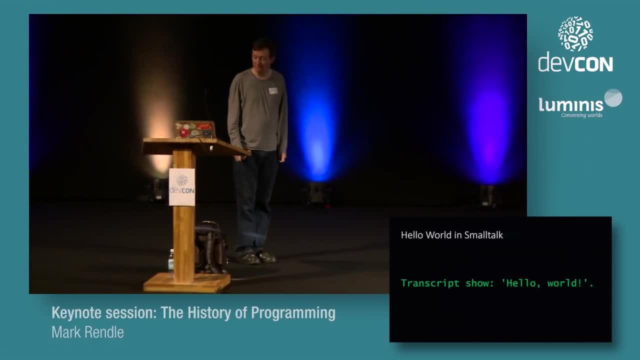 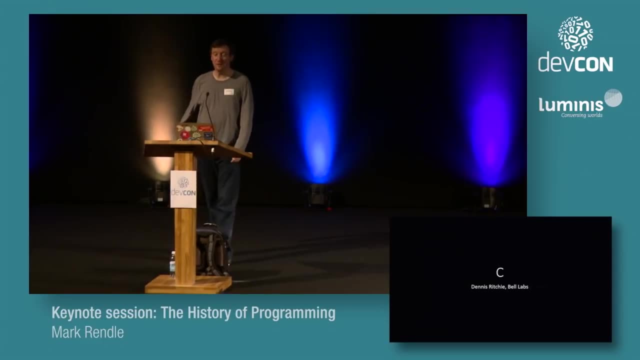 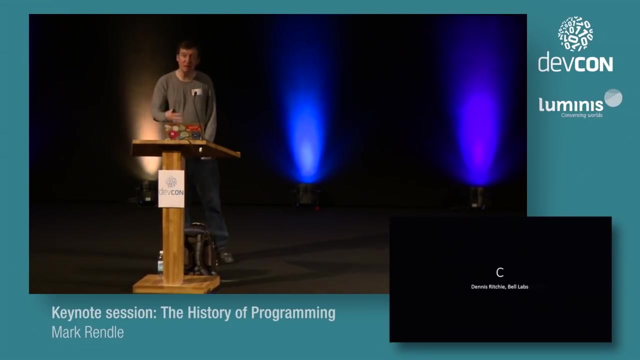 Here's Hello World in Smalltalk. That's just weird. I'm glad I don't have to write Smalltalk code. And, of course, C, created by Dennis Ritchie and various other people at Bell Labs. C was derived from B, which was derived from ALGOL. 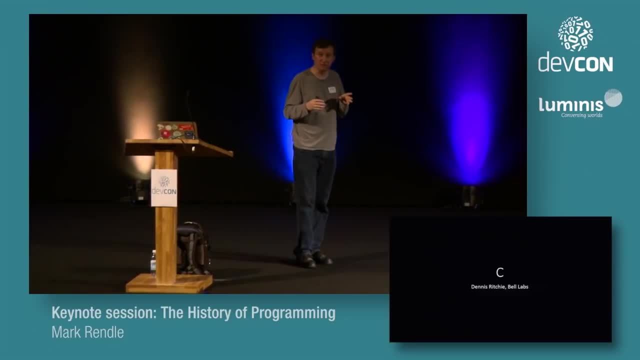 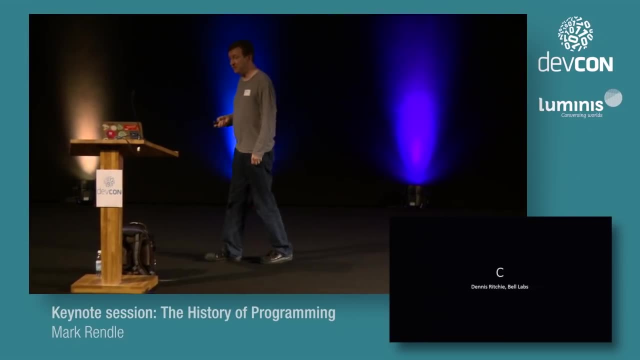 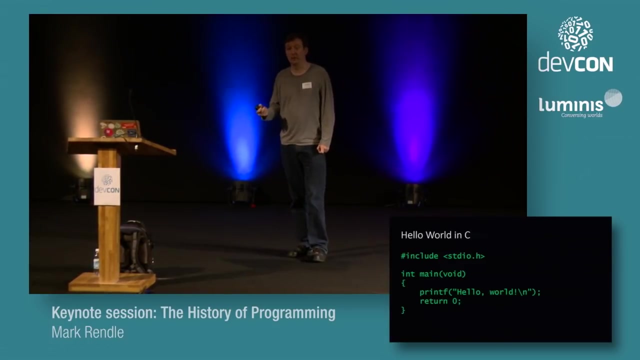 And pretty much every programming language that matters in the world today is derived in some way from C. It is the grandfather of all programming languages And this is Hello World in C. And Hello World in C is special because Hello World in C was the first actual Hello World. 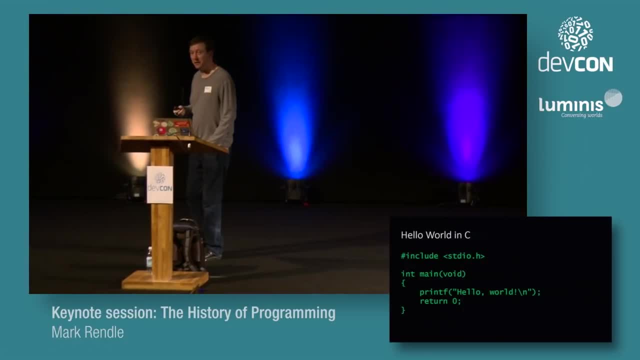 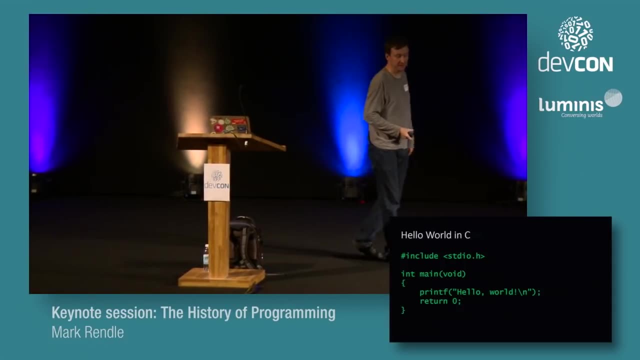 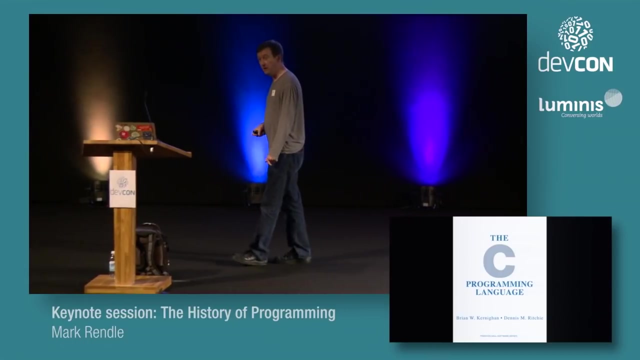 It was the first programming language where the first example of it was to print Hello World to standard output and exit. This was the first ever program you wrote in C. if you learned C from this book, If you didn't learn C from this book, 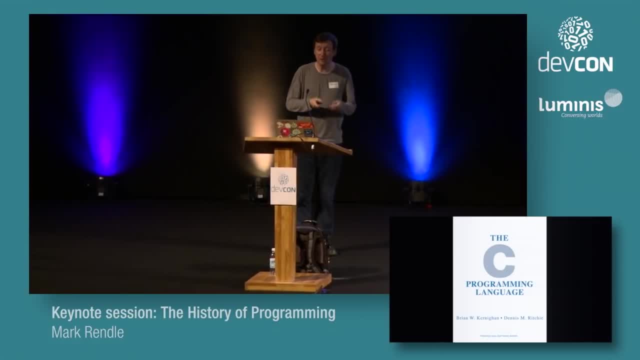 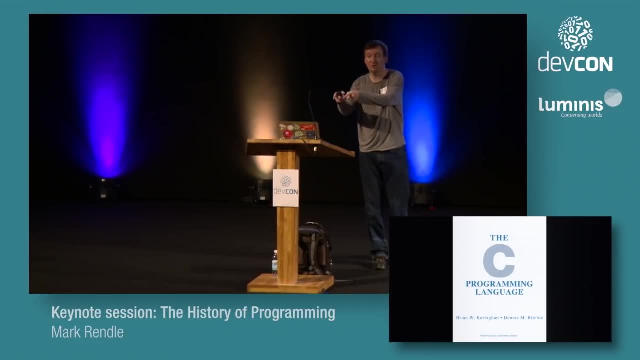 I mean never mind if you didn't learn C at all, but if you didn't learn C- not C++, but C from this book. maybe not this book, maybe the second edition, maybe the third edition, but if you didn't learn C, 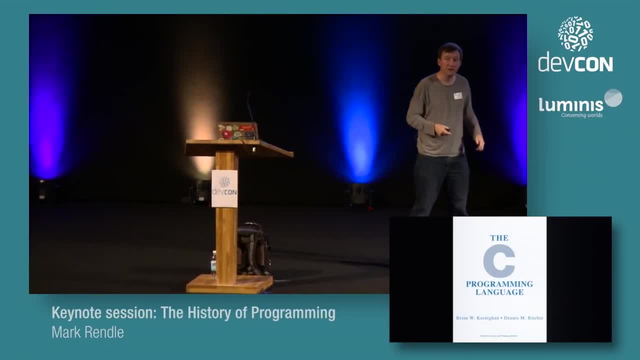 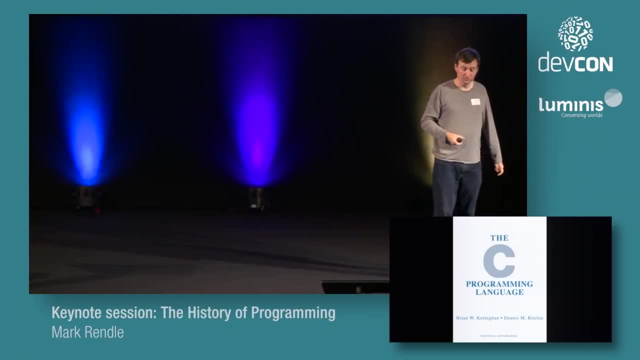 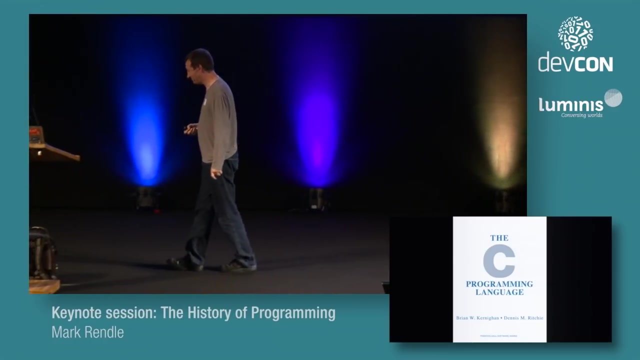 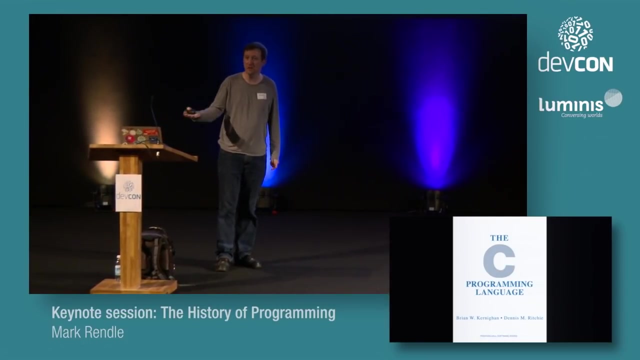 if you have at no point in your entire life learned C from this book, that book, you are not a real programmer. I do know people who actually believe that It certainly would be a useful thing if everybody did learn the fundamentals of C from that book. 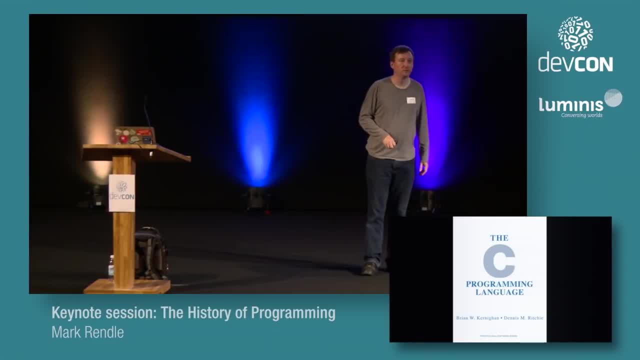 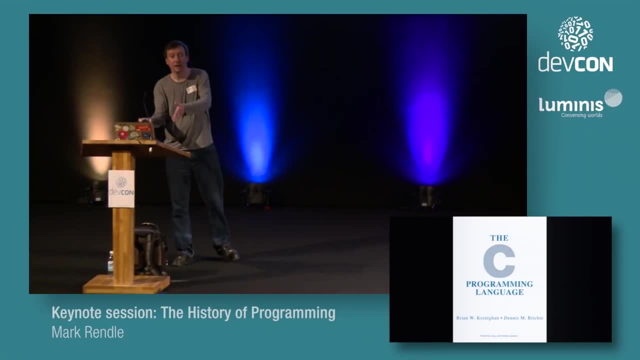 because it kind of teaches you about memory management and gives you at least a vague idea of what garbage collectors are like and what they are actually doing for you. The problem with not knowing an unmanaged language and just knowing managed languages is you don't know how lucky you are. 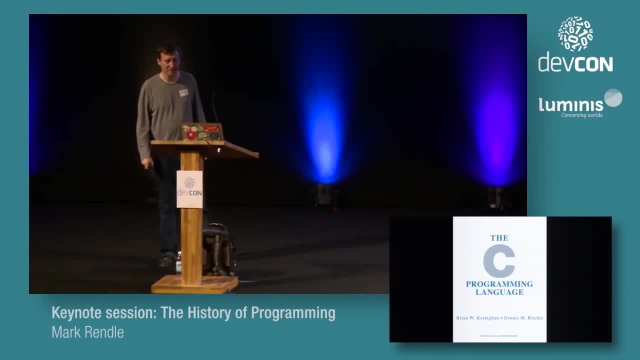 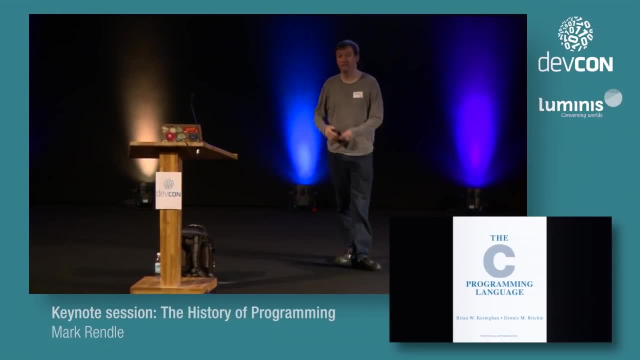 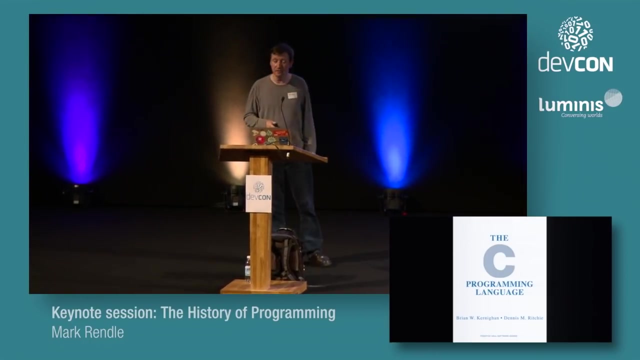 Bloody malloc and free and dealloc and God knows what else was going on. But yes, so there was C And, like I say, C was the grandfather of all modern programming languages, which of course meant that there were some evolutionary dead ends in the 1970s as well. 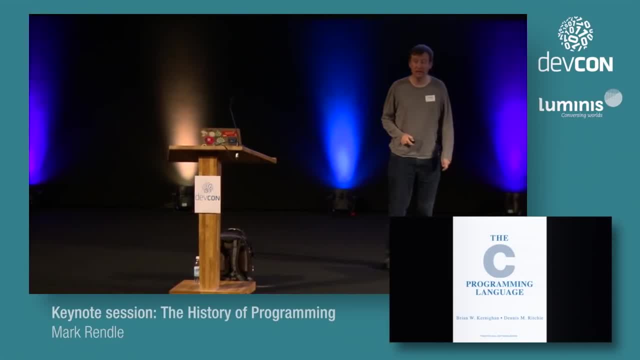 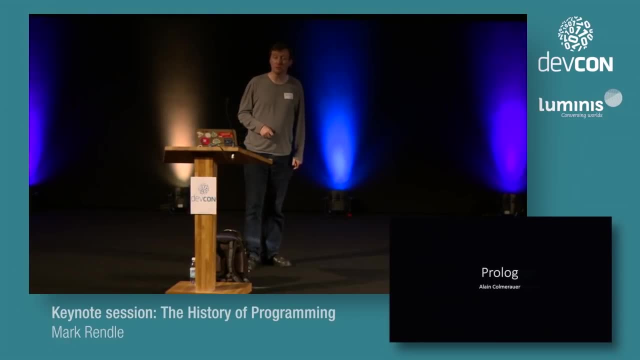 because if you were creating a programming language and it wasn't C, then yeah, good luck with that. So a good example of that: Prolog. There are still people who use Prolog, but in America there are still people who ride around in horse and carts. 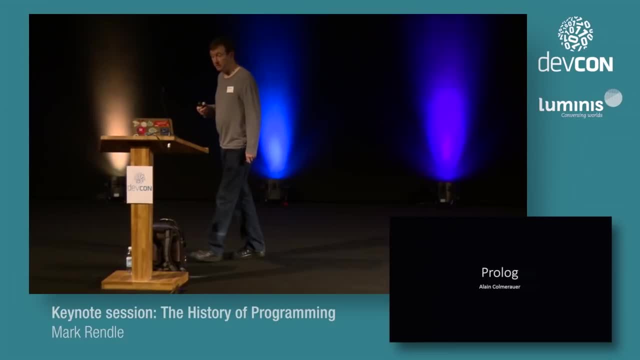 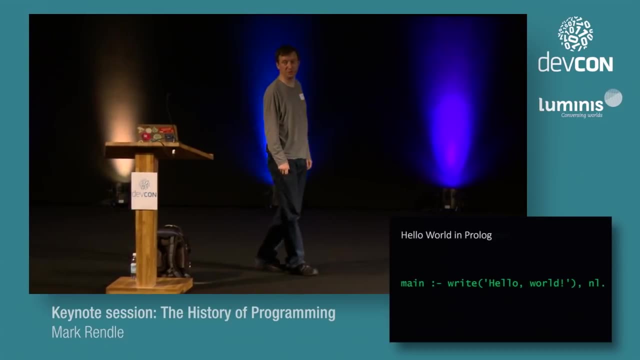 and put up barns with their hands and don't believe in watching television or modern medicine. But yes, Prolog was great. Here's Hello World in Prolog, which, of course, is not what Prolog is for: It's for building expert systems. 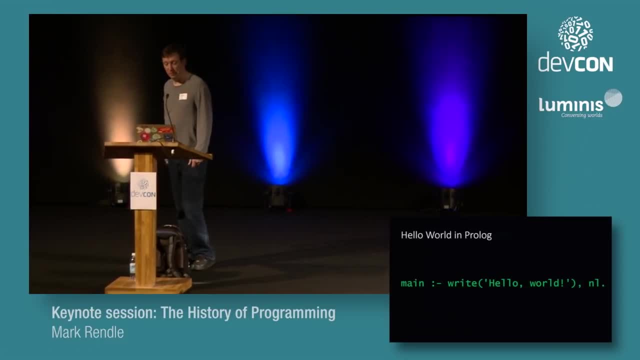 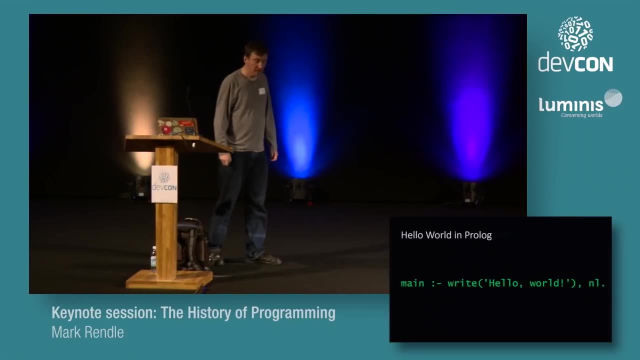 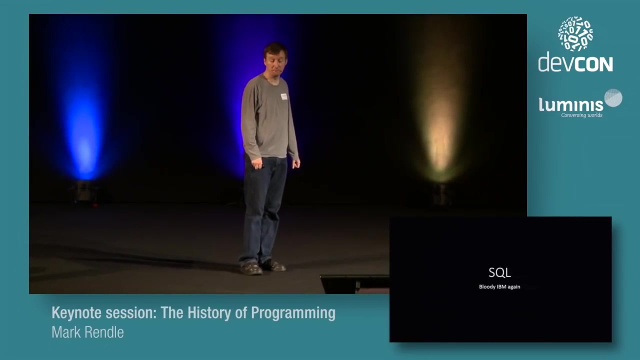 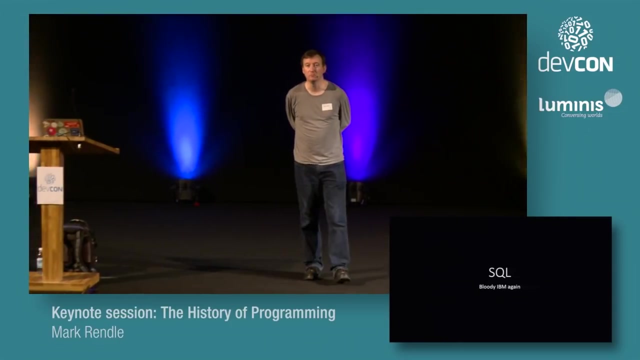 Maybe now we've actually got kind of bots as a service and machine learning libraries and Watson and everything else. People will finally shut up about Prolog and let it die. IBM created this. How is that pronounced? Hands up if you think it's SQL. 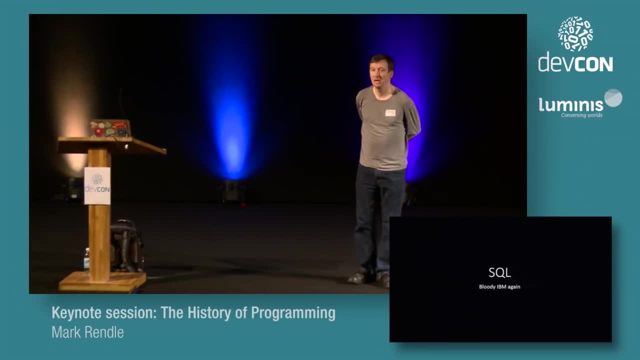 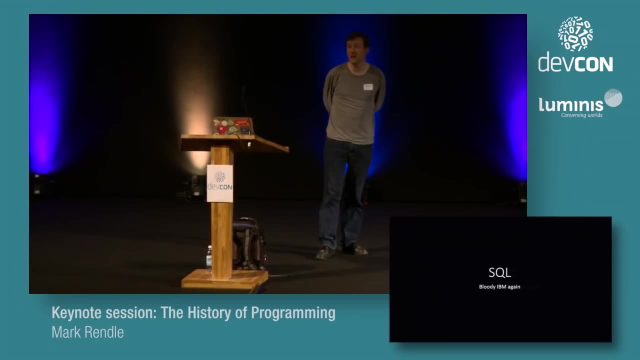 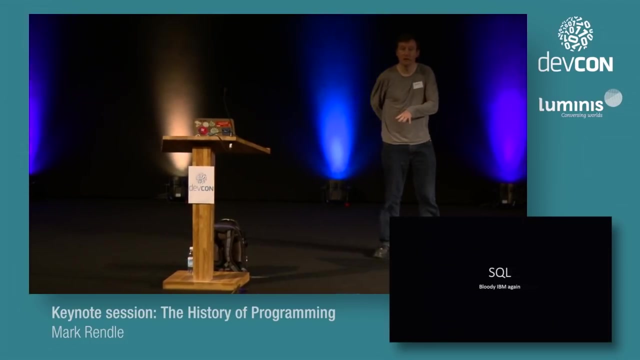 Hands up if you think it's SQL. Yeah, It is actually SQL, officially IBM. it was originally called SQL S-E-Q-U-E-L. IBM wanted to call it SQL It was. there was the kind of structured query language bit in there. 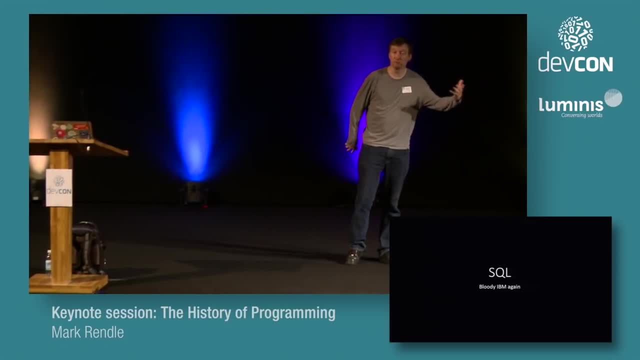 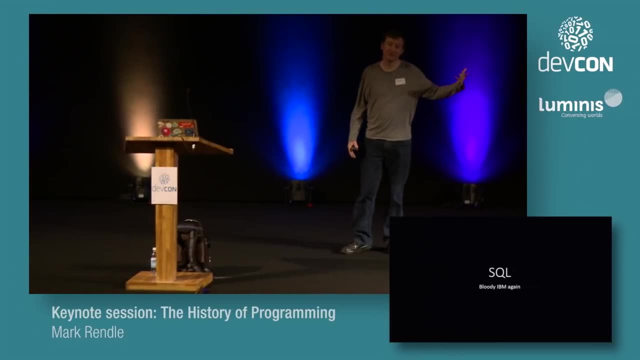 but they wanted to call it SQL because it was the follow-up to just raw CISAM instructions, So it was the SQL And it was for DB2.. And it was DB1, and DB2 was the SQL, So they wanted to call it SQL. 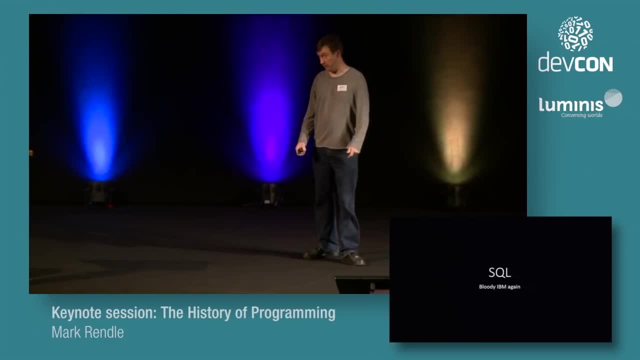 but they couldn't get the trademark, So they called it S-Q-L, said it stood for Structured Query Language, but then pronounced it SQL all over the place. So yes, next time you have that argument you can go well. Mark Rendell says. 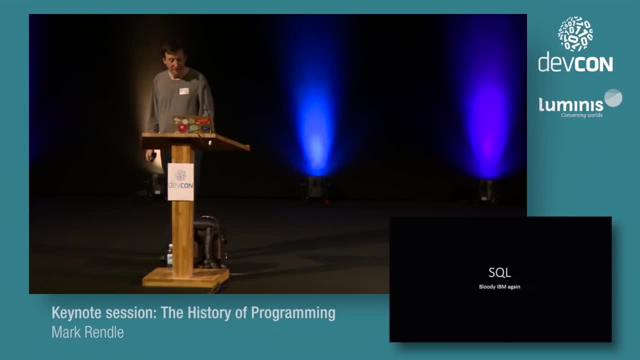 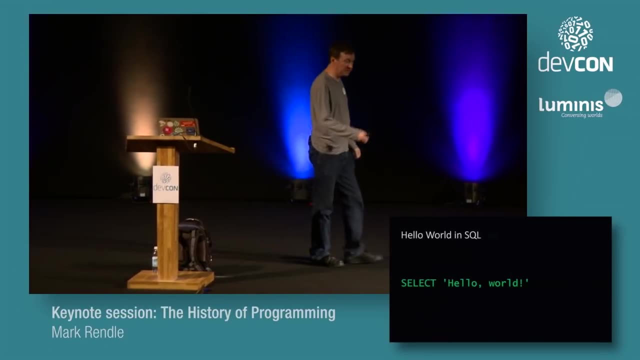 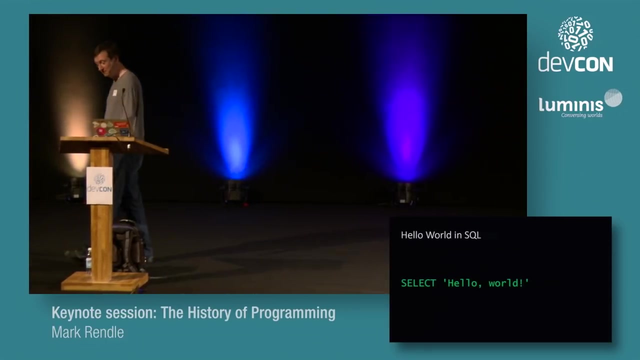 and then the person you're arguing with who the fuck is? Mark Rendell. I get that on Twitter a lot. Someone tweet that now Quick Is Hello World in SQL, Because you can. It does Now. a lot of people in the 1970s realised. 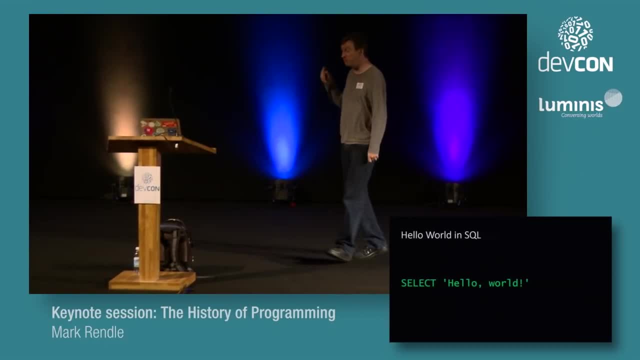 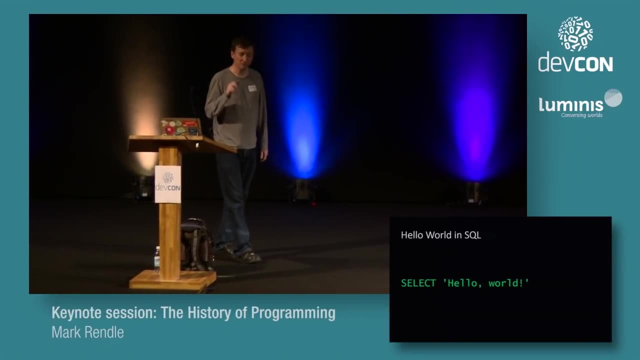 that C was going to take over the world and there was nothing they could do about it. but they really wanted to create a programming language. so why not just create a bloody stupid one? Literally, deliberately create a stupid joke- programming language. The 1970s was the first joke programming language. 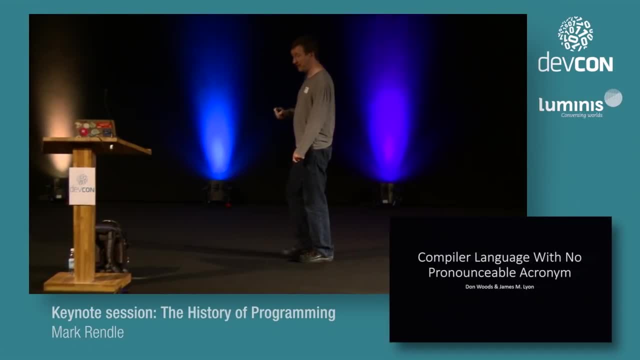 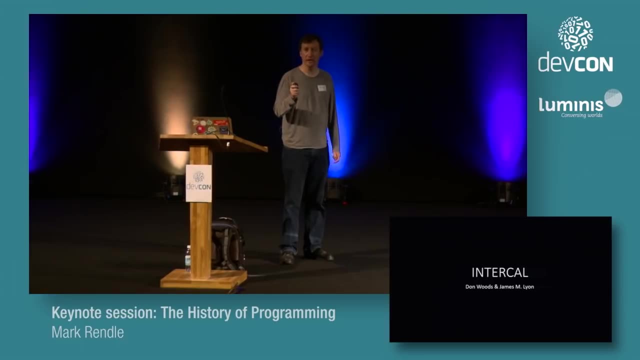 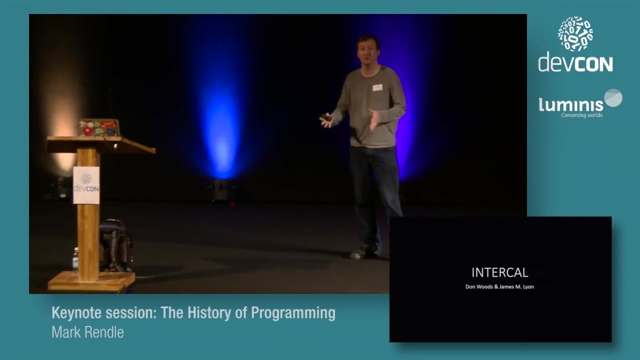 and it was called the compiler language, with no pronounceable acronym Or intercal And intercal. it is a complete joke programming language. There's lots of in-jokes and there was lots of digs at IBM and various other people. 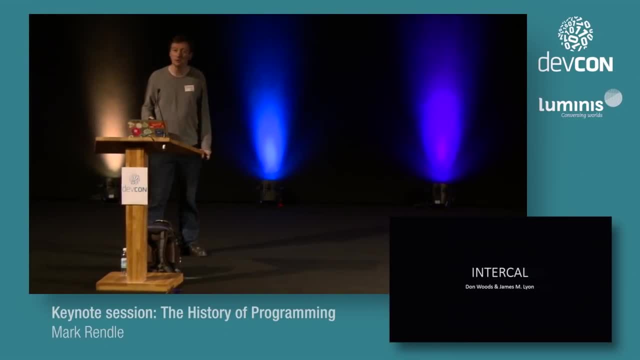 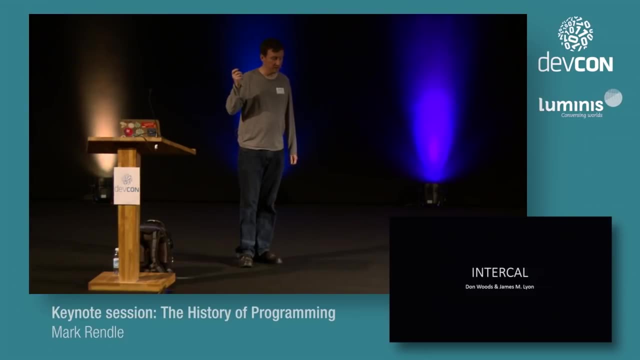 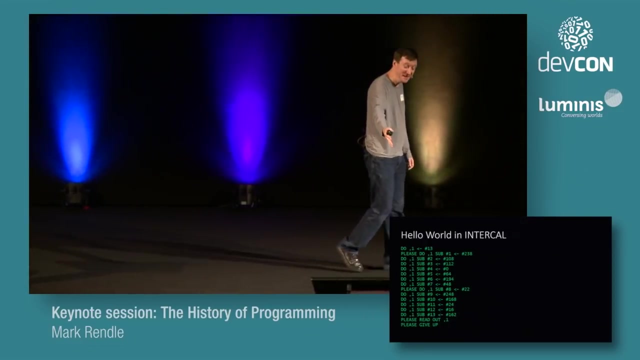 and it's very, very, very, very, very difficult to programme in, for reasons that will become apparent when I show you Hello World in intercal. Honestly, I'll put the slide somewhere. okay, and you can. this is not a picture. 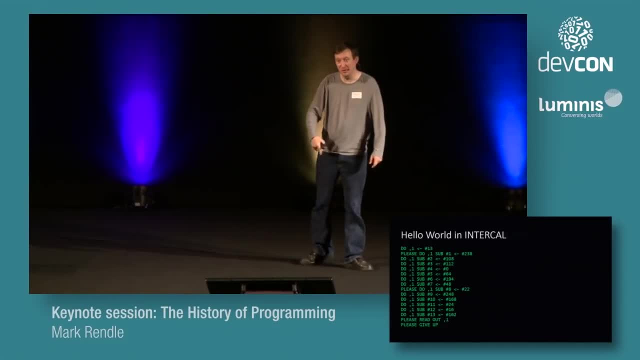 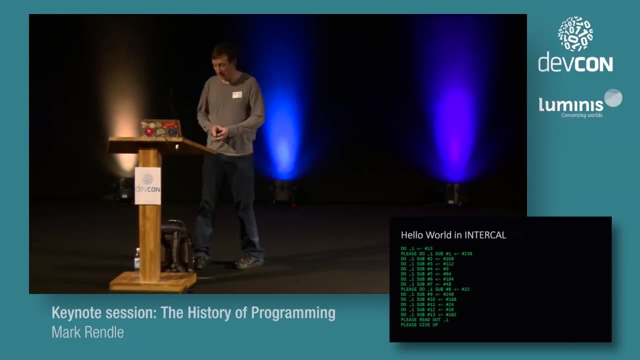 this is text. You can copy and paste that out of the slide and put it into an intercal compiler and eventually it will print Hello World out to the screen. So let's take a look at some of the stuff that we've got here. 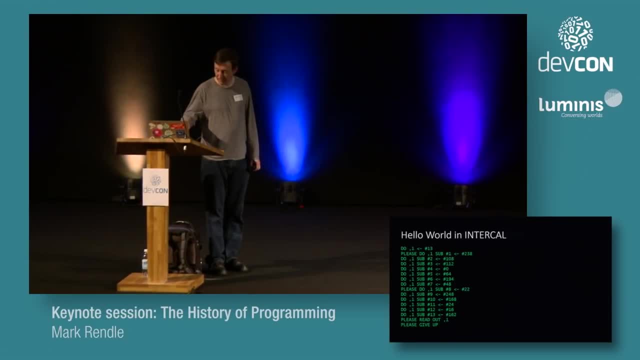 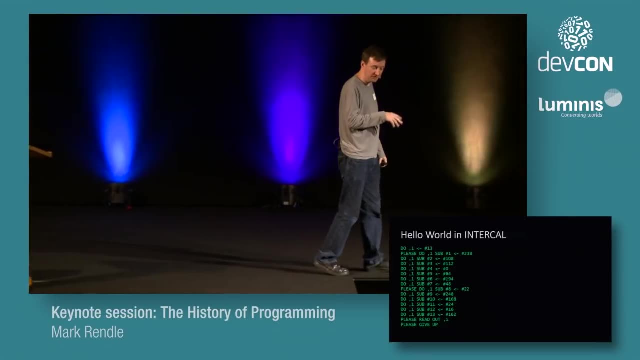 So we've got this. do one sub hash nine from this thing here. So this is basically just putting the ASCII values for Hello World into various registers and so forth And then down at the bottom you can see we've got. please read out. 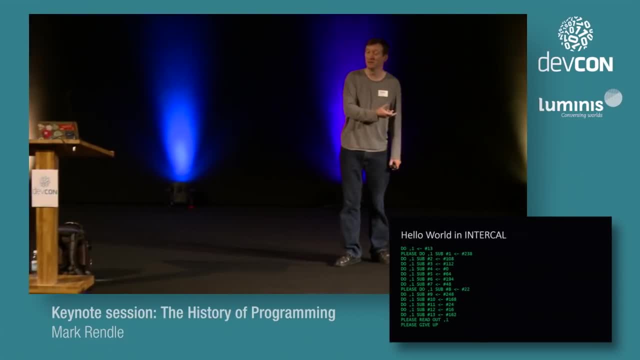 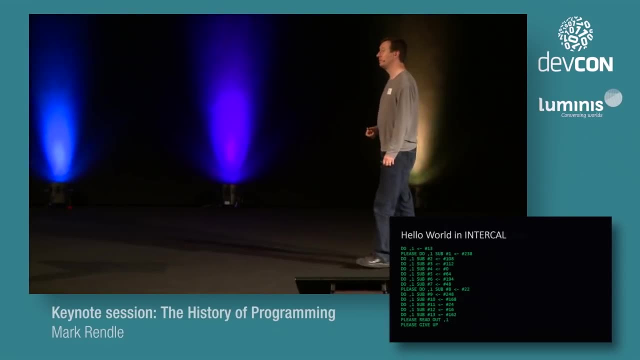 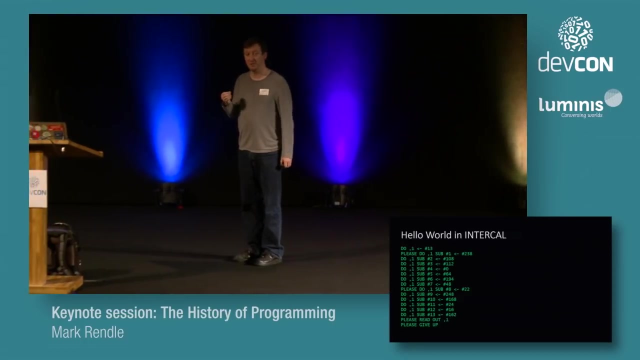 Intercal said read out to print and write in for input, just because it could, And then at the end, please give up. You had to end your programme with please give up because if you didn't, it would immediately start consuming 100% of the CPU. 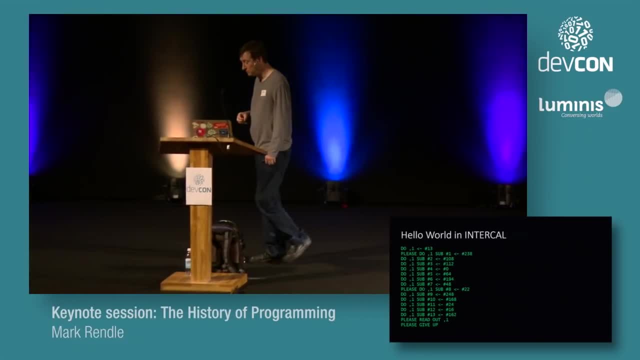 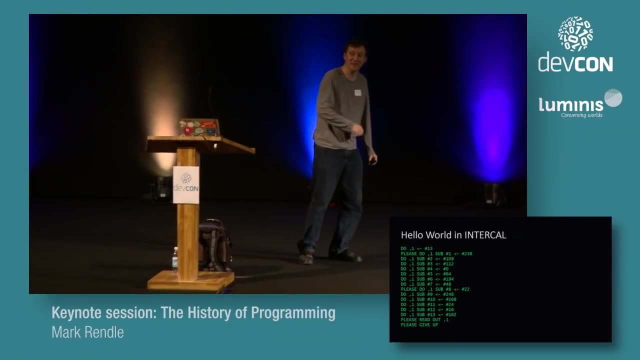 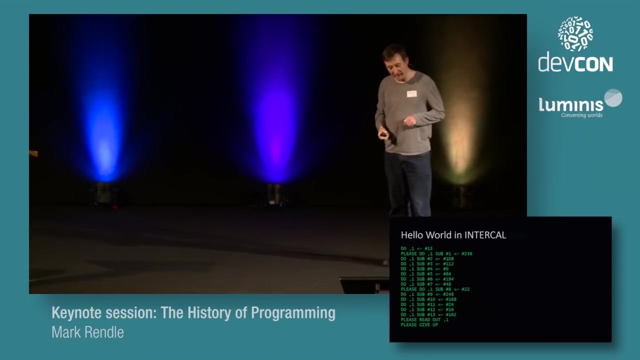 and kill your machine. That's in the spec, And if you create an intercal compiler that doesn't do that, then it's not compliant. There's some stuff in intercal that isn't in here as well. It didn't have go to. 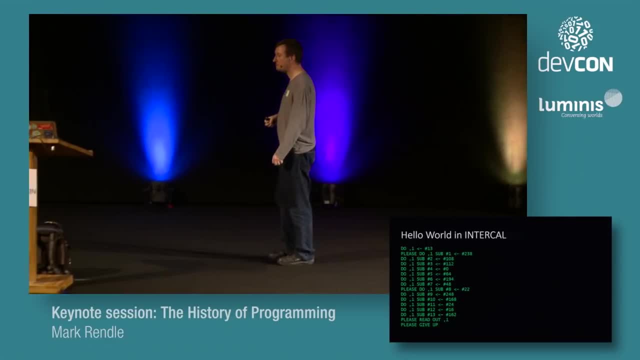 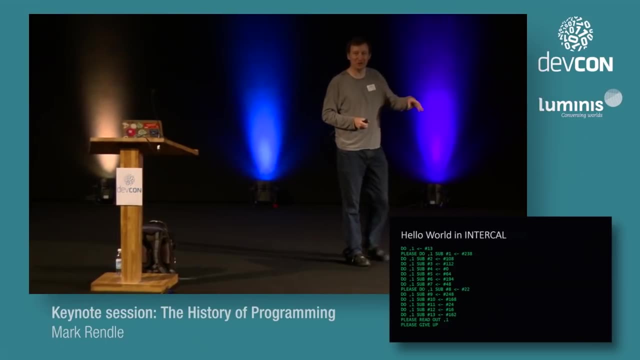 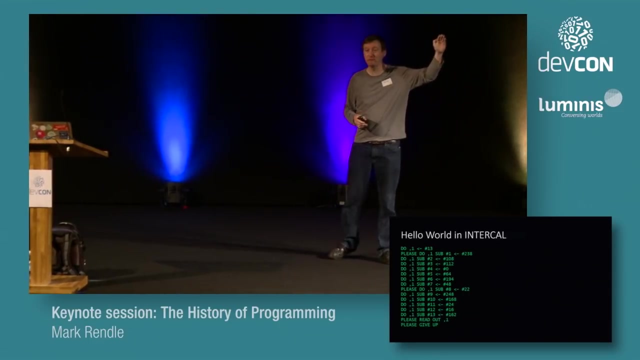 It had come from. And the thing is see you laugh, right, Because that seems so arbitrary. It's kind of: oh, we're going to come here from that line. It's identical. There is, semantically, there is no difference. 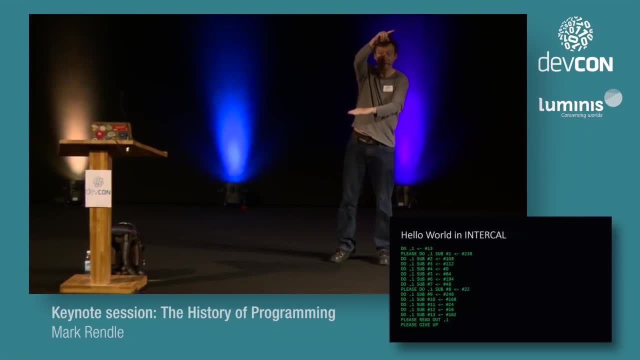 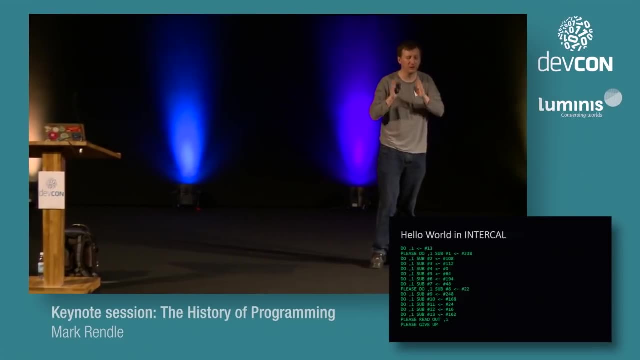 between having a line here that says come from that line or having a line there that says go to that line. It is identical, It's just for some reason go to you kind of go, that's fine, go to Come from. oh big laugh. 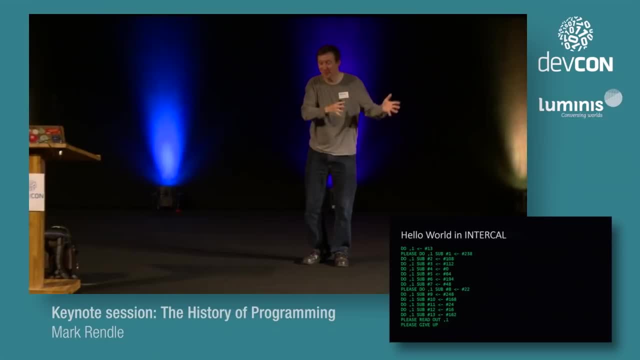 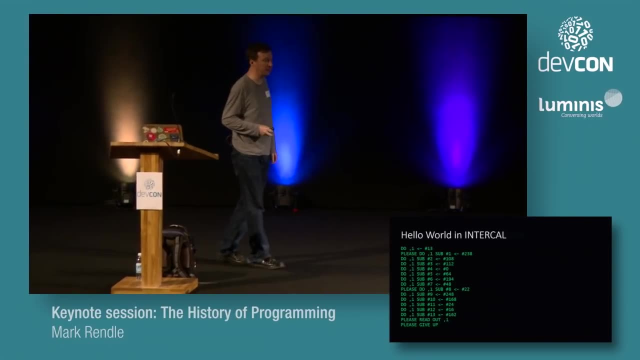 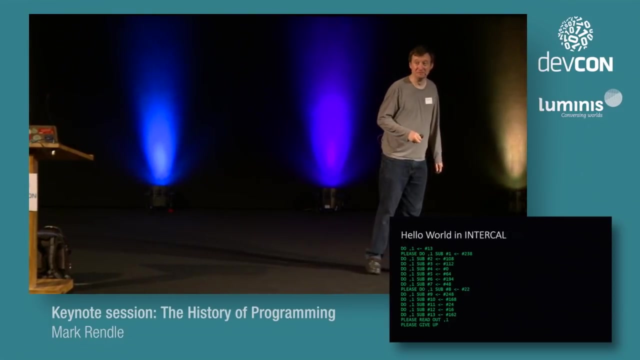 But no, there is no difference between those two things. There's lots of other fun stuff in there as well, but my absolute favourite thing about intercal is just these pleases. You have to say please some of the time, And if you don't start enough. 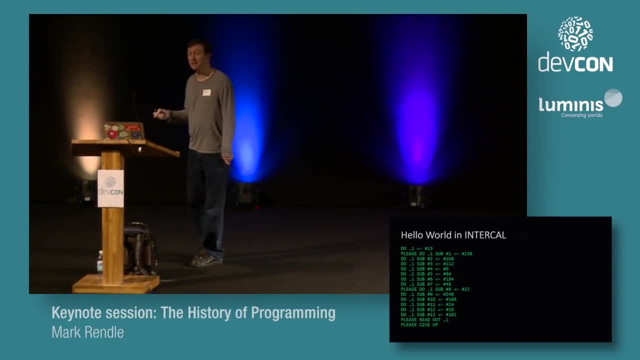 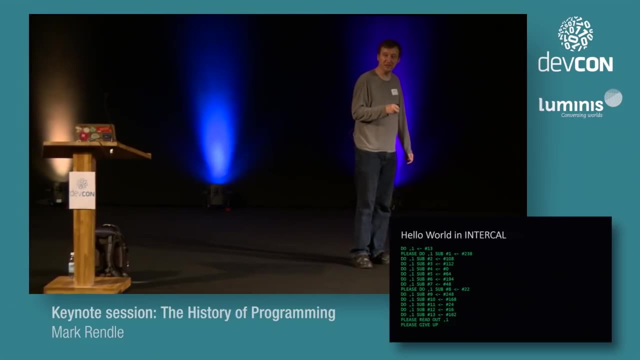 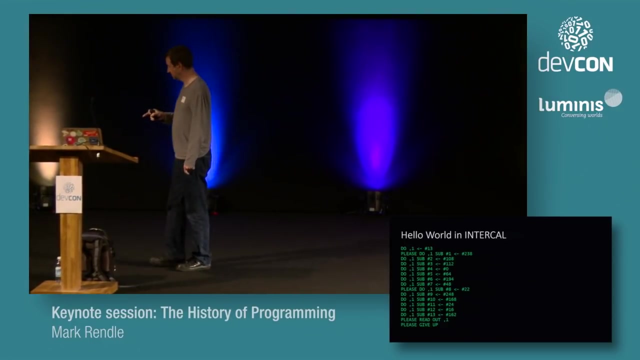 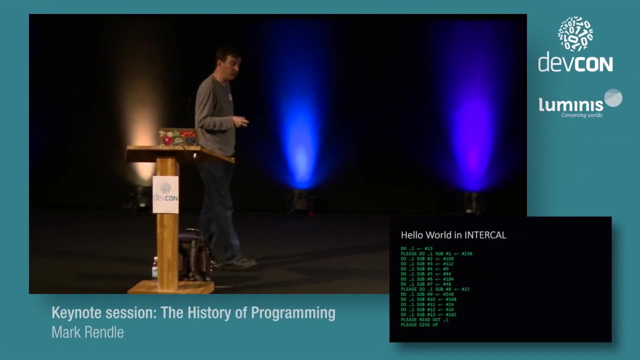 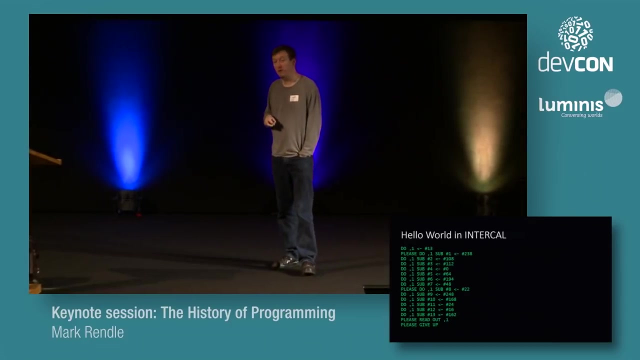 of the lines of the programme with the word please, the compiler will give you the error programmer is insufficiently polite. If you try to cheat, however, and just start every line with please, the compiler will fail with the error programmer is excessively polite. 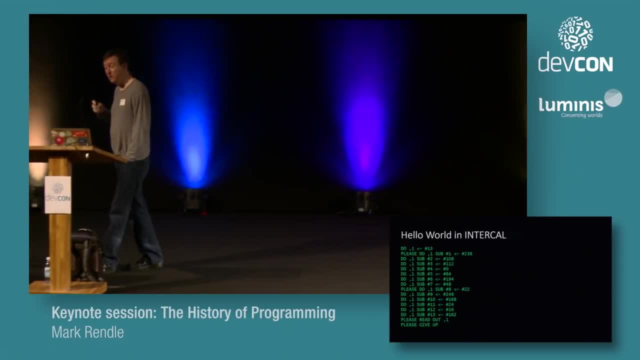 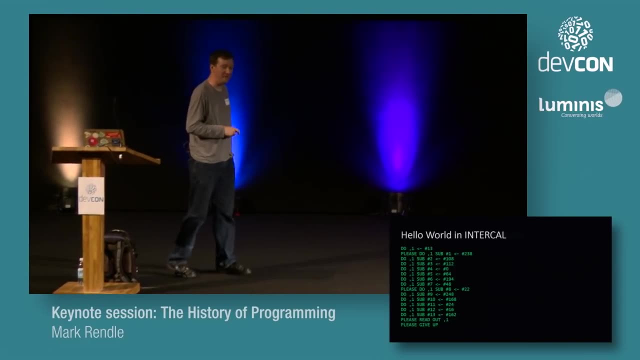 So you have to get the right number of pleases, which is not documented anywhere. I love intercal. I have a whole other talk which is 10 minutes of intercal. I've got code running and everything. It's great. 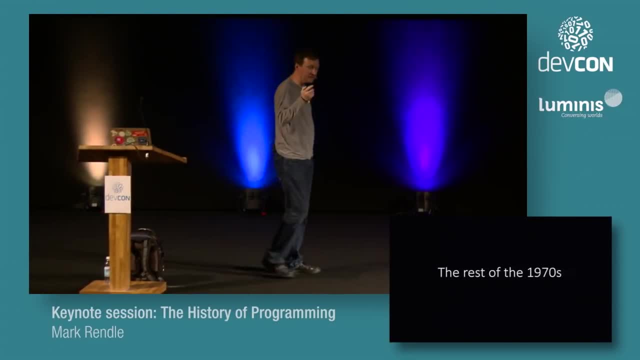 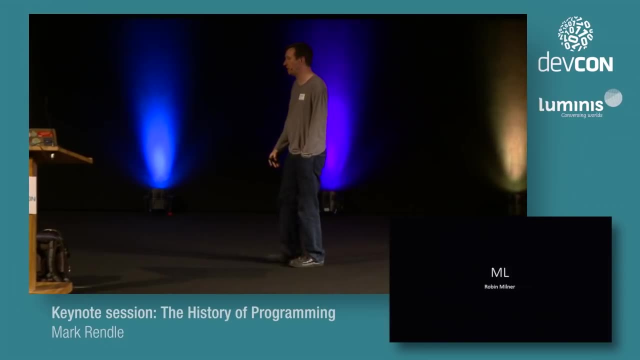 I love it. Rest of the 1970s: yeah, some other stuff happened as well. Robin Milner created ML, which then became Camel, which then became OCaml, which then became F sharp, which then became nothing at all, and nobody cared. 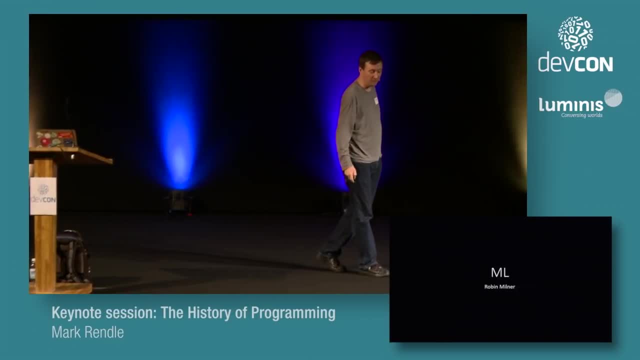 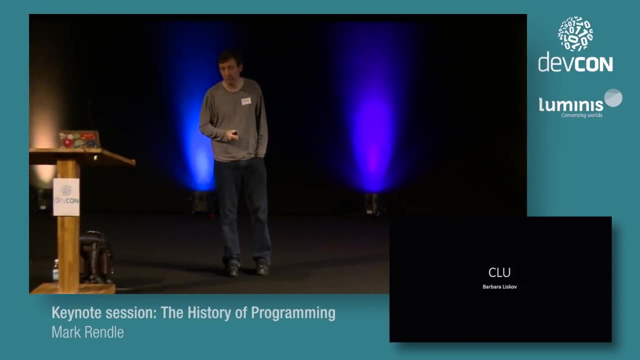 But yeah, that's kind of the whole functional programming side of things there. Barbara Liskoff created something called Clue in a doomed attempt to explain to people what the Liskoff substitution principle is, And still nobody got it. For those of you who don't know, 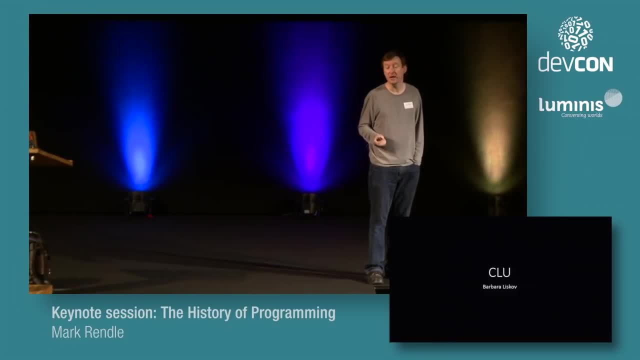 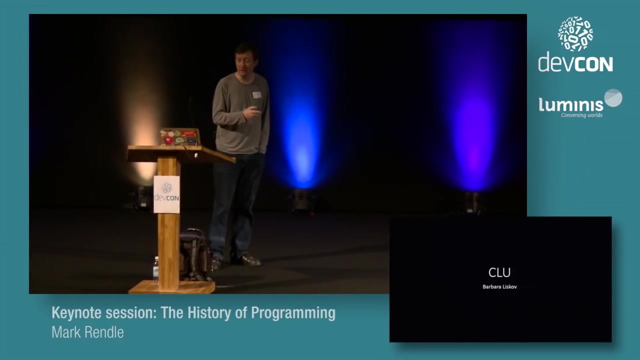 what the Liskoff substitution principle is. it's the thing that L stands for in solid, which Bob Martin only put in to solid so that it wasn't just soyed. It doesn't mean anything, It's entirely random and it shouldn't really be there. 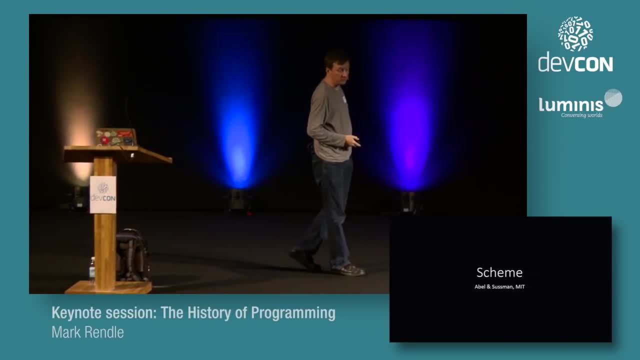 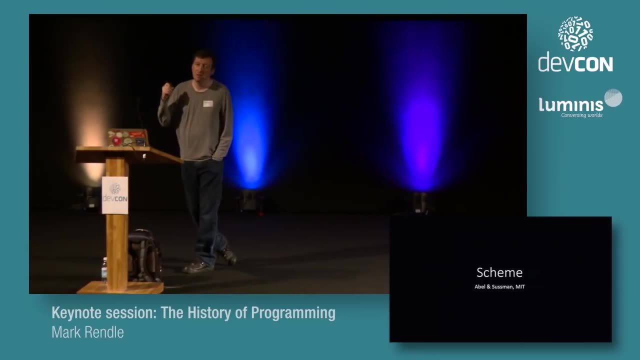 Abel and Sussman created Scheme, which was a simplified version of LISC, because LISC's so complicated, And they used that to create probably the most famous programming language introductory course in history- Computer Programming 601 at MIT. You can still learn Scheme. 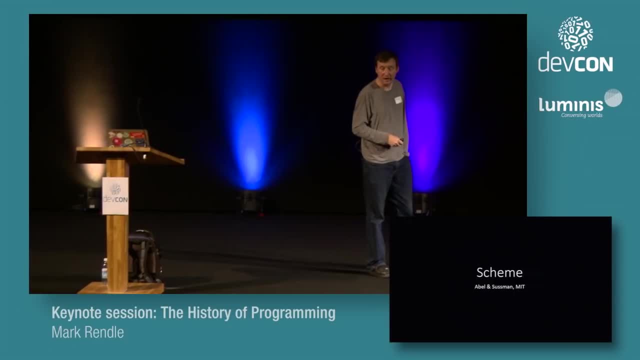 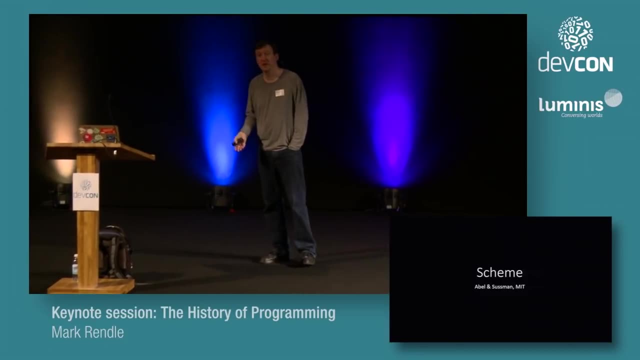 using their book Structure and Interpretation of Computer Programming. If you've ever got a spare couple of weeks between jobs or something like that and you want to do something interesting in programming terms, I do highly recommend it. I recommend working your way through. 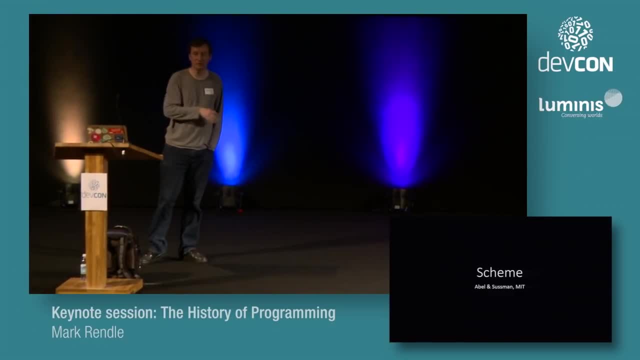 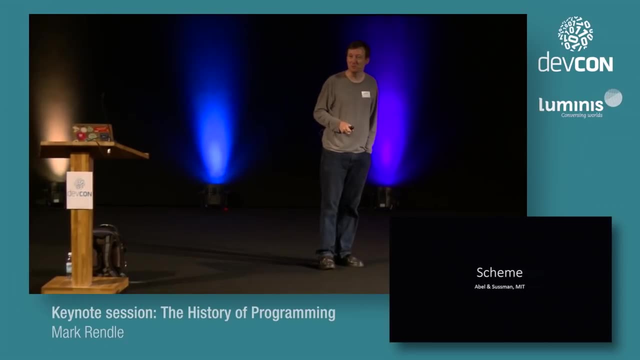 Structure and Interpretation of Computer Programming, SICP, free to download from the MIT website. It's great You get on to. I think it's chapter five, where they introduce the concept of mutable state. Everything up to then has been done. 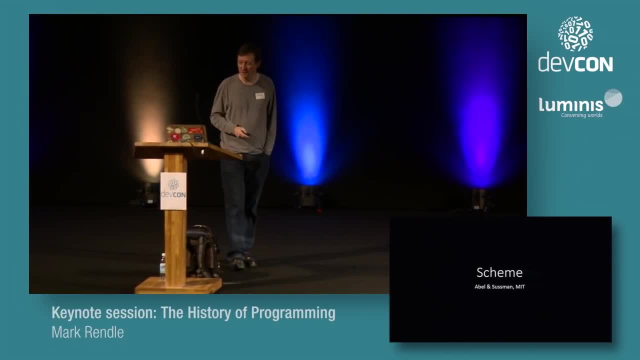 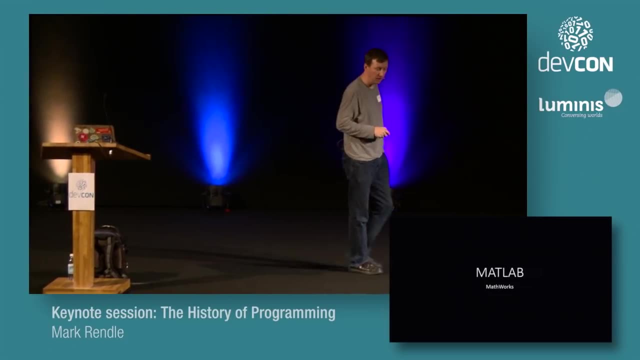 without mutable state and you start to go: oh, there are other ways to do things. MATLAB- that was created in the 1970s. Anyone use MATLAB. Very clever people Hurts my brain. VisiCalc was- I don't know really why. 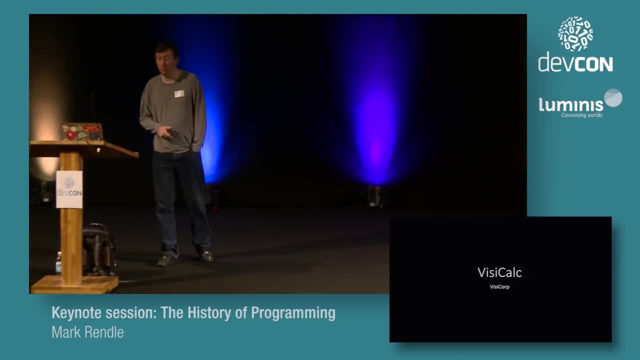 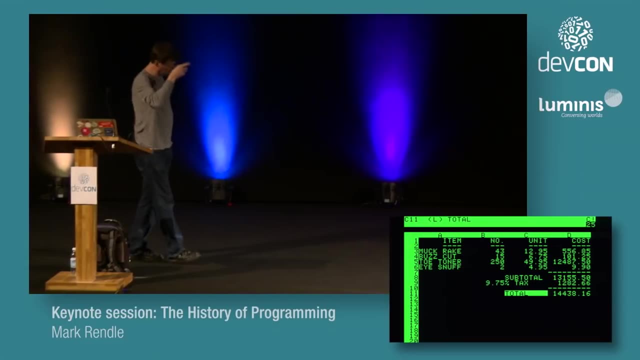 you can't do Hello World in VisiCalc. It's a spreadsheet, but it was a programmable spreadsheet. You had formulas and all this sort of stuff, and so I put it in. There's a screenshot of VisiCalc, and that was the 1970s. And then the 1980s started. I was seven when the 1980s started. In 1981 in the UK we got the first computer that you can actually pester your parents to go and get and bring back to the house. 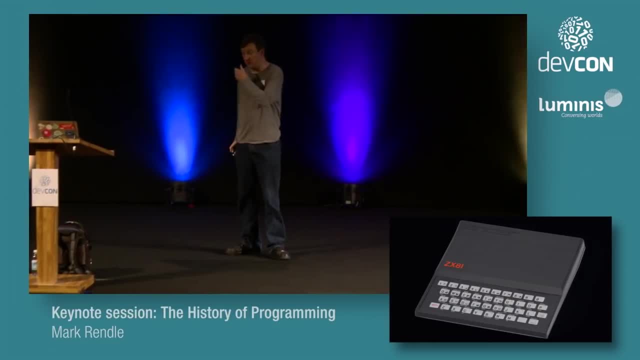 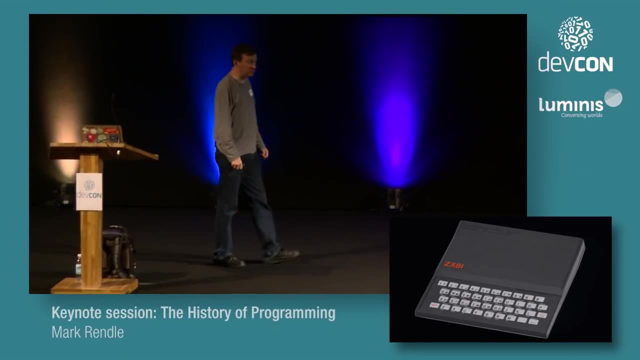 and plug into the television. and it was this one. Anyone have one of these? Yeah, I had a ZX81.. Terrible, terrible one. She had 1K of memory. You could generally get about 40 lines of BASIC into it. 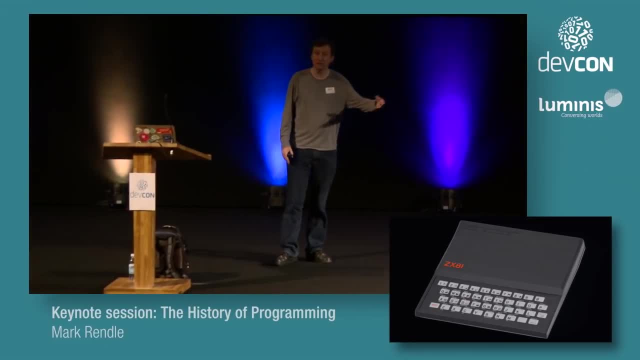 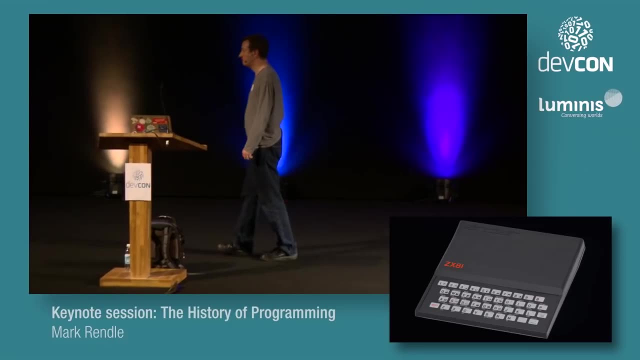 and then it would just run out of memory and it didn't have any memory left to tell you what was wrong. It just went And you'd have to work it out for yourself And the keys here. that's basically just a sheet of plastic. 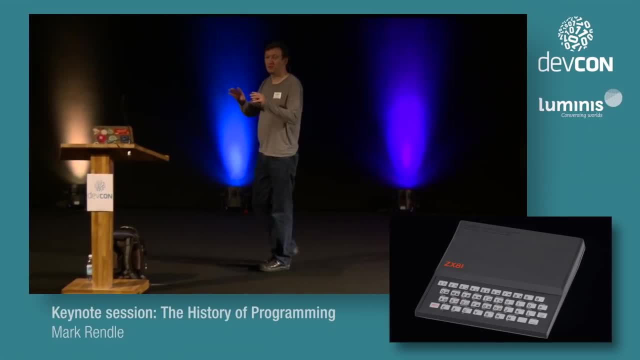 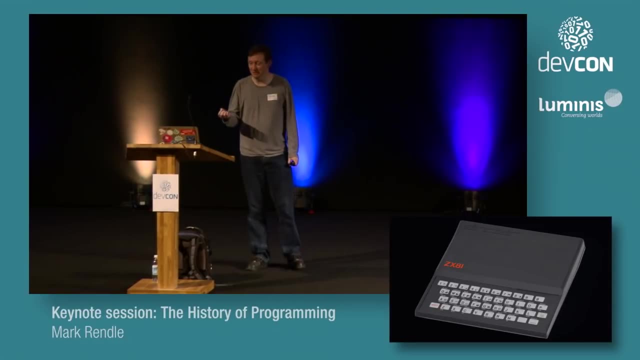 and the keys are printed on And on the box it said touch-sensitive keyboard. Those weren't. An iPhone is touch-sensitive. These things were like hammer-sensitive. You'd be there. just fucking do the print keyword. bloody hell. 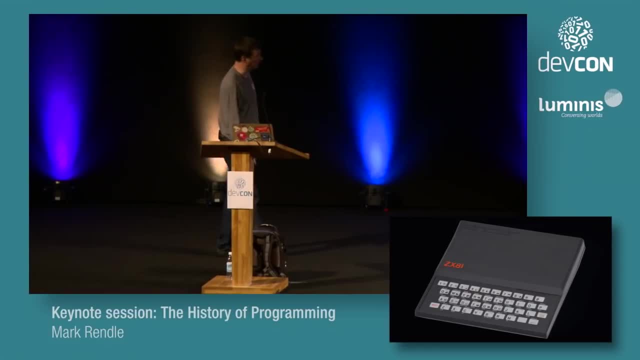 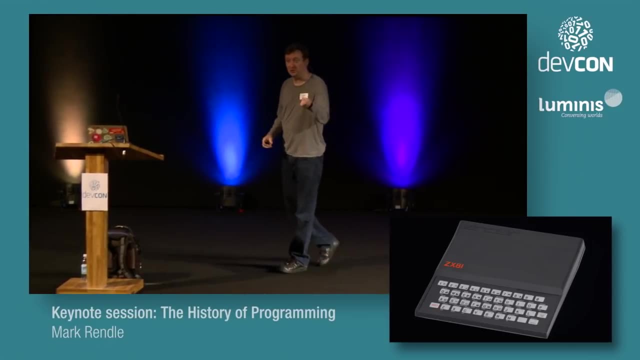 Yeah, All to try and fill up the 1K of memory and see if you could get a thing to crash. But I learned to program on that. The really cool thing about the ZX81 and all the Sinclair machines is that the keys didn't just have P on them. 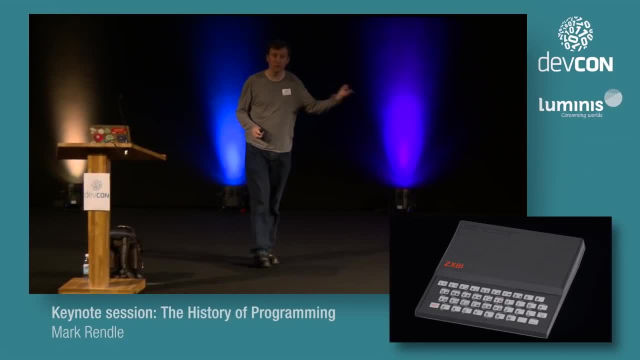 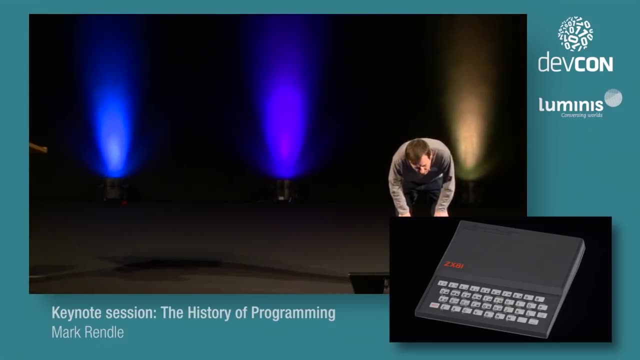 They also had BASIC keywords on, And so the way I learned programming and the way I learned more about BASIC than you would have got from a book is kind of staring at the keyboard and going: what does unplot do? That sounds, Oh. what's LList do? 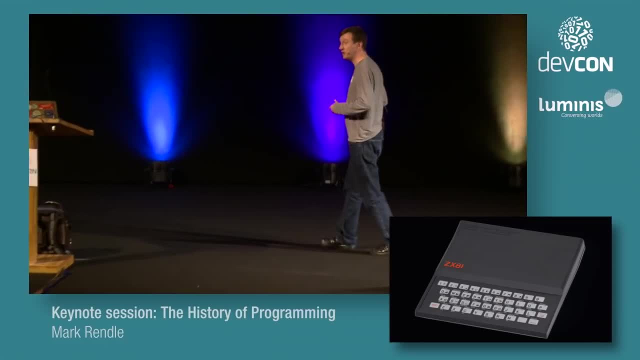 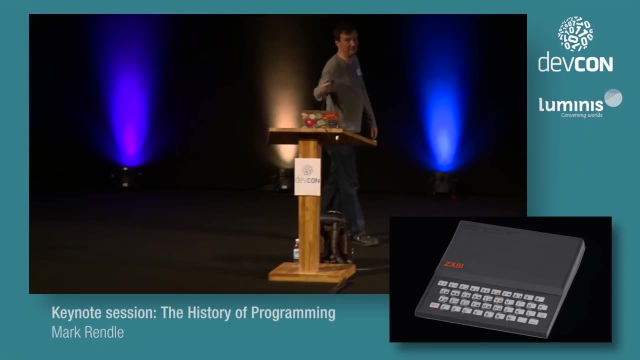 That's in red. That must be really cool. And I kind of explored the language just by finding words on the keyboard and then going to the paper manual to find out what they meant And, of course, eventually, 1K of memory. 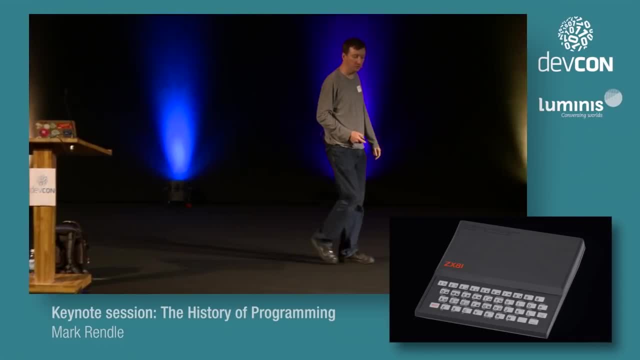 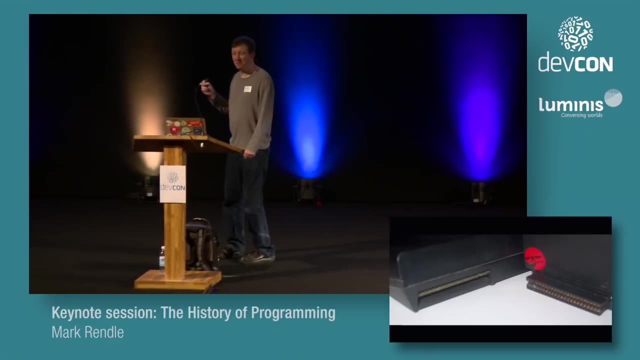 you know, even with that exhaustive amount of RAM, you're going to run out sooner or later. And so you go and pester your parents some more and go. can you buy me 16K of memory For something like 140 pounds? 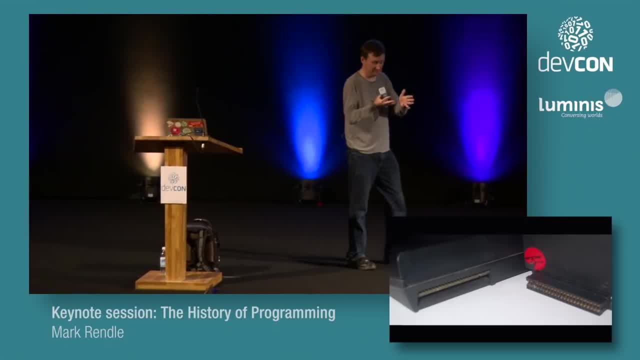 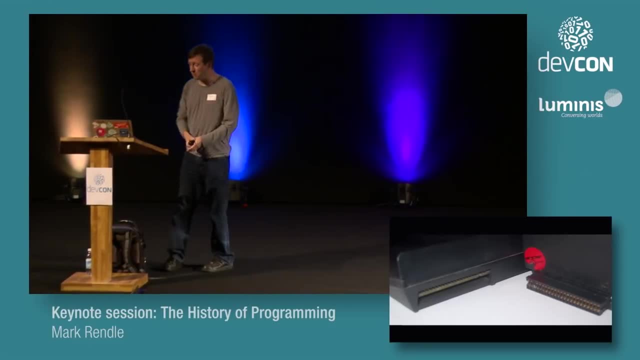 it was insane And it came like this: And that is just a very wobbly copper connection, And so you plug it into the back and you go: I have 16K of memory. And then you start programming and of course you're just doing this. 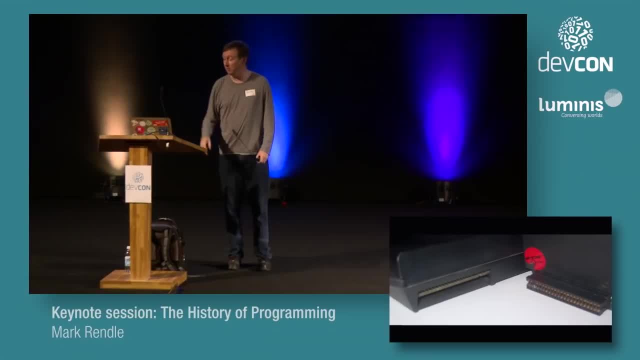 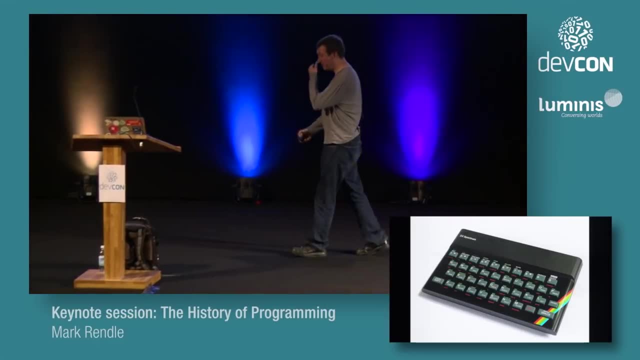 to try and get the, And then the RAM pack would wobble and the connection would break and the whole thing would crash. Yes, So then this came along. This was the Sinclair ZX Spectrum, And this had even more: It had 48K of memory. 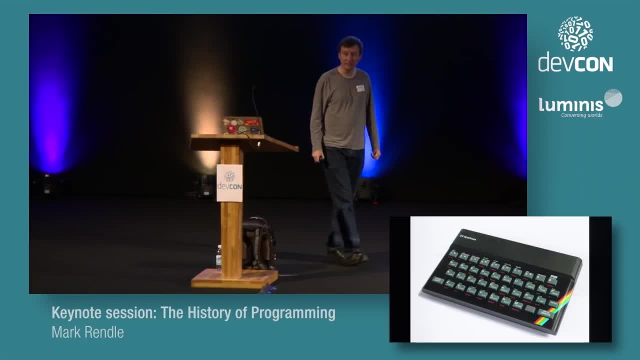 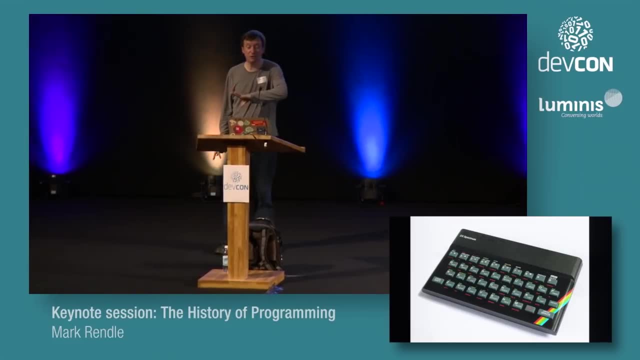 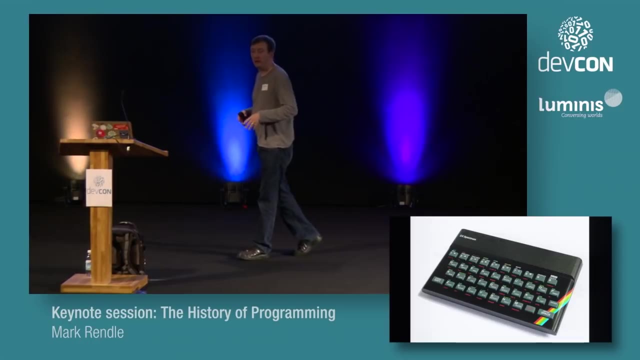 if your parents were rich enough to buy you the more expensive version of it, And who had a Spectrum? Yes, So you sort of learned to program, but if you wanted, The Spectrum was the first thing I learned. Z80 Assembler on the Spectrum. 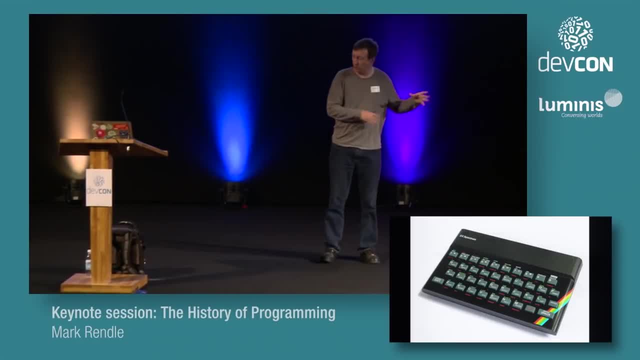 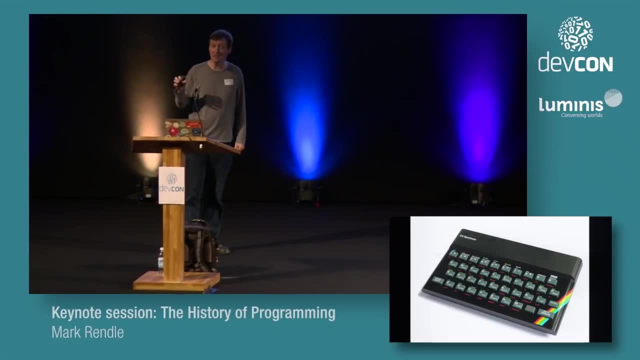 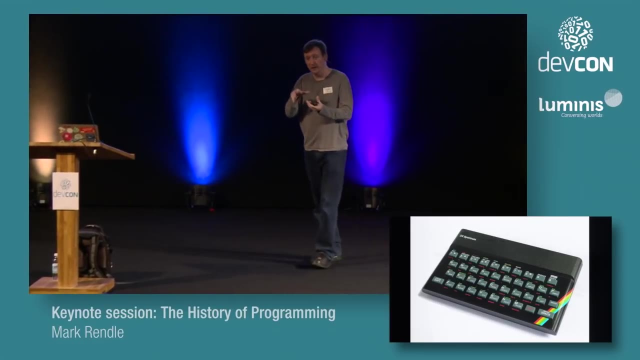 which was proper programming, And this was how you could actually get it to do proper things like play games and so forth. And in those days software came on cassette tapes. Cassette tapes were strips of magnetic material wound around two spools in a plastic case. 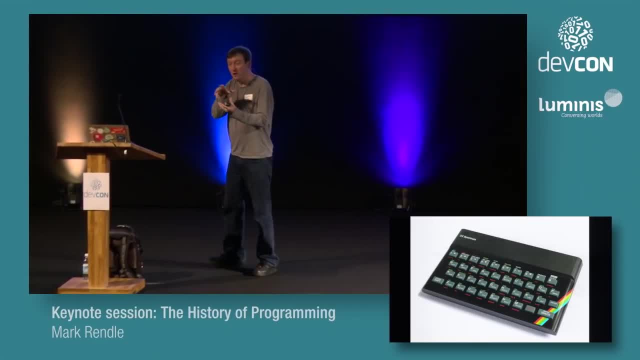 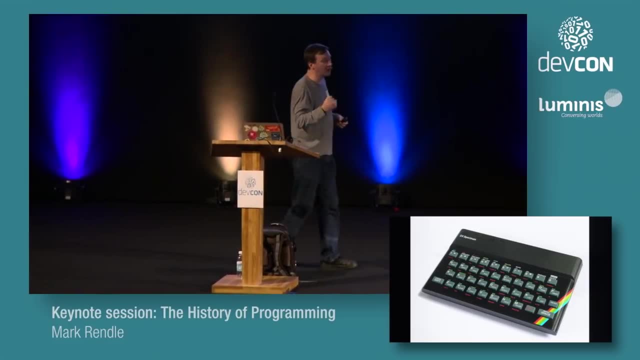 Seriously, there are people in the audience who don't know. I find this very depressing. Floppy disks used to be floppy, That's what the little save icon is. But yes, you get it on a cassette tape And copying cassette tapes. 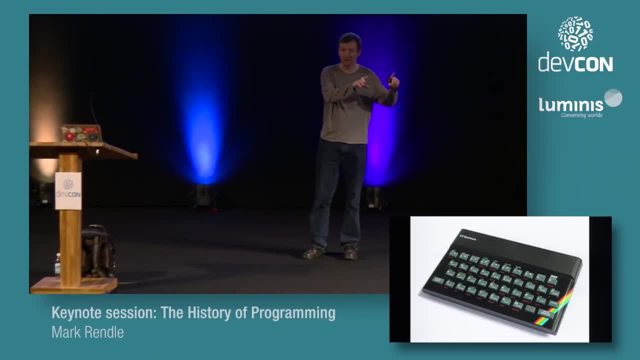 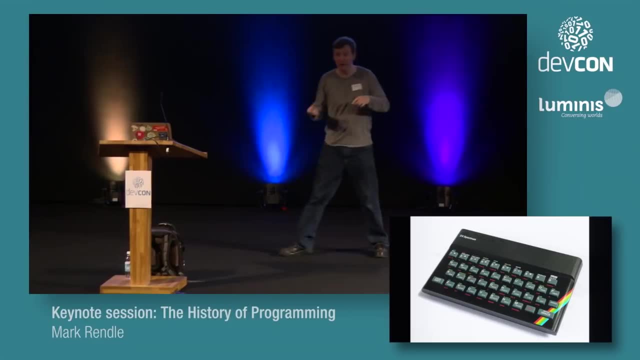 you literally have to get one cassette tape which had something on it and then run it all the way from start to end and record the sound that it made onto another cassette tape. But if you wanted to make another copy you had to rewind this one and then do it again. 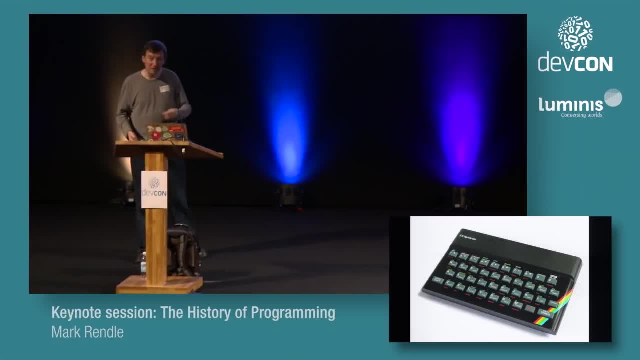 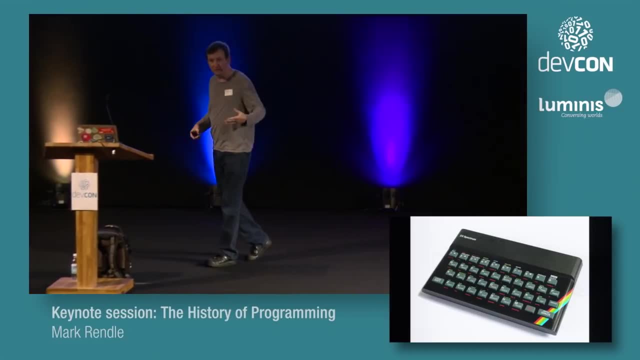 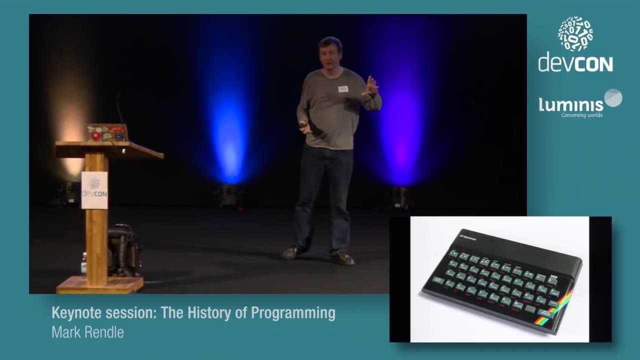 So distributing software was really quite complicated and expensive. And so you know you get magazines these days that have got disks on the front with Linux, because you've got a crap internet connection and can't download Linux for some reason. But in those days, putting a tape on the front of a magazine, 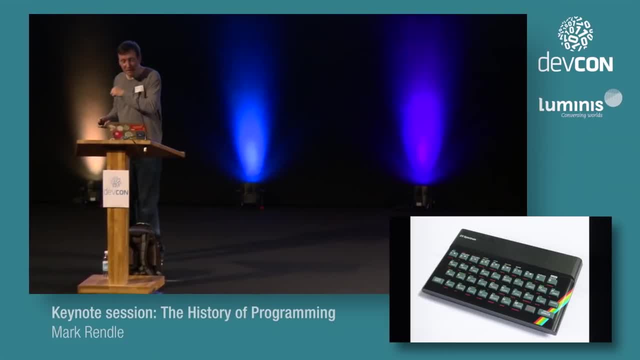 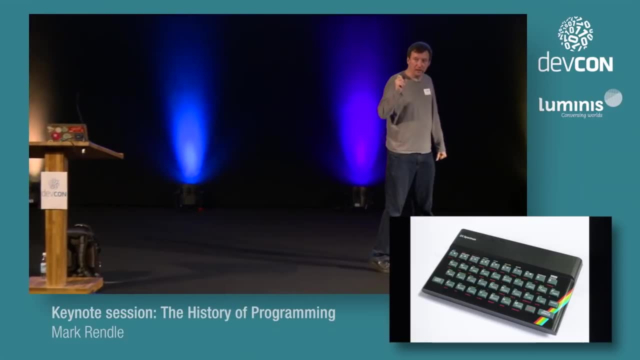 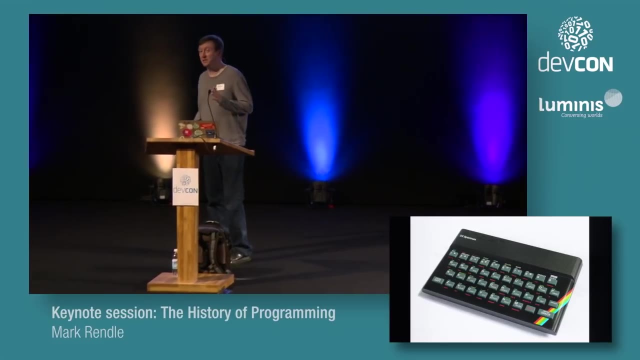 was an expensive proposition, And so some very, very clever person at the computer magazines of the 1980s went: why don't we get the game running on a Spectrum and then just dump the entire memory out and print it in the magazine? 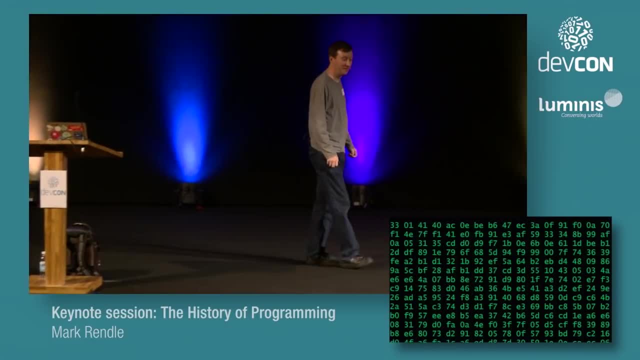 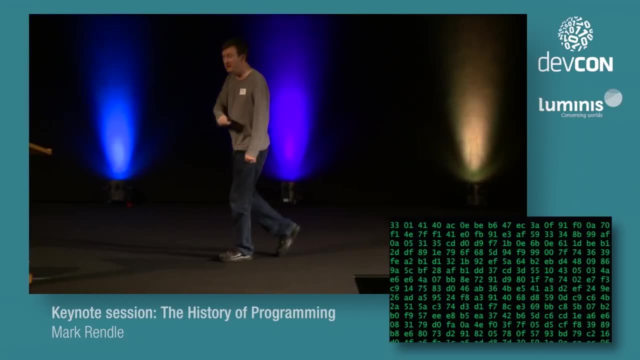 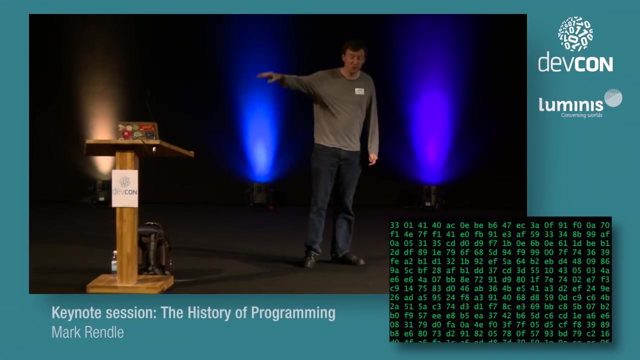 That'll work. Seriously, people in the audience will back me up on this. If you don't believe me, ask an old person. Six or eight pages of a magazine would just be filled, literally filled, nothing else, just Well. no, actually that's not entirely true. 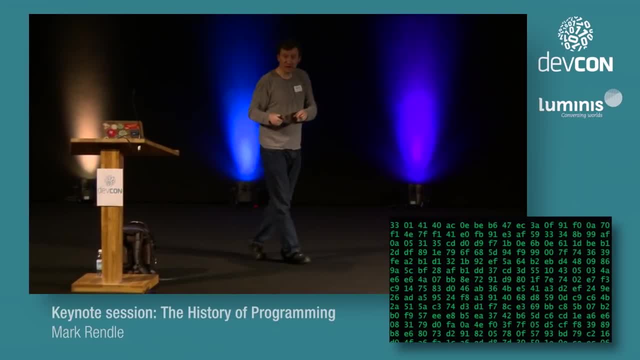 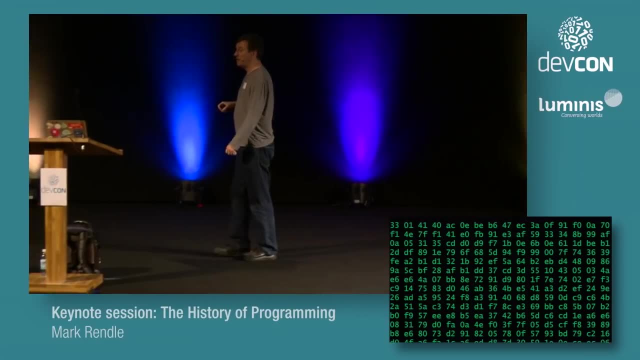 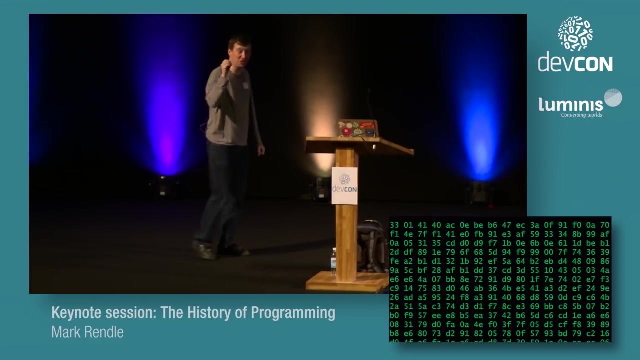 They would be filled with mostly this, with the occasional picture of what was promised to run once you'd typed all the numbers in. None of them ever worked, But because it was just a raw dump of the memory state that had to be in the Spectrum. 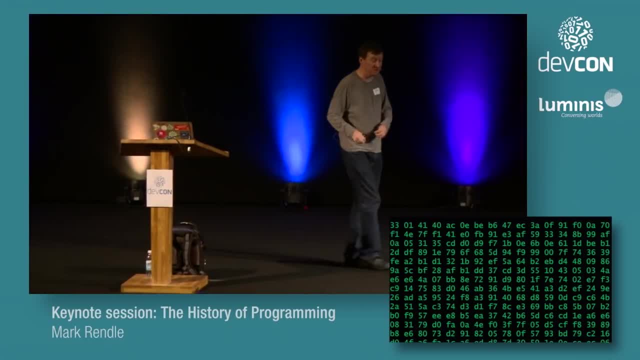 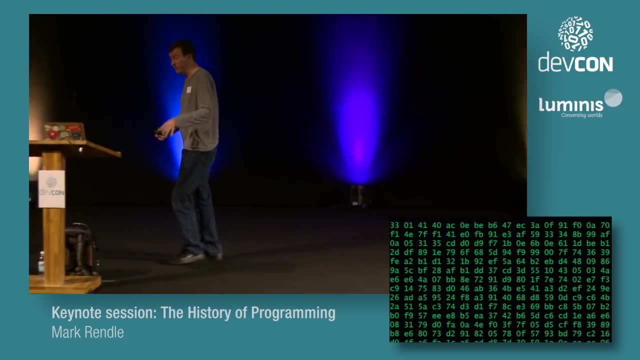 in order for it to be running. you couldn't debug it, You couldn't kind of go: oh well, that 92 should clearly be a 93. No, And you wouldn't know that it didn't work until you typed in the last character. 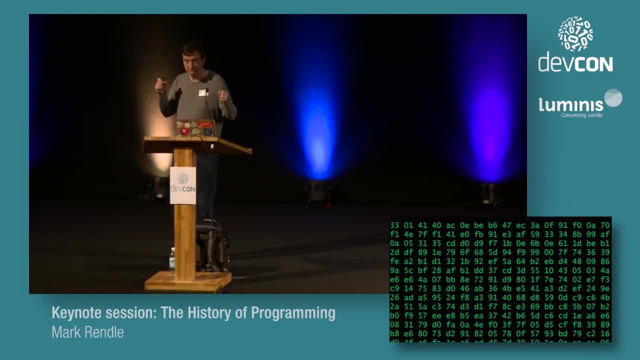 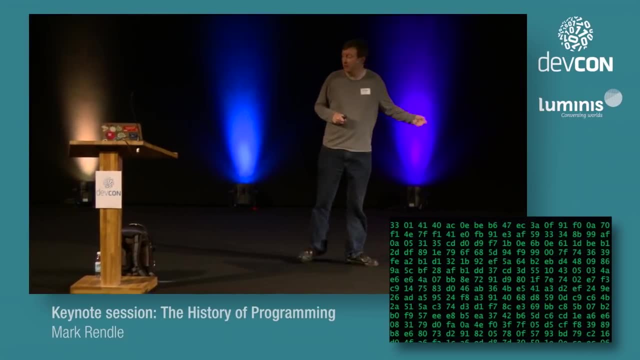 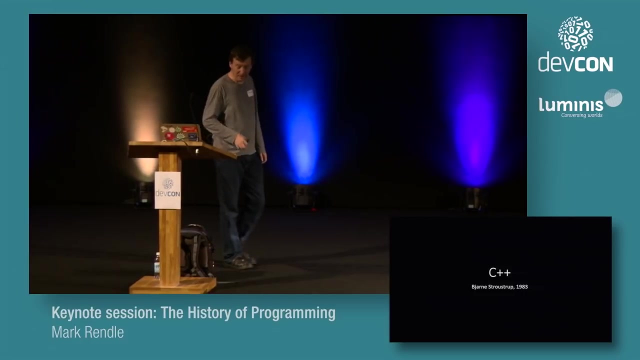 and sat there and went: nothing's happening. Should we go back and check what's doing this, or should we just hit each other with pieces of 2x4, which will probably be more fun? So, yes, that was my junior programming experience. 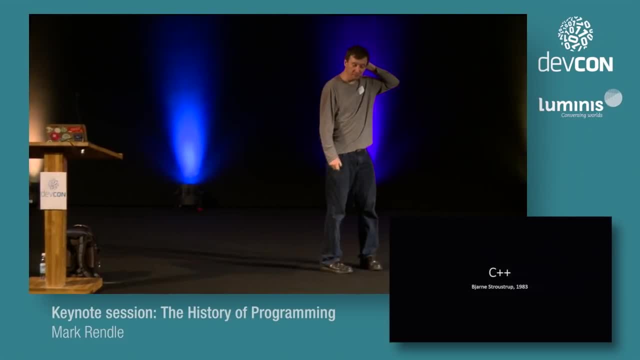 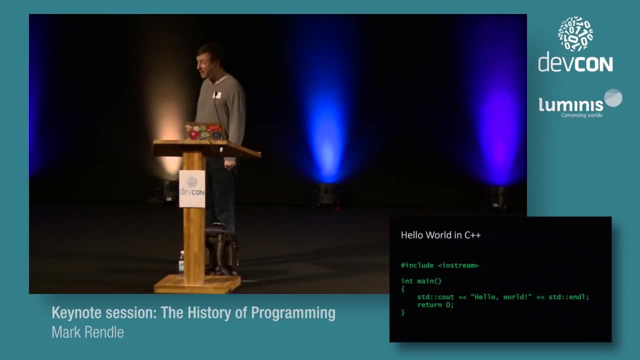 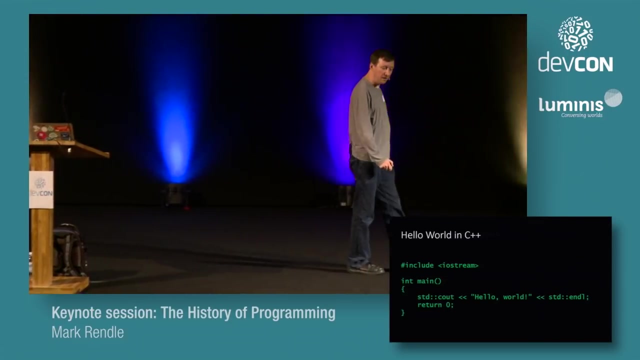 And then, of course, C++. That was created in 1983, which made a lot of people very angry. Here's Hello World in C++. Yep, that's definitely better than C. We can totally see why that took off. Not really sure. 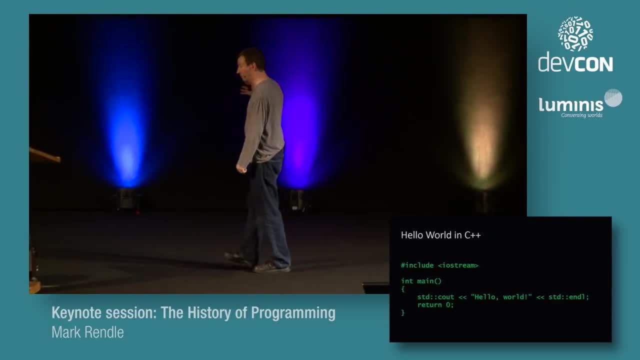 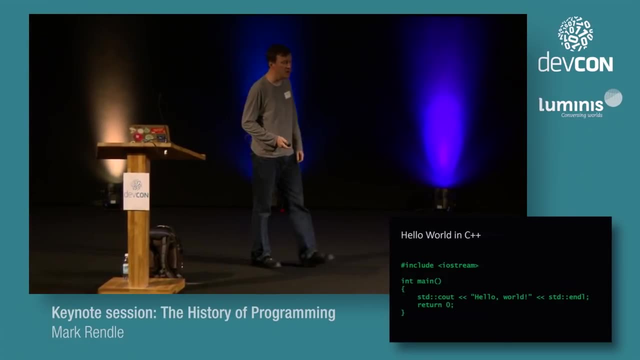 And, of course, C++. that was one way of doing object-oriented programming. Apple, at this point, were getting all kind of up themselves and becoming the Apple that we all know and love today. And so, Apple, they created Objective-C. 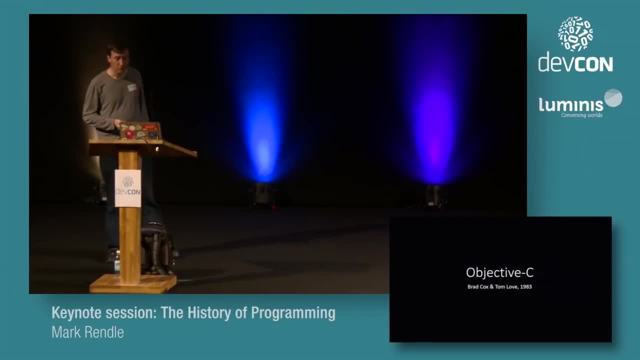 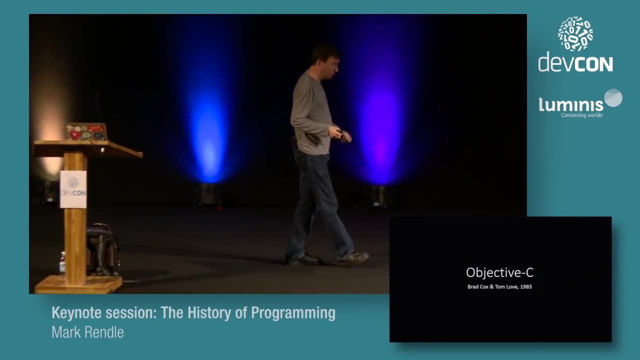 which was their own um object-oriented version of C And actually the recipe. if you want to make Objective-C, the recipe is very, very simple. All you do is you take the best bits of C++ and the best bits of Smalltalk. 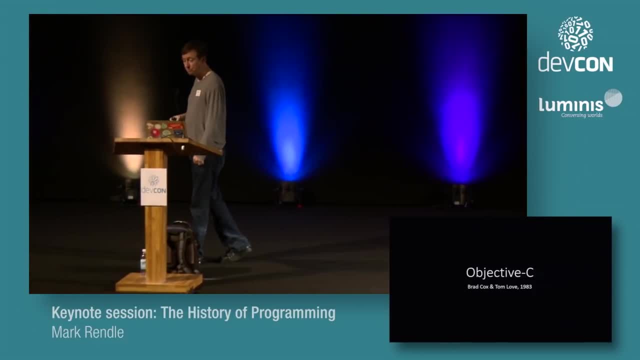 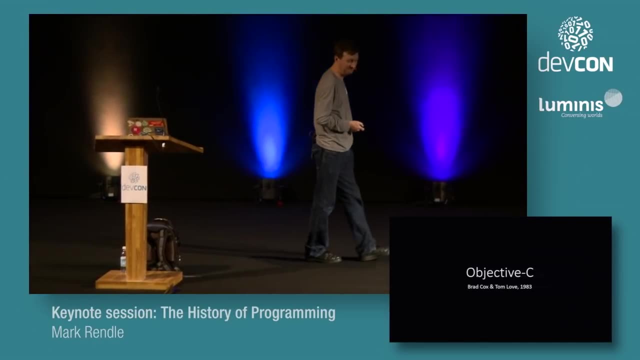 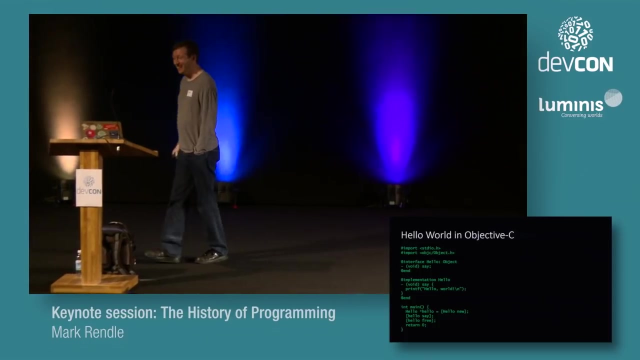 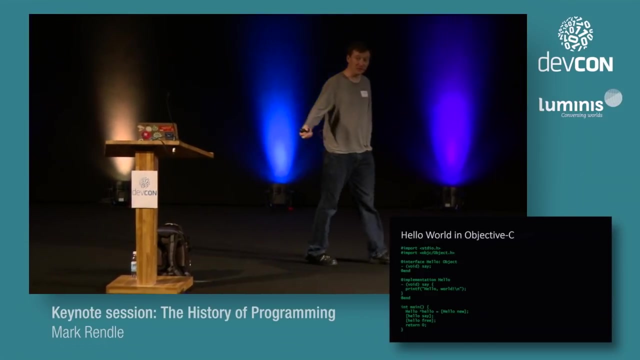 and you throw them away And what you have left will be Objective-C. It's Hello World in Objective-C, Oh dear, But object-oriented programming. obviously everything had to be able to do. object-oriented programming, Not message-oriented programming, object-oriented programming. 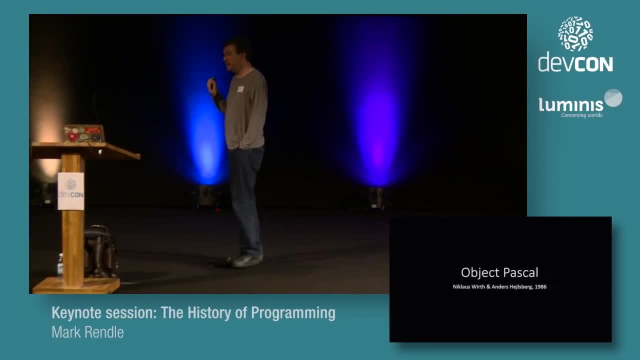 And that's how we got Object Pascal. Literally, Object Pascal is only in here because the secondary designer, the kind of right-hand man of Niklaus Wirth, was Anders Heilsberg, who you may have heard of. He created some other languages. 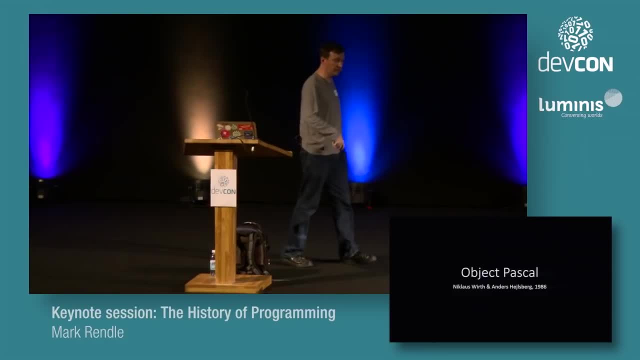 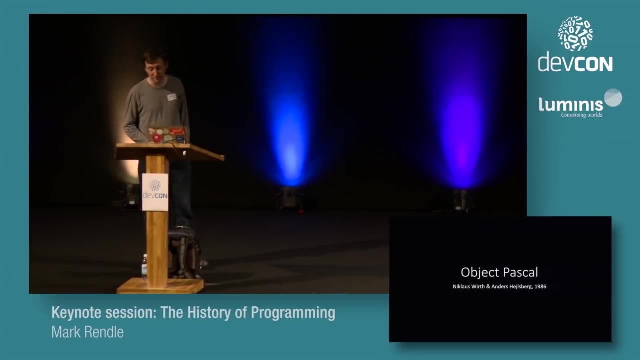 And some of them are quite good. So yes, Hello World in Object Pascal looks exactly like Hello World in ordinary Pascal, so there's not much point. Another guy working over at Apple had this brilliant idea because he was going: oh, these 10 prints and gotos and gosubs. 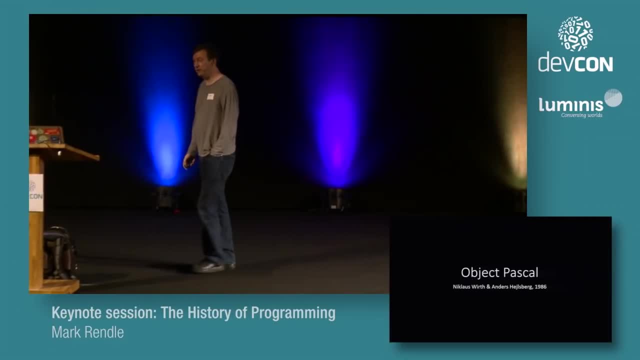 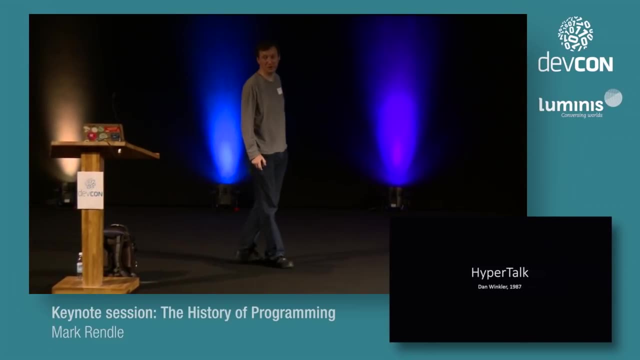 and writelands and printlands and all this sort of stuff. What if you could just talk to your computer in English? So he created a programming language called HyperTalk. Has anyone ever actually seen HyperTalk code? Yeah, yeah, So you will back me up on this. 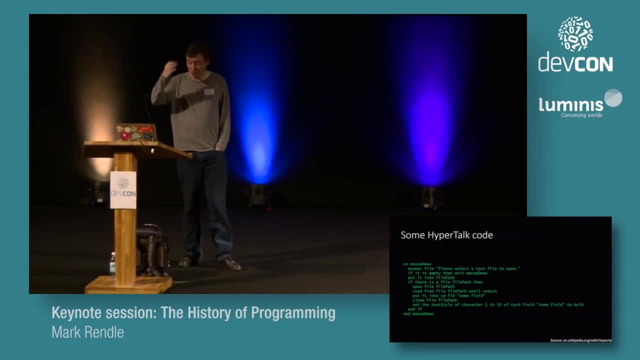 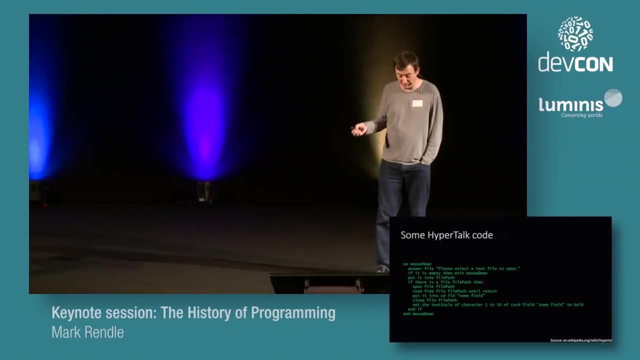 I'm not making this up, That's HyperTalk code. It's literally answer file. please select a file to open. If it is empty, then exit mouse down. Put it into file path. If there is a file file path, then open file file path. 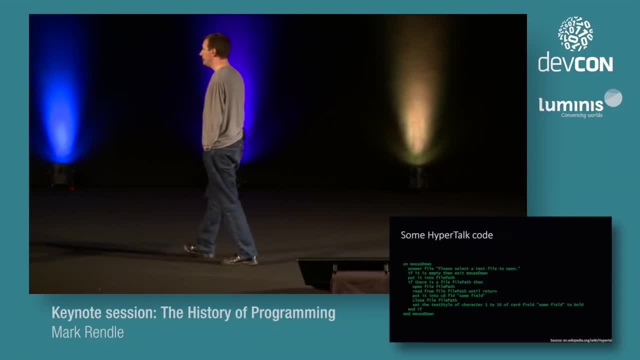 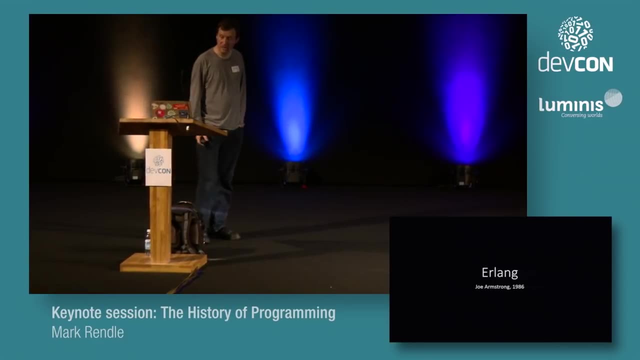 Yeah, no, that's easier. Yeah, well done, dude. You've just made programming accessible to the masses. Idiot Erlang. yes, I know It's the best programming language ever. Yes, I know It's entirely fault. tolerant and brilliant. 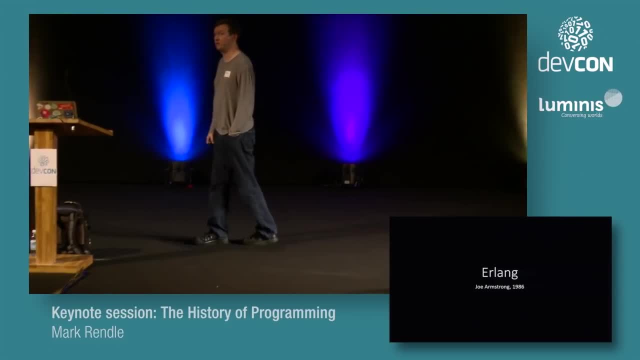 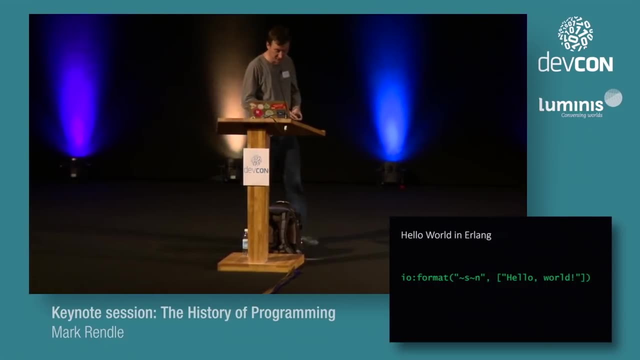 and the best thing ever. and you can even do it in Elixir now, which looks like Ruby. Shut up, It's hello world in Erlang. My battery is running low, which is interesting, considering this is supposed to be plugged in. 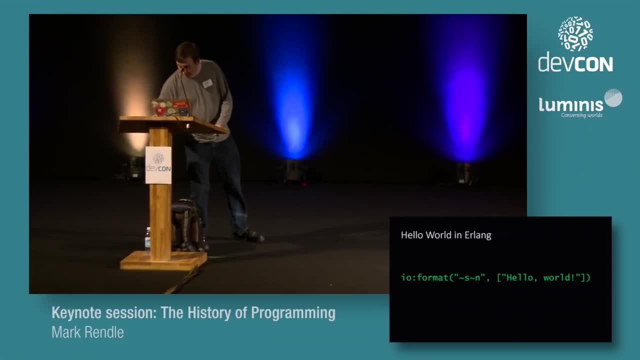 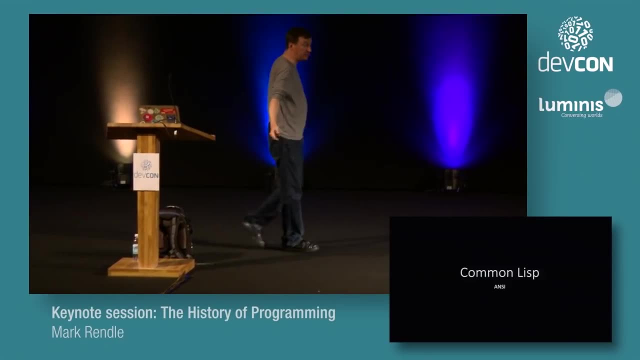 It's not plugged in. Let's just really hope I can make it to the end of the talk. I've got 50 slides to go and five minutes. But yes, Lisp, ANSI created Common Lisp, which had a lot of standard libraries and stuff. 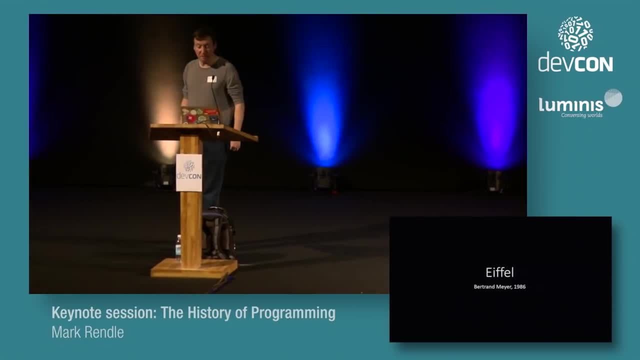 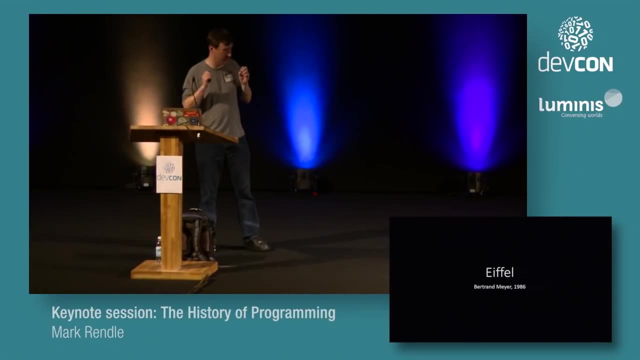 to make Lisp actually usable. Bertrand Meyer came along and created Eiffel, which is contract-based programming, and there's a lot of good stuff about Eiffel, but, dear God, don't go and see Bertrand Meyer talk about it. 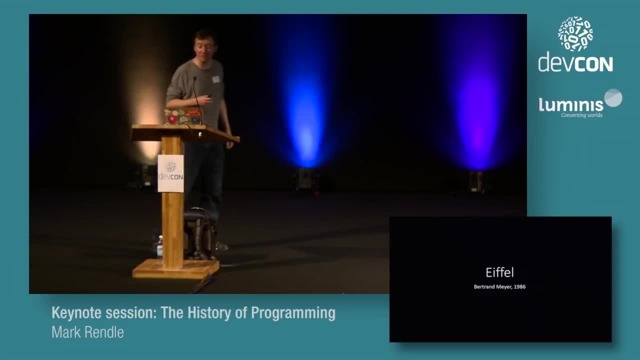 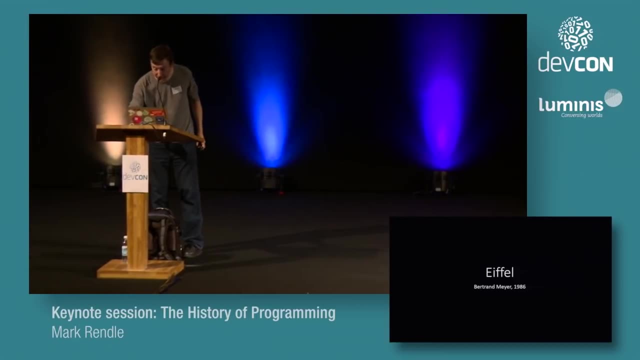 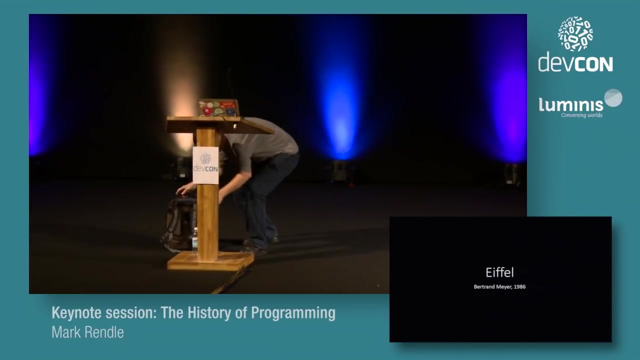 Shit, this is being videoed, Sorry, Hello, Yeah, no, it's 7%. I seriously need some power to this PC. Bad things are going to happen. if this PC does not get power, Why has it not got power? 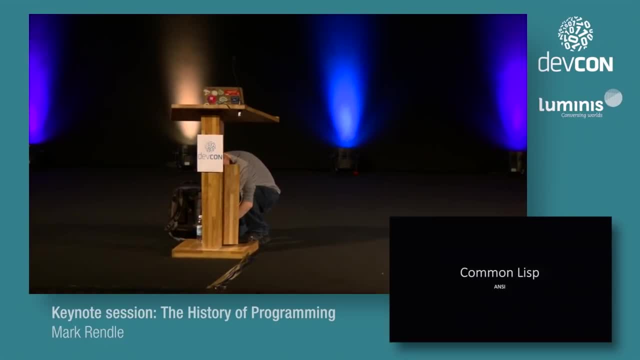 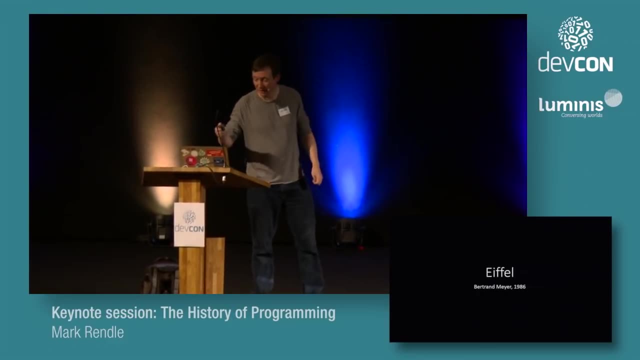 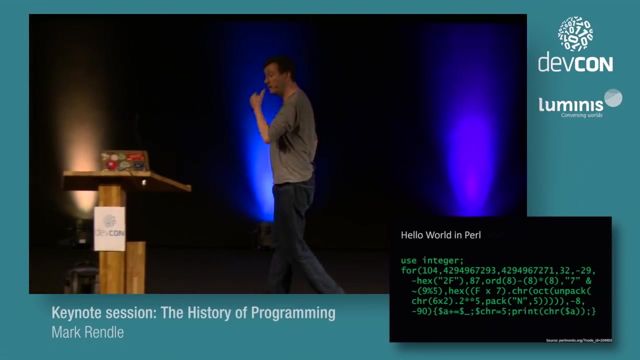 Hardware problems. There we go, That should do it. Yes, right, Yes, Common, Lisp, Eiffel, Larry Wall created Perl After what can only be described as a methamphetamine bender, Which is why Hello World in Perl looks like this: Because real programmers write the code right first time. They don't need to be able to read it. And on that note the 1990s started, And they started brilliantly. We got Haskell. Must be some Haskell people in the room. 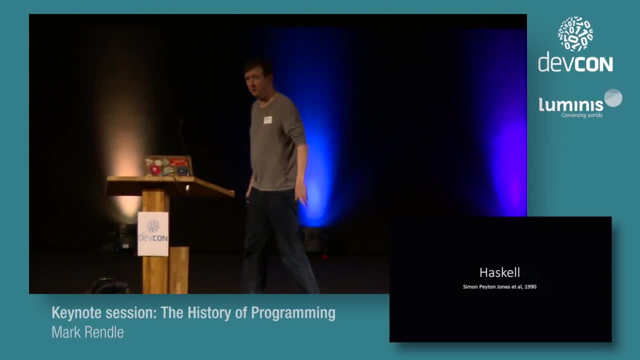 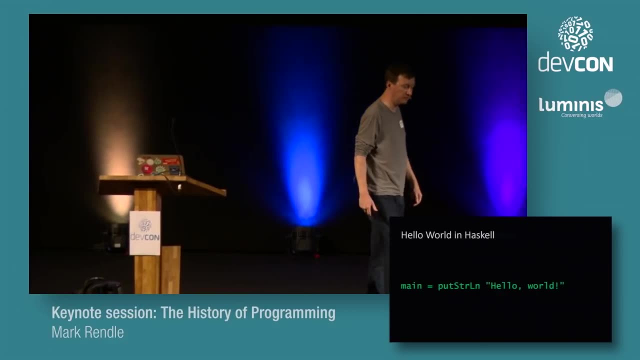 I actually quite like Haskell. It's a very good way of teaching some very useful things that you can then go and use in proper programming languages. But that was created Here's Hello World in Haskell, Not Pascal Haskell, I'm guessing. 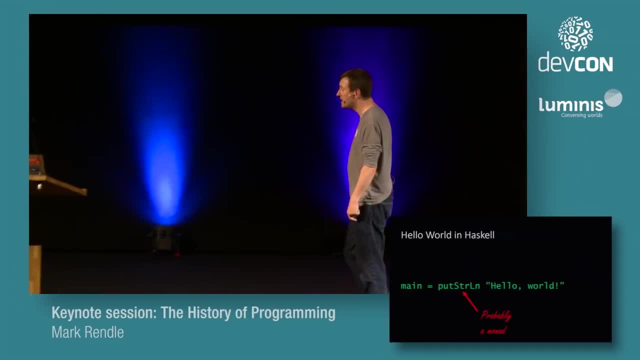 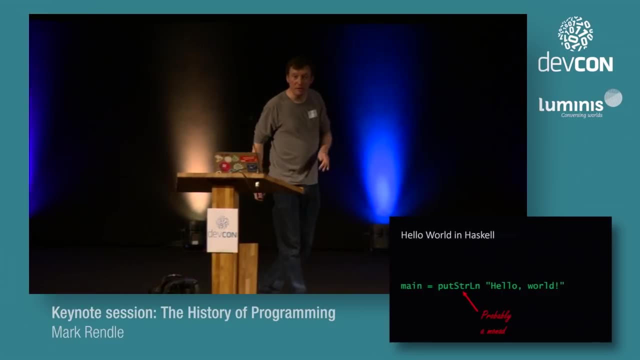 I don't really understand it, But I'm guessing that this is probably a monad. So, yes, Common Lisp was starting to take off, But the EU, in their kind of heyday, were going: hey, We're the EU. 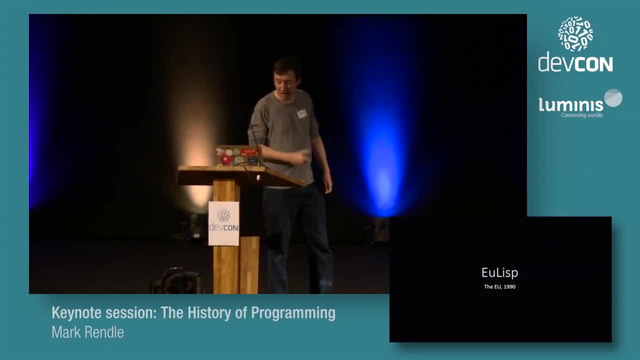 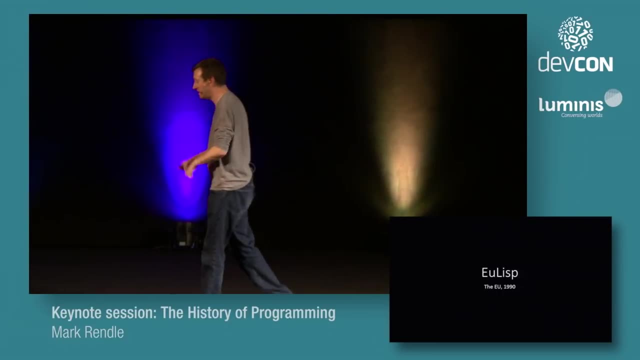 And we define standards of our own and everything, And so we're going to create EU Lisp. So they formed a committee to create EU Lisp And that came out in 1990.. Except it didn't because the EU had formed a committee to do it. 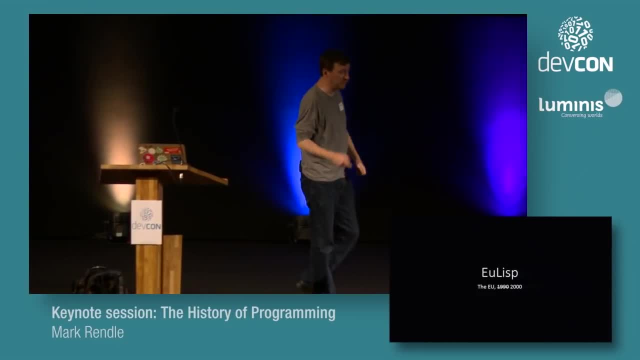 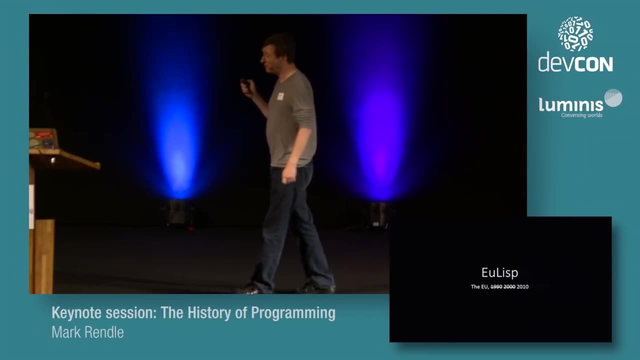 So it actually came out in 2000.. Except it didn't because, let's face it, it is the EU, So it came out in 2010.. Actually, that's not what happened in 2010.. In 2010,, the EU finally admitted they weren't going to do it and just scrapped the project altogether. 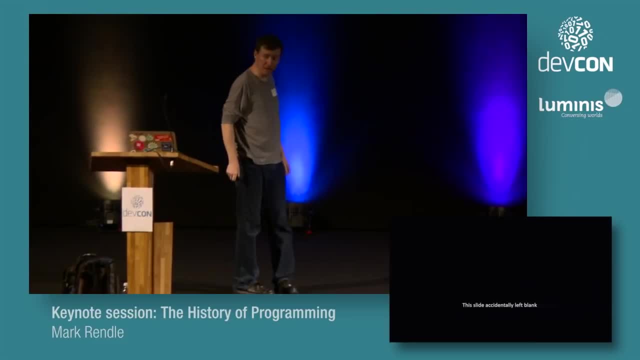 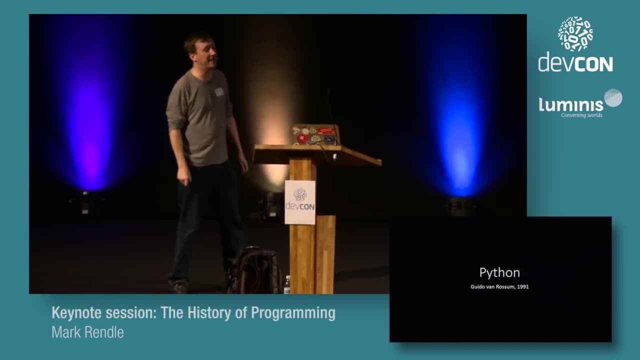 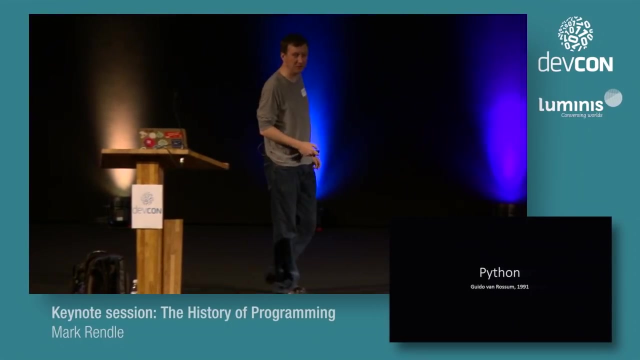 Yes, This slide accidentally left blank. So quick mention of the hometown boy Python. Yes, Python was created in 1991 by one of your guys. Python is fantastic. I love Python. I actually use Python for a whole bunch of stuff. 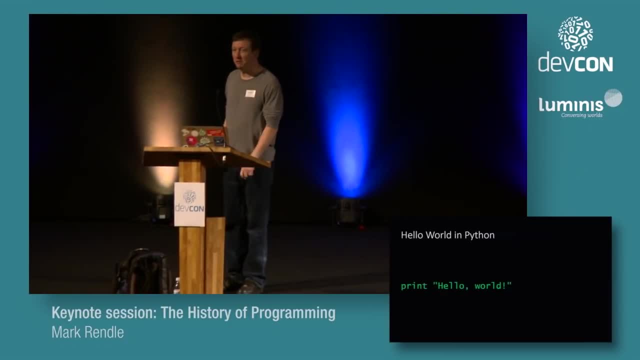 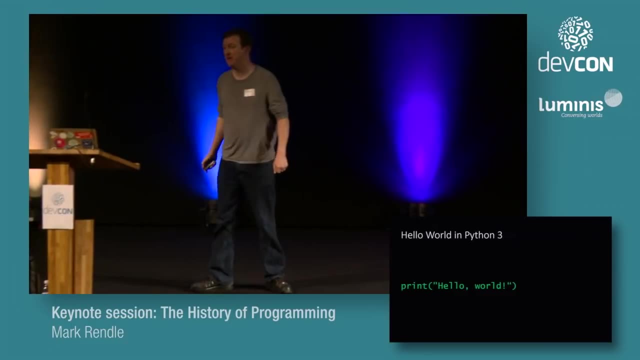 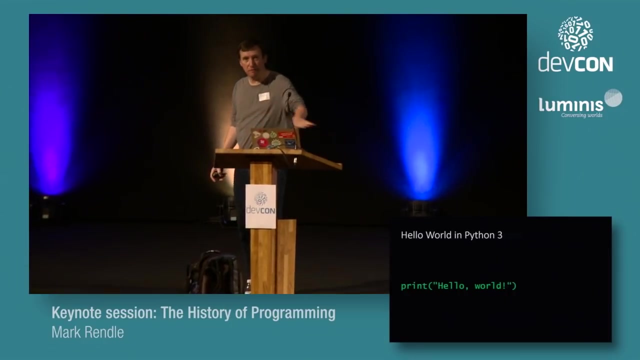 There's only one slight problem with Python. It's hello world in Python. It's hello world in Python 3.. Can we please sort that out, Because it's really starting to piss me off? Apparently, Ubuntu now standardizes. The new Ubuntu that's coming out tomorrow has got Python 3.. 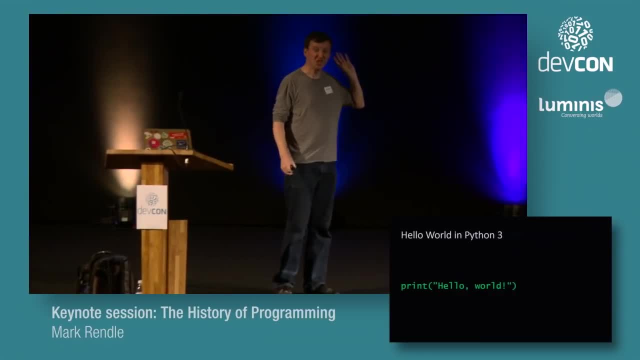 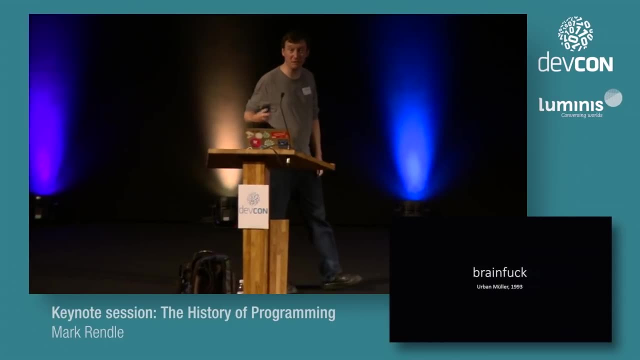 It's now the Python interpreter And Ubuntu have said: just upgrade, Still not ready. Joke programming languages: in the 90s These started to get really good. Brain fuck. Has anyone done? brain fuck, It's hello world in brain fuck. 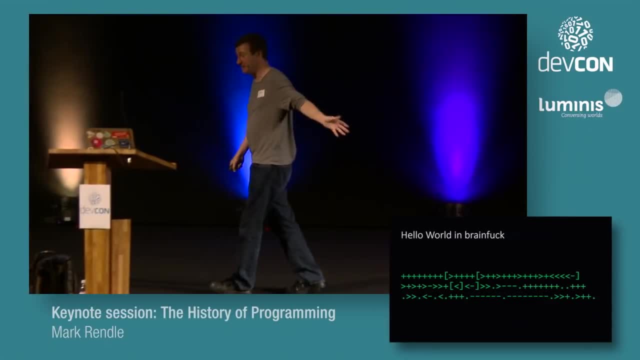 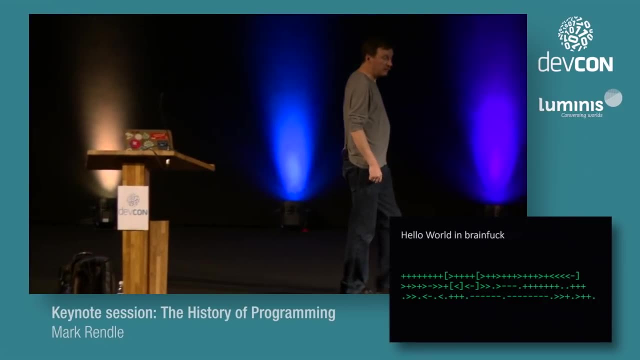 Another great programming exercise: Write a brain, fuck interpreter or compiler. It's very, very easy to do. You'll learn nothing, It's just fun. Someone else came along and went. ah, that's easy. Here's a proper programming language. 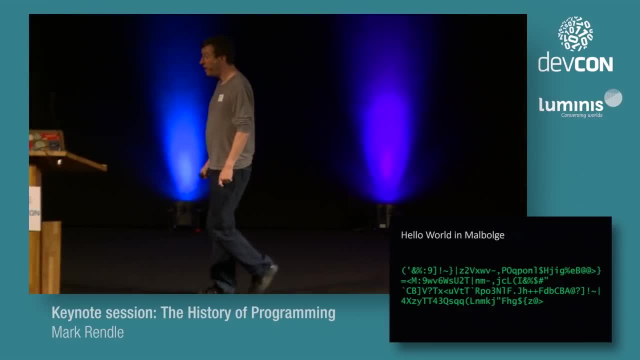 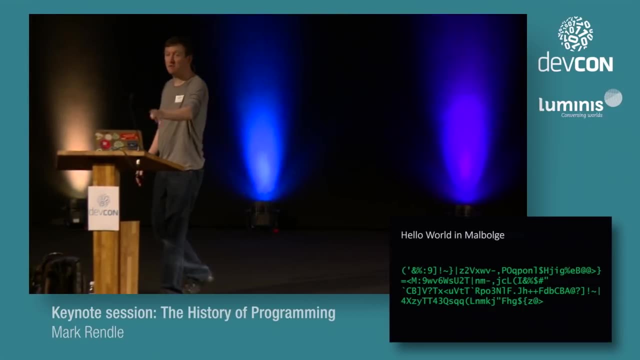 Malbolge. Here is hello world in Malbolge. I swear to you, you can get Malbolge compilers, interpreters, You can copy and paste that It will print hello world. eventually, Malbolge actually encrypts itself as you're going along. 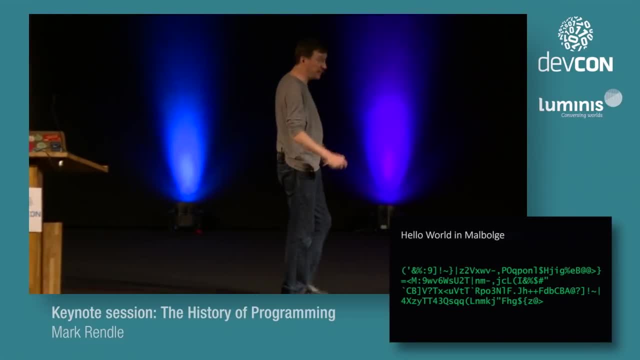 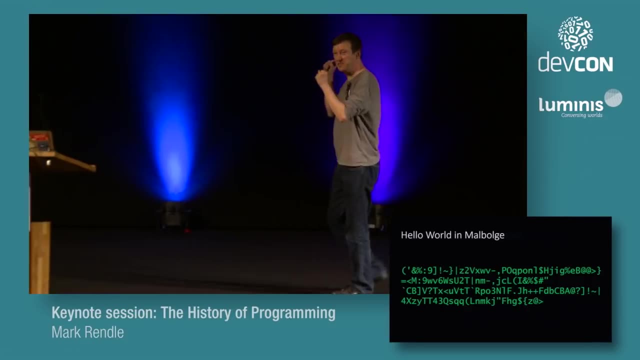 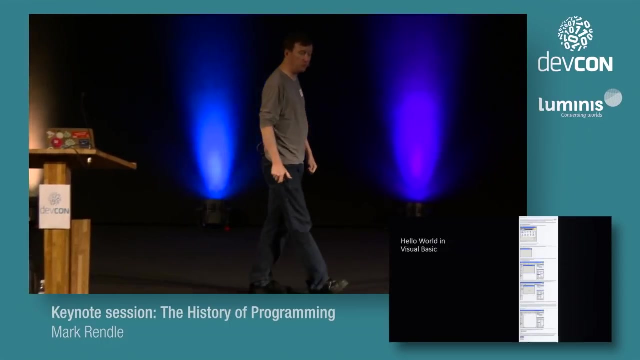 And you have to. But then something came along that just beat all the other obscure, esoteric joke programming languages Into the ground. It was just. nothing could ever top this Visual Basic. So you think I'm joking, but here's hello world in Visual Basic. 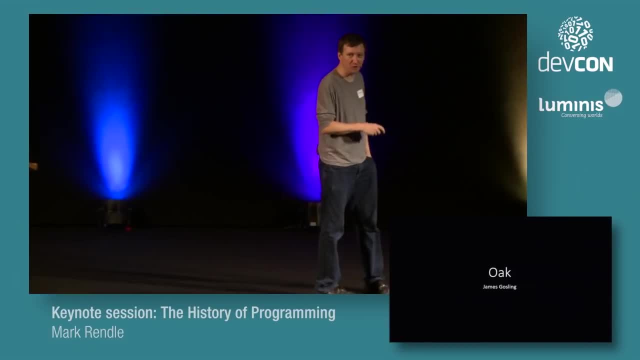 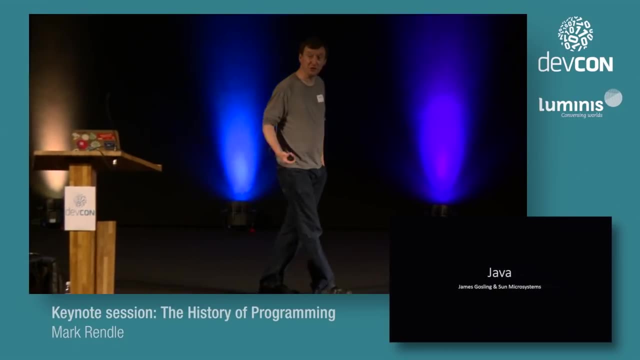 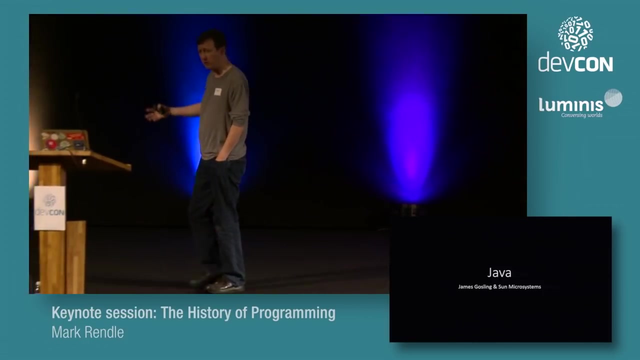 1995, a chap called James Osling created a programming language called Oak, And then he joined forces with Sun Microsystems And they renamed it to Java. Apparently, it was originally called Oak Because there was a tree outside the office where he was working on the programming language. 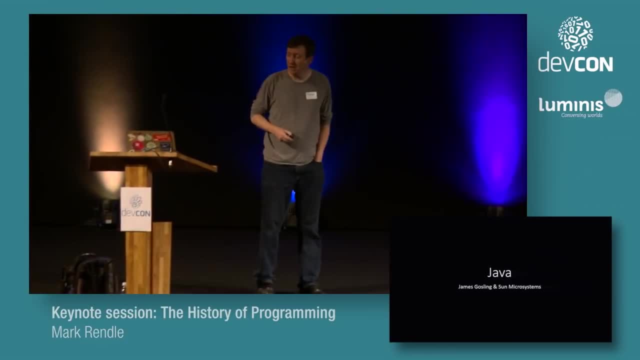 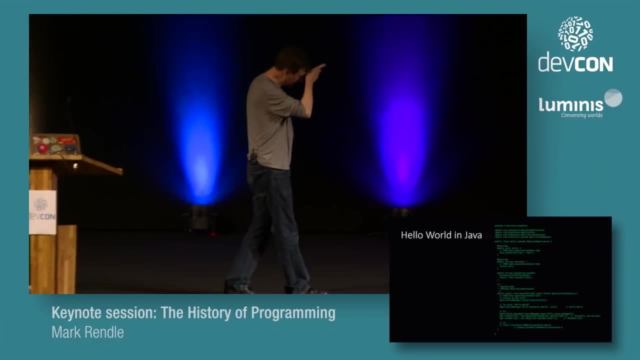 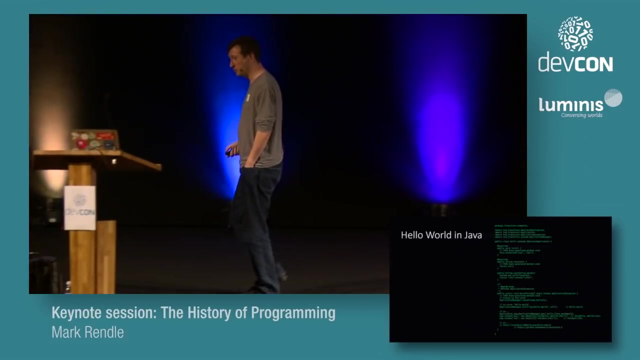 And he couldn't call it two squirrels fucking. So yeah, There's hello world in Java- I'm being mean, That's obviously enterprise Java beans And their great contributions to mankind's continued survival. Around the same time, someone called Rasmus Lerdorf decided that Perl was too complicated. 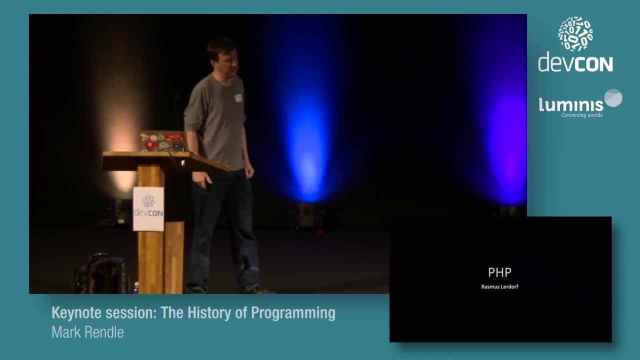 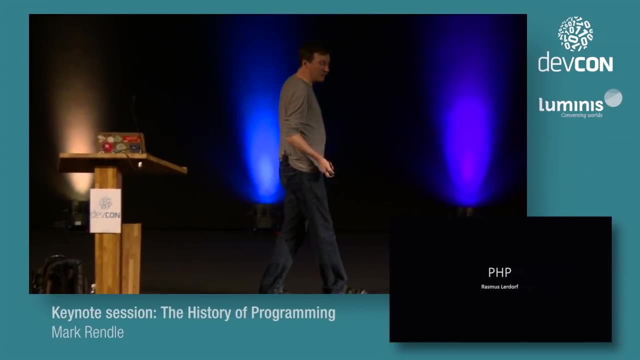 And created PHP to fix the problem. Cheers, Rasmus. Thanks for that Number three on my list of go back in time and kill Over. in Japan, Matsi created Ruby. Ruby is supposed to be a programming language that makes programmers happy. 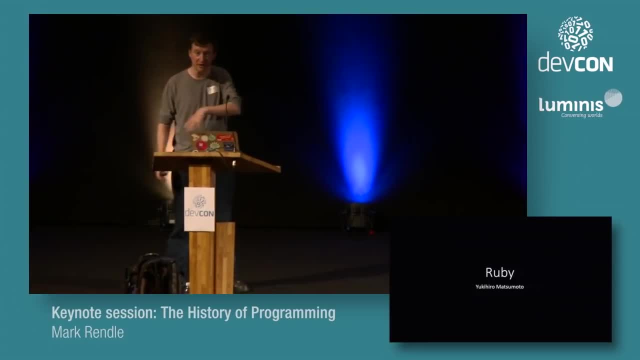 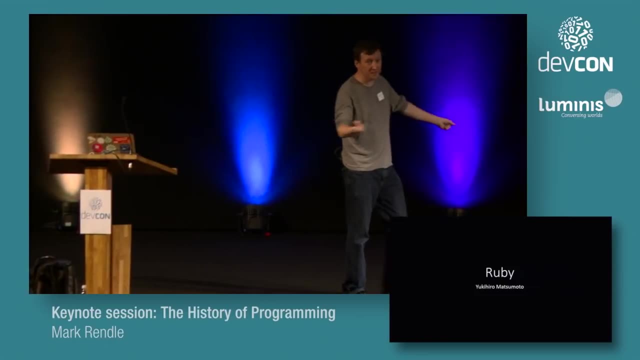 The best reason they seem to be able to give for this is that, instead of saying if something, do something, You can say do something unless something, Which is a terrible way around to have the syntax. It's like walking into this theatre and going: everybody, get out. 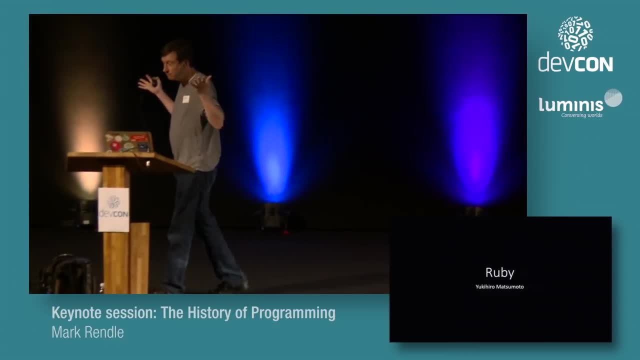 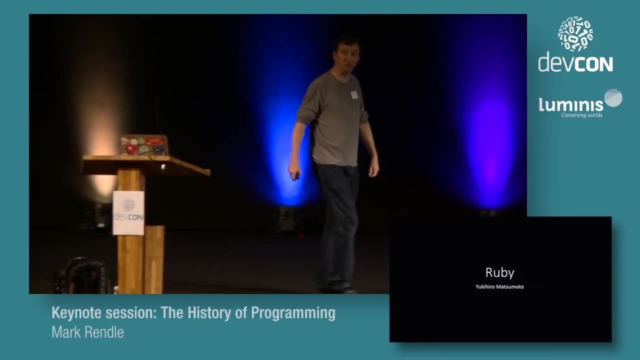 Unless there's not a fire. I'm just saying. Meanwhile, over at Netscape, someone poked their head around the door of Brendan Eich's office And went: can you knock together a scripting language for a demo next week? And Brendan went: yeah, sounds easy enough. 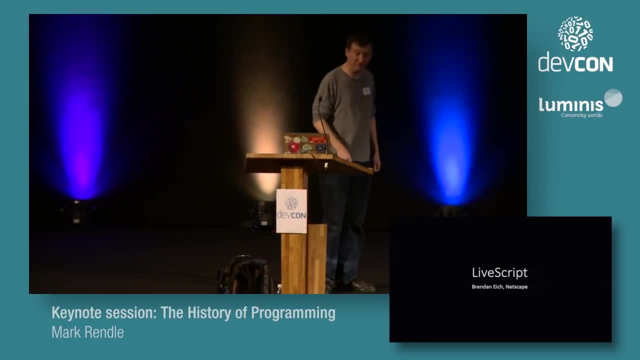 So he created LiveScript And LiveScript. they went well. no, Because LiveScript It's looking a bit like Lisp And we don't like Lisp. Can you make it look like Java? And he went all right. 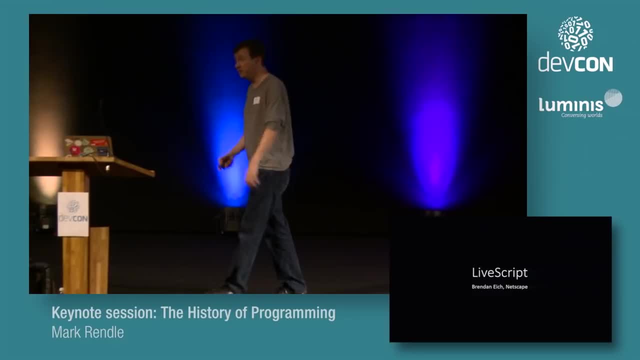 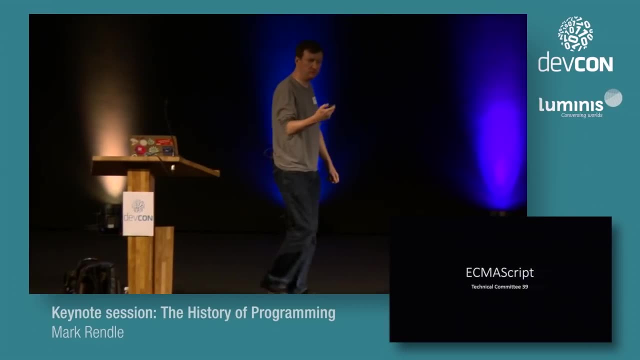 I'll put some curly braces and semicolons in, But underneath it will still be a Lisp. And so he called it JavaScript. And then that got standardised and they called it ECMAScript. And then ECMA got weird about that and just changed it to ECMAScript. 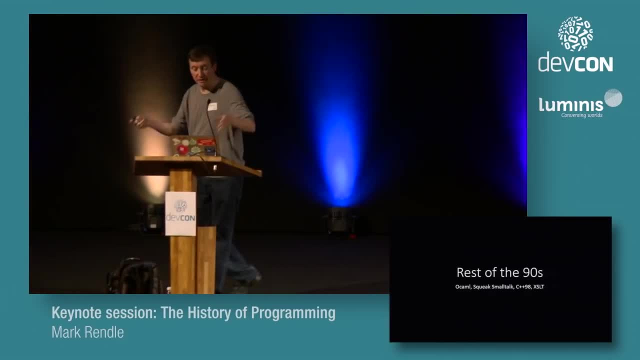 But the CMA are lower case And the rest of the 1990s. we had OCaml, We had Squeak Smalltalk, We had C++98. And we had XSLT. That takes us into the 2000s. 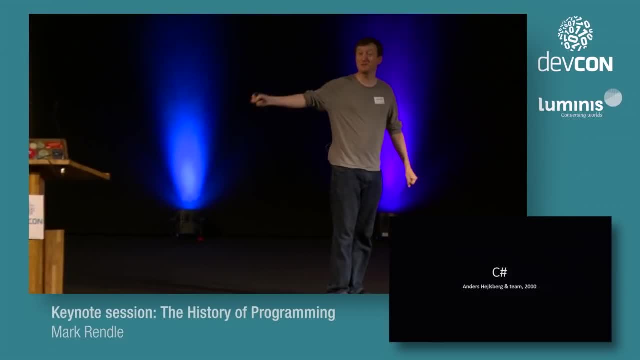 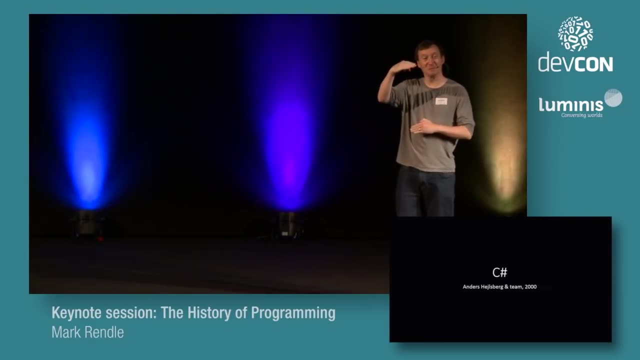 Then we get C Sharp. Does anyone know why C Sharp is called C Sharp? I've run out of time, Can you tell, Talking very fast? C Sharp is called C Sharp because it's C++++ And you take the first plus plus and you put them on top of the second plus plus and it 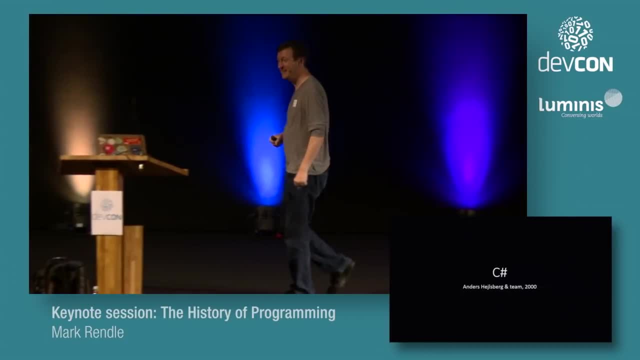 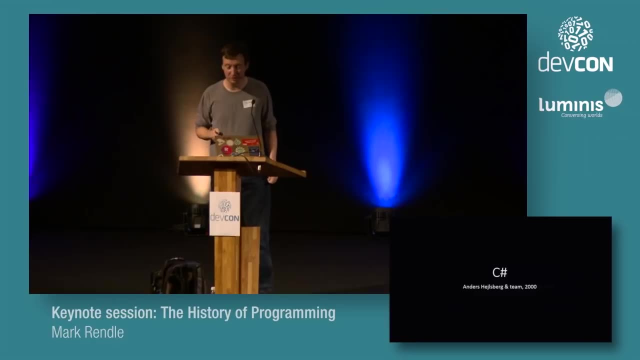 makes a sharp symbol. There you go. Honestly, that's not like a joke. That is actually why it is called C Sharp, Or C Splat, as the Java guys call it. ECMAScript 4 came out, except there was a huge bust up and ECMAScript 4 became ActionScript. 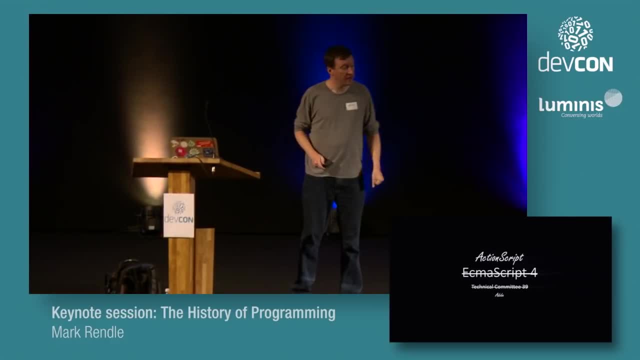 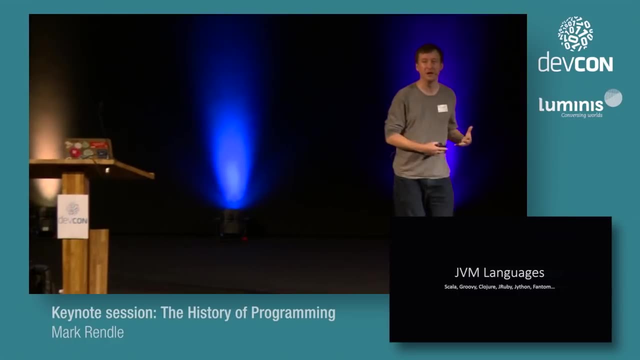 and was only used in Flash and ECMAScript, jumped to 5.. Lots of people started writing programming languages that targeted the JVM, because Java was so shit And it was just not evolving at all. So we got Scala and Groovy, Enclosure and JRuby and various other things. 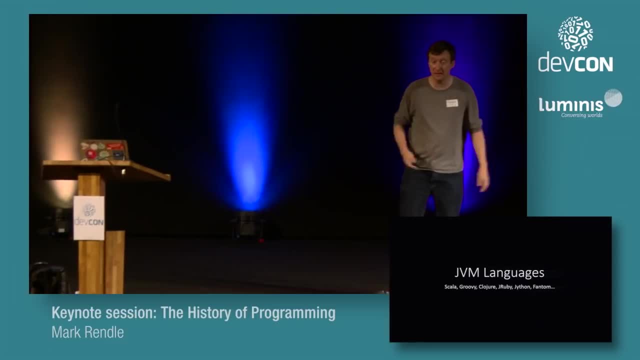 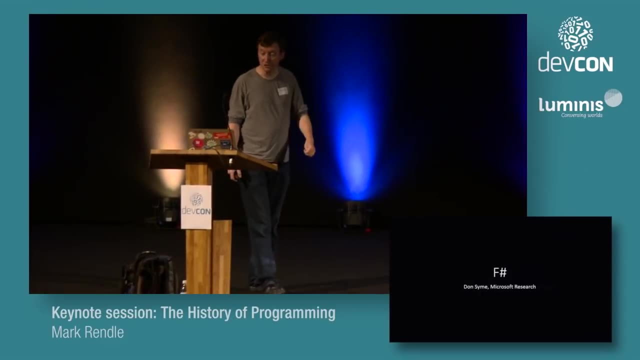 And then Microsoft went: oh, that's a good idea, Let's see if we can get people to target our language. And so we got CLI languages like Boo Namurl, IronPython, IronDiscontinued and so forth, And, of course, F Sharp from Don Simon at Microsoft Research. 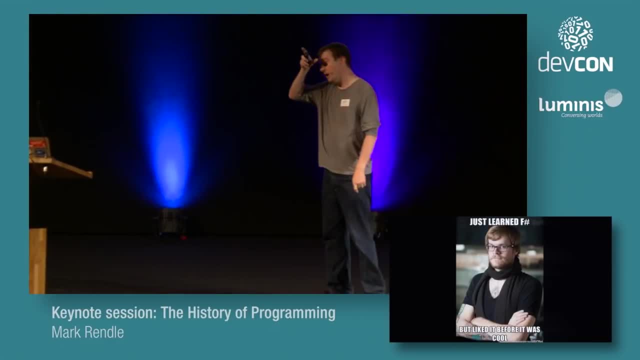 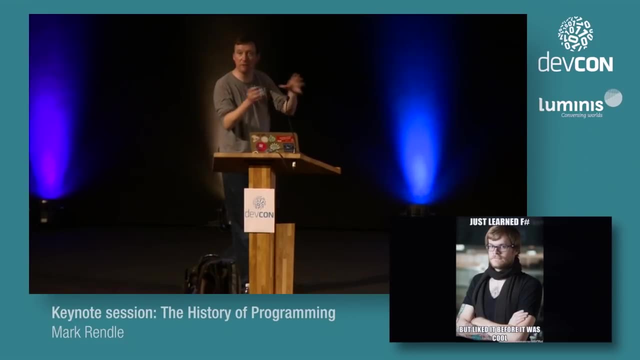 Lots of people like F Sharp. This chap likes F Sharp, So that's great. But you know, since then we've had some great advances in programming languages. in the 2000s We've had Go from Google, which is really rather good. 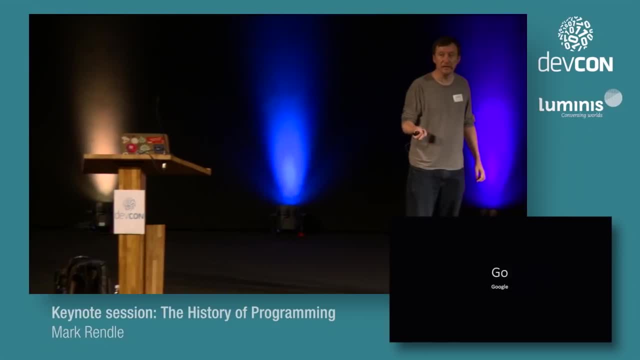 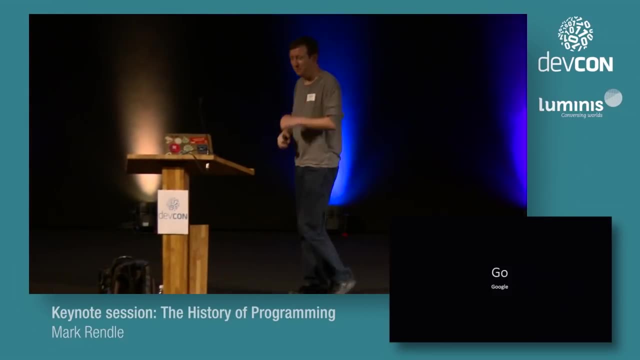 It's got some great ideas in there. I don't like it because of the idea that you're supposed to use eight space tab indents. Yeah, I'm not getting on board with that, But it's a compiled, statically linked garbage. 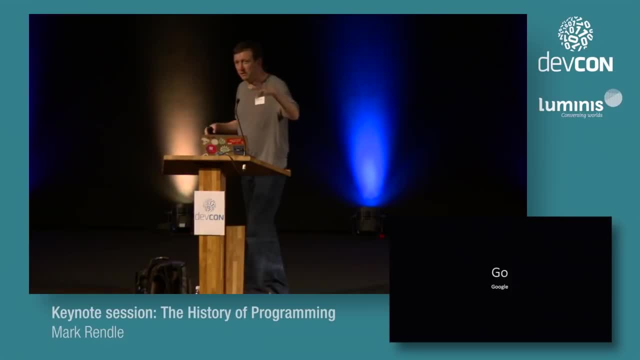 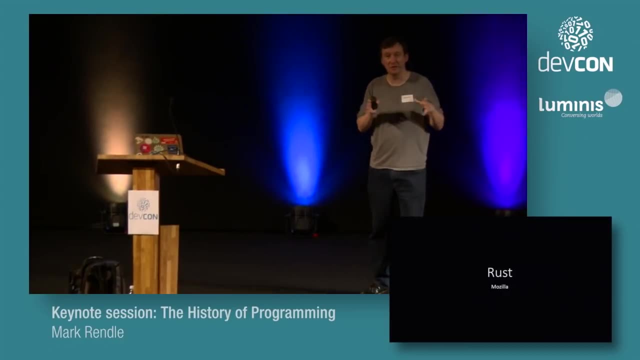 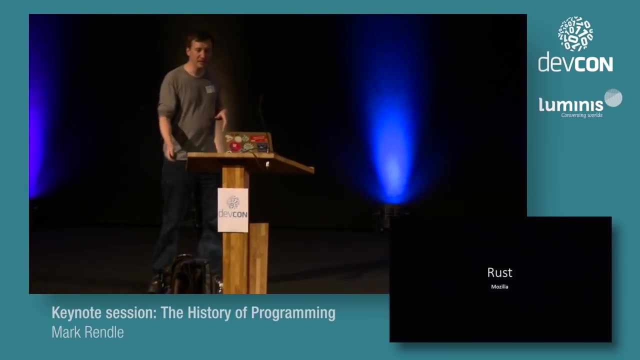 And it's got this defer keyword and go routines, and those are quite cool. We've also got Rust, which has come from Mozilla, which is a programming language specifically designed for writing browser engines, So that's fun. And then the other thing that we've started to get lately- and this is weird- is languages that compile to JavaScript. 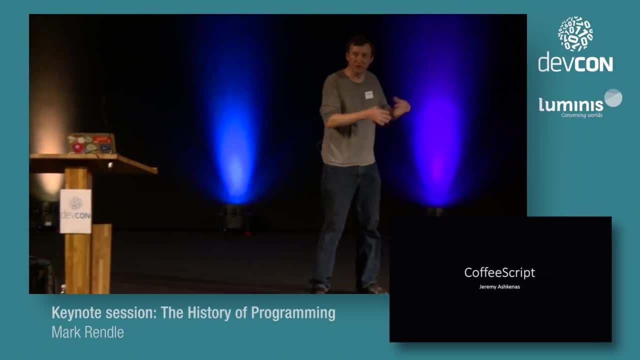 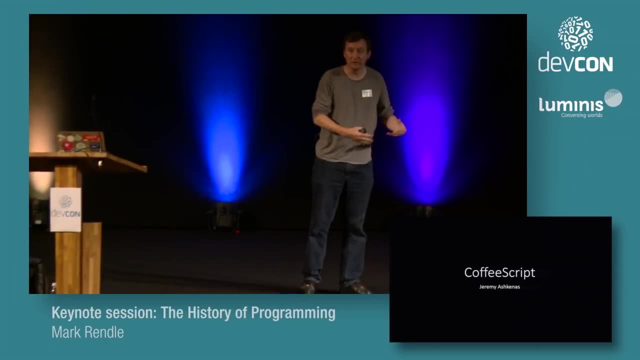 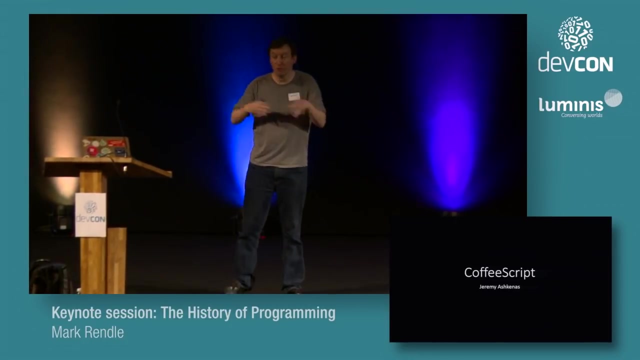 So this started with CoffeeScript, because lots of the people who were trying to write JavaScript were Ruby programmers who can't actually program. They can just write Rails commands on the command line that generate JavaScript. And so this guy created CoffeeScript, which makes JavaScript look more like Ruby, but it compiles to JavaScript. 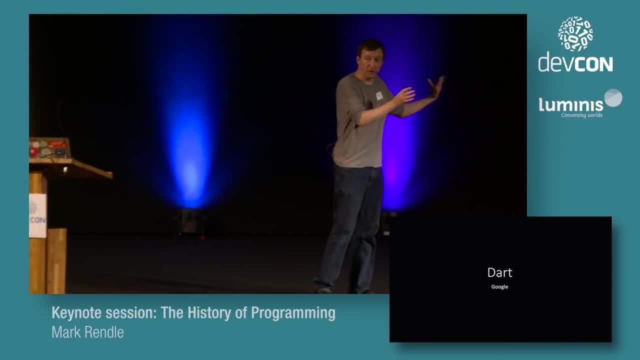 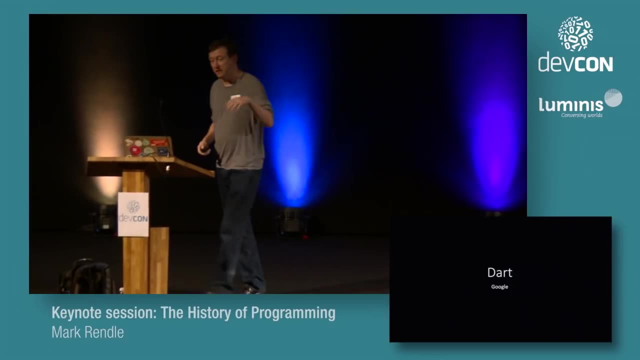 Google created Dart and the idea was that everyone was going to make their browsers support Dart, and everyone turned to Google and went piss off, And so Google went: all right, let's compile Dart to JavaScript. That'll be good, So that works. 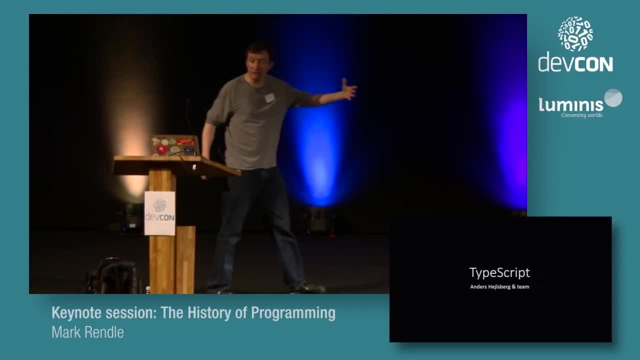 And then Anders Heilsberg, they rewrote the C sharp compiler and they've just finished that and it's called Roslyn And basically they had feature freeze on C sharp while they did it and it took a very long time. 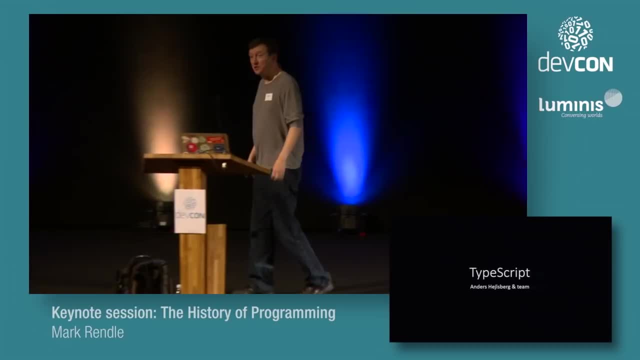 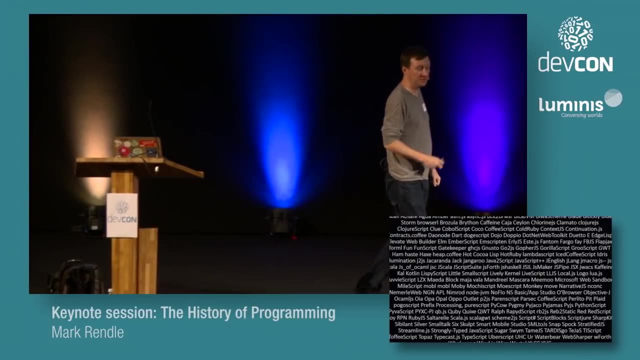 And so Anders got bored and created a typed version of JavaScript. So you know there's languages that Actually, this is not even an exhaustive list. There are a lot of languages that compile to JavaScript. There's also Elm now, which lots of people are getting very excited about Elm. 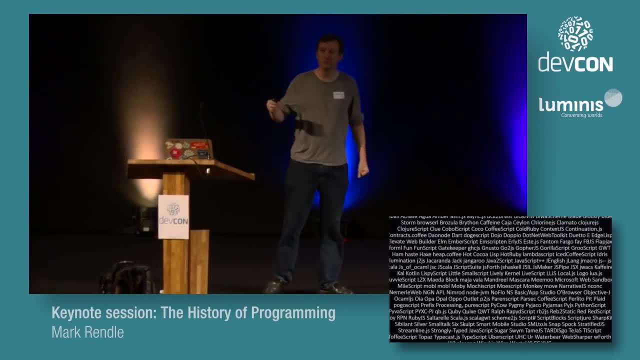 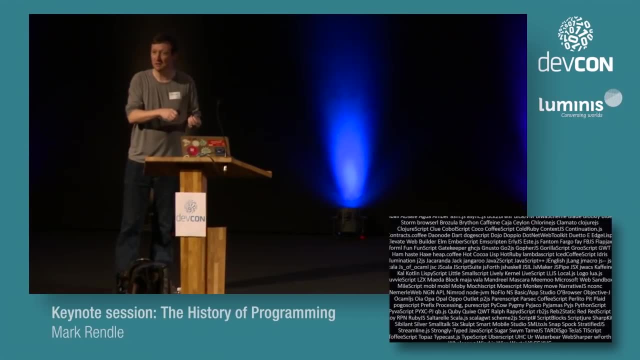 And you know, I'm just thinking Dutch Elm, that's like leprosy for trees, isn't it? Or is this a thing? Do you call it Dutch Elm disease? Yeah, Because I wasn't sure if that was. You know, it's like the.